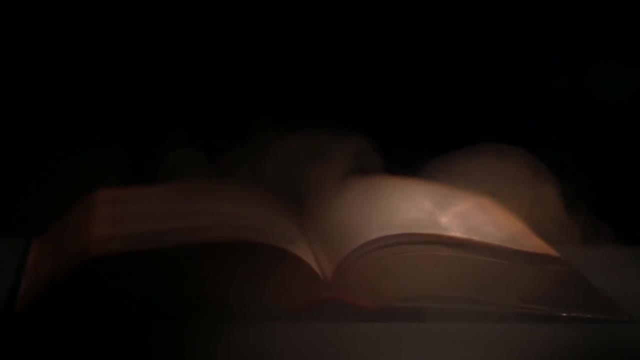 A single sentence in one of the oldest math books held the key to understanding our universe. Euclid's Elements has been published in more editions than any other book except the Bible. It was the go-to math text for over 2,000 years, But for all that time mathematicians were. 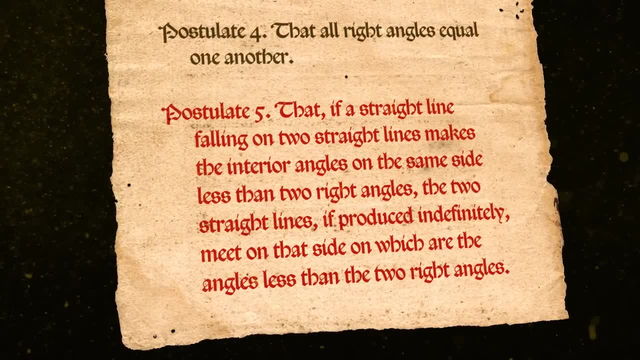 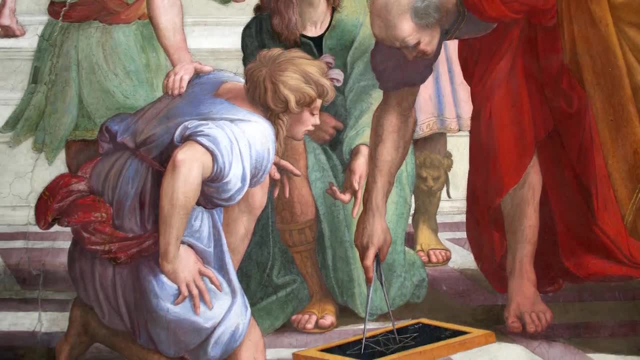 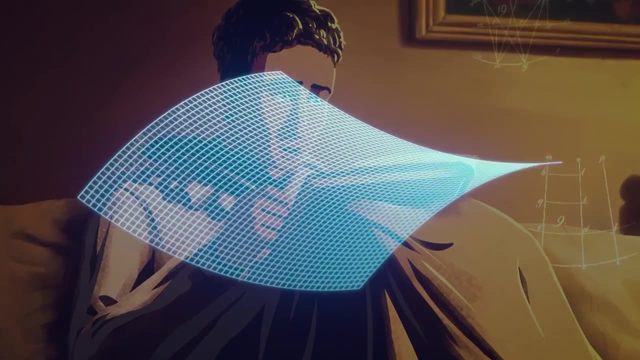 skeptical of a single line which seemed like a mistake. Ultimately, some of the greatest math minds realized that Euclid wasn't wrong after all. But there was more to the story. Slight tweaks to this line opened up strange new universes out of nothing. Surprisingly. 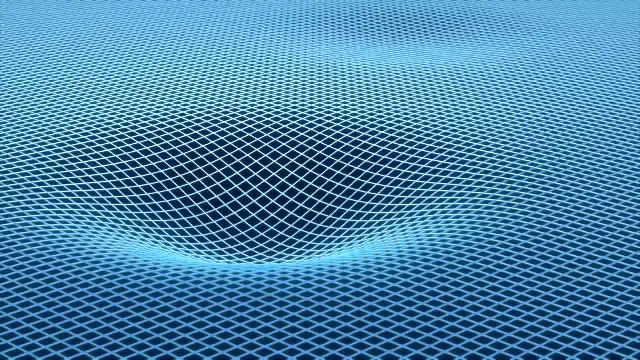 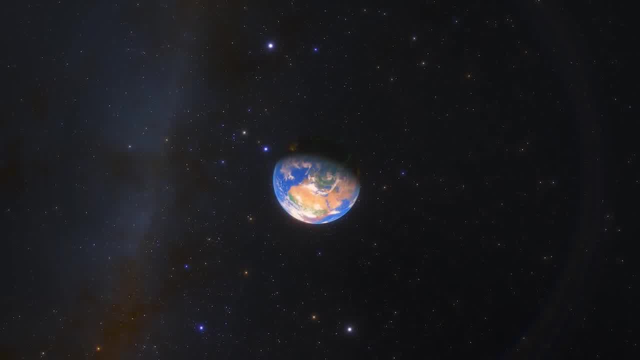 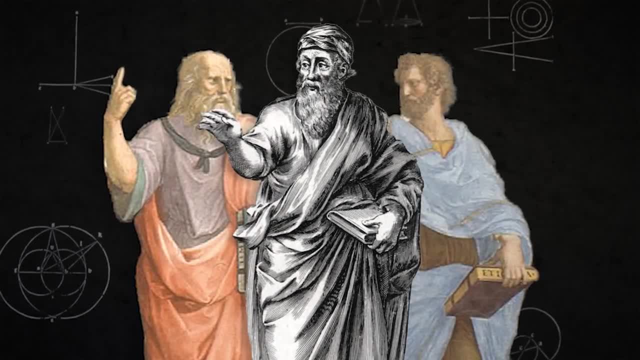 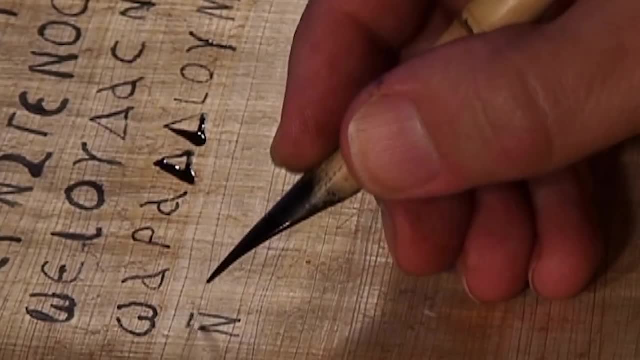 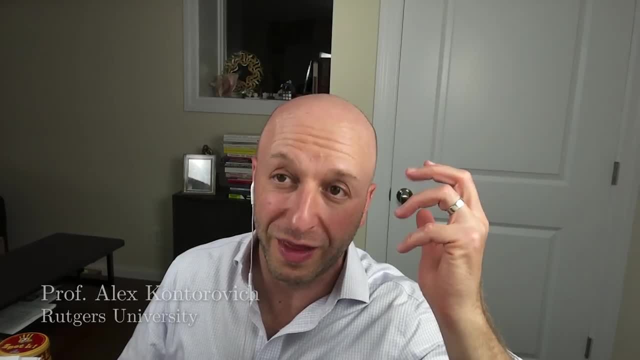 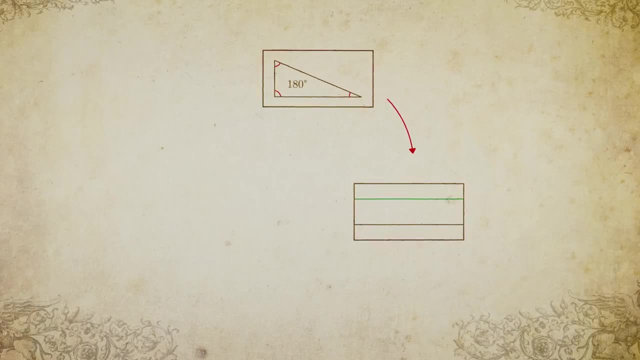 there was a bit of a problem with math. People would prove things, but they would just be going around in circles. Why does a triangle have 180 degrees? Because if you take two parallel lines, yeah, but why do parallel lines exist? 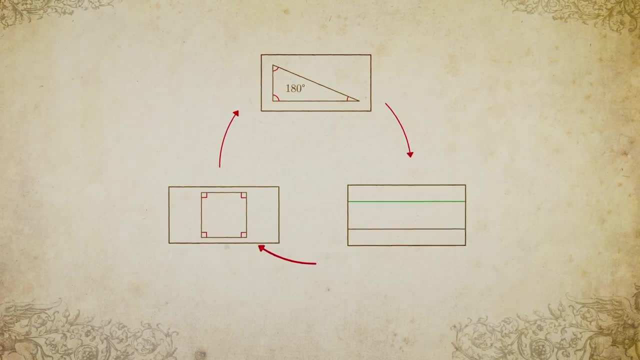 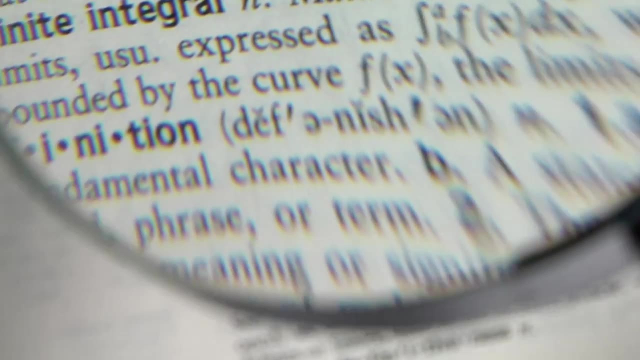 Oh, that's because you can make a square. Why does a square exist? You have this infinite recursion of what the fundamental reason why something is true is. It's kind of like in the dictionary: Every word is defined in terms of other words. 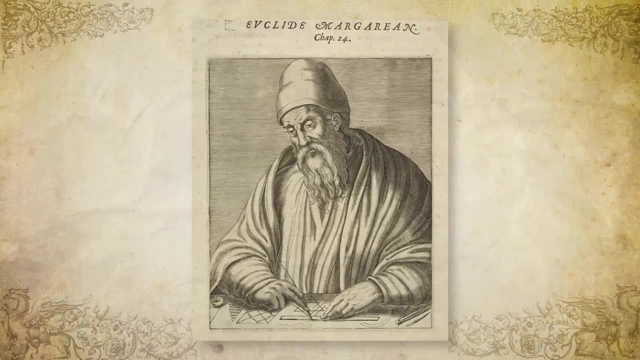 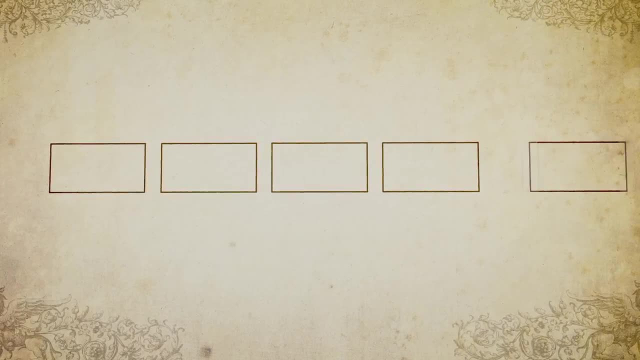 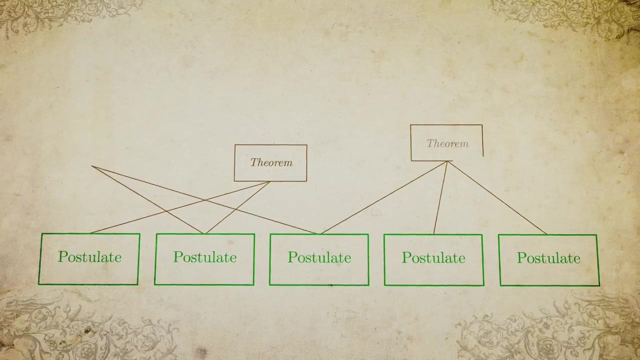 So how do you get to ground truth? Euclid used a solution that was pioneered by the Greeks. Let's just accept a few of the most simple basic things as being true. These are our postulates. Then, based upon these postulates, we can prove theorems, one at a time, building up our math using logic. 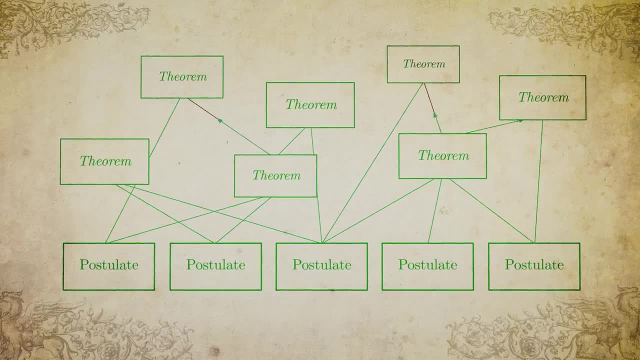 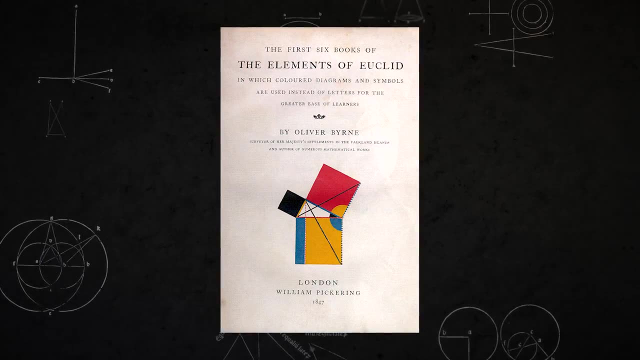 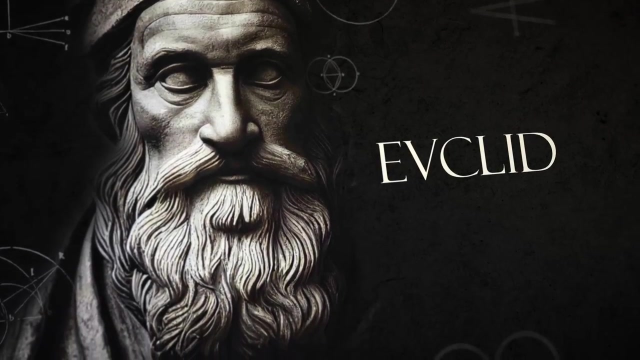 So that as long as those first statements are true, then everything else that follows from them must definitely be true. He had perfected the gold standard for rigorous mathematical proof that all modern math relies on. Okay, Euclid used this method when he published his 13-book series called The Elements. 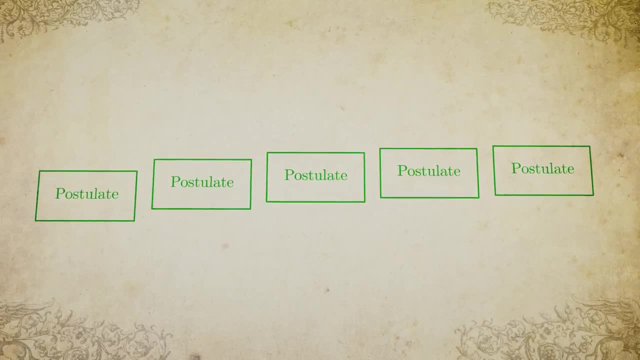 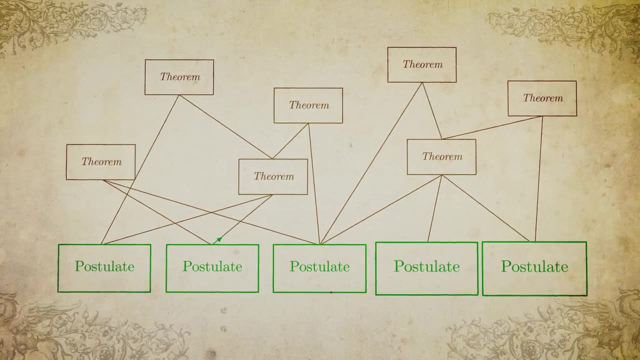 These are our postulates. Then, based upon these postulates, we can prove theorems, one at a time, building up our math using logic, So that as long as those first statements are true, then everything else that follows from them must definitely be true. 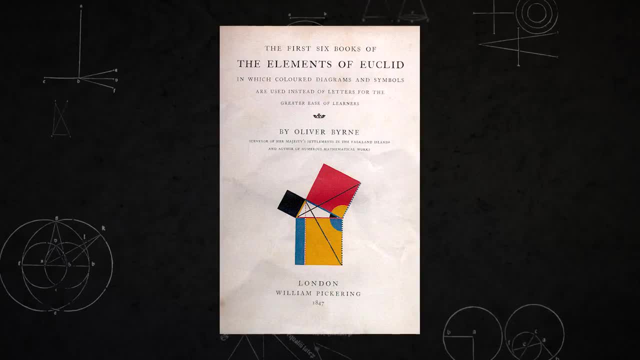 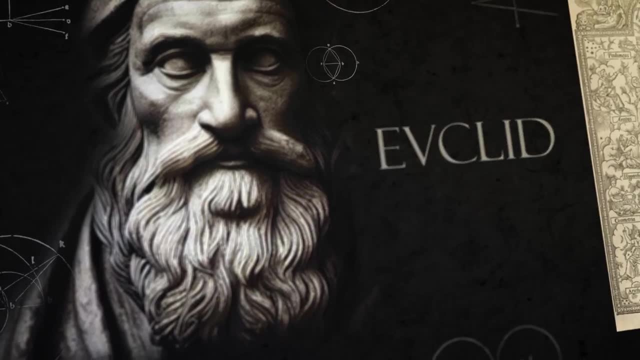 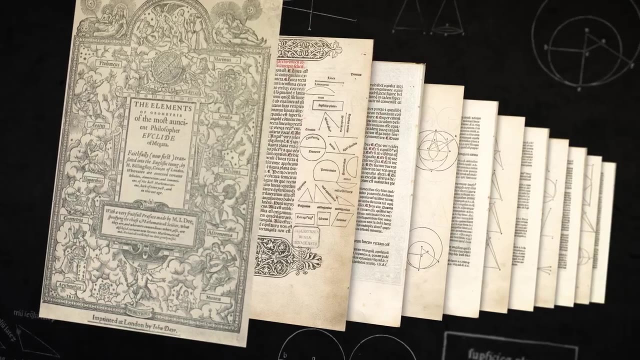 He had perfected the gold standard for rigorous mathematical proof that all modern math relies on. Euclid used this method when he published his 13-book series called The Elements, in which he proved 465 theorems covering almost all of mathematics known at the time. 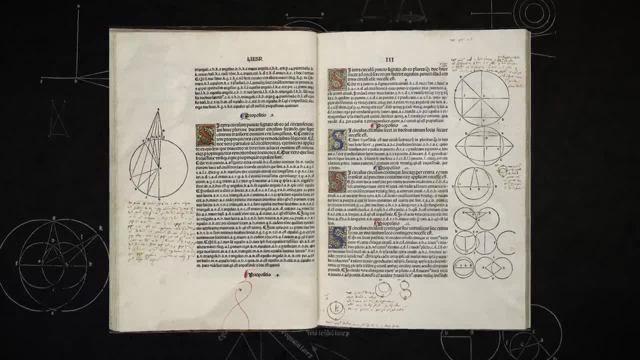 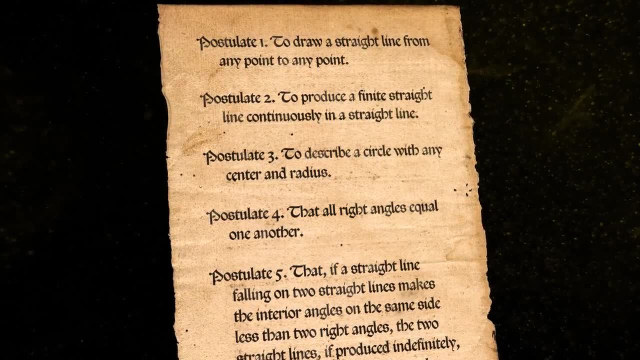 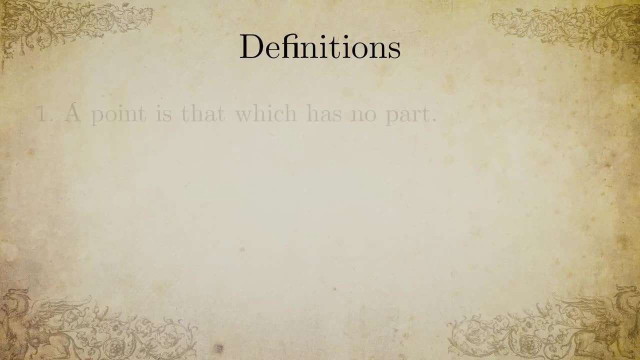 including geometry and number theory, And all these theorems depended on were some definitions, a few common notions and five postulates. We go right to book one, And book one starts with definitions. You gotta start somewhere, And the definition is a point is that which has no part, a line is a breathless 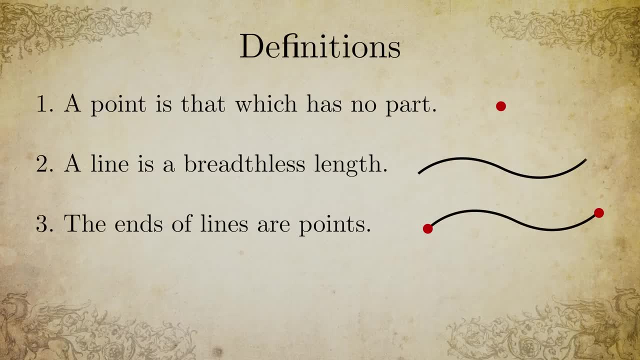 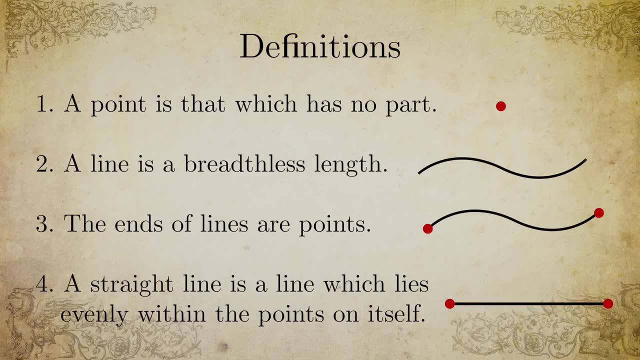 length and the ends of lines are points By line. he really means a curve, and then it has some ends. A straight line is a line that lies evenly within the points on itself, and then so on and so forth. He's got 23 definitions. Then he's got the five postulates. 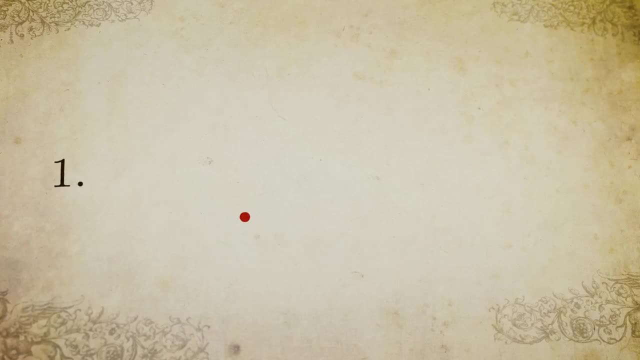 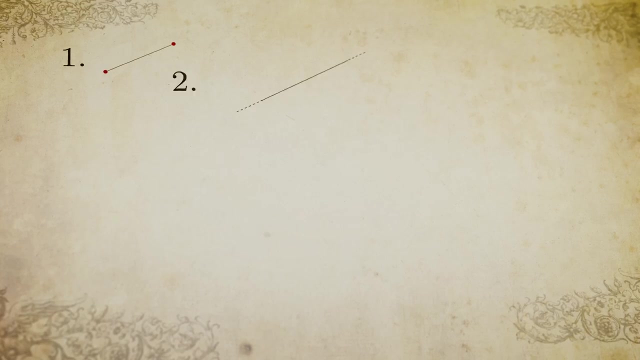 The first four are simple. One: if you have two points, you can draw a straight line between them. Two: if you have a straight line, you can extend it indefinitely. Three: given a center and a radius, you can draw a circle. 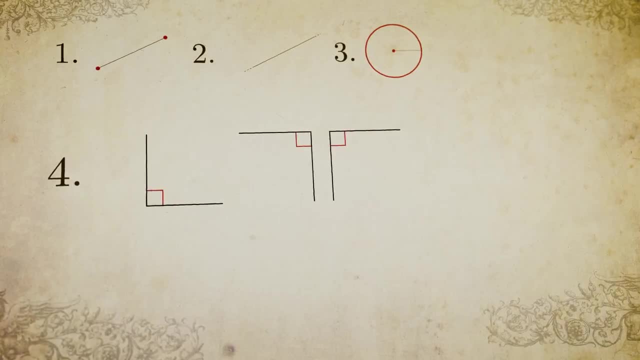 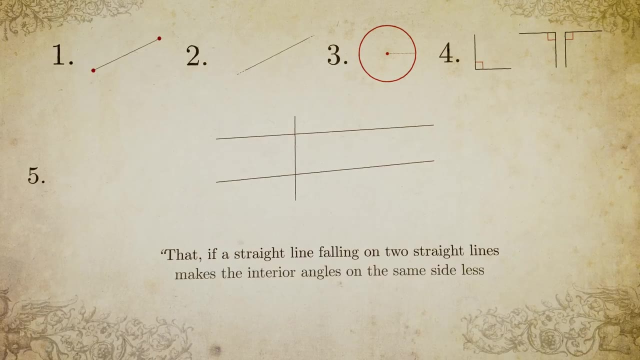 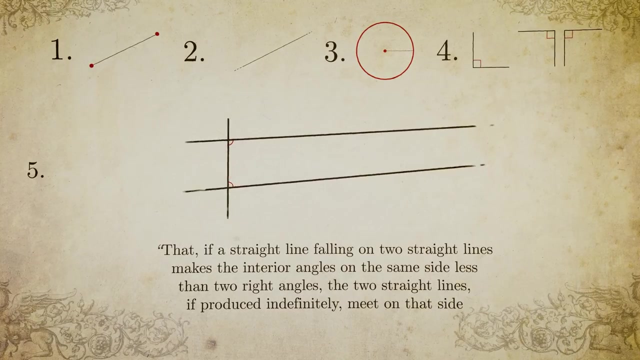 And the fourth is that all right angles are equal to each other. But postulate five gets the big guns, Which is that if a straight line falling on two straight lines makes the interior angles on the same side less than two right angles, the two straight lines, if produced indefinitely. 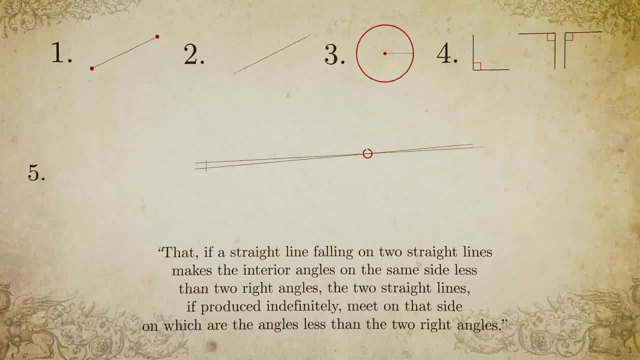 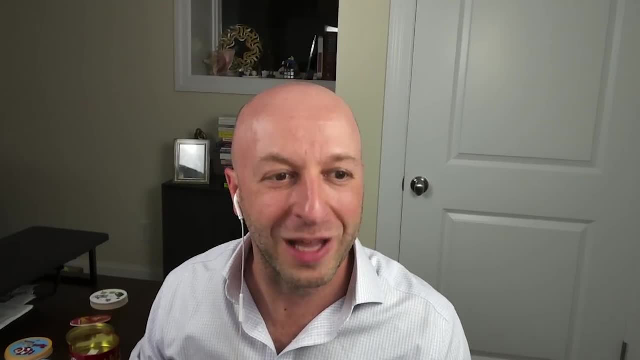 meet on that side, on which are the angles less than the two right angles? What the hell is he talking about? That's a postulate, Like all of these are, you know, half of a sentence, and they're all blatantly obvious. 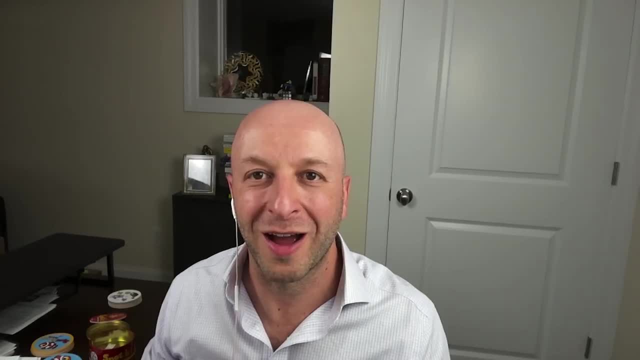 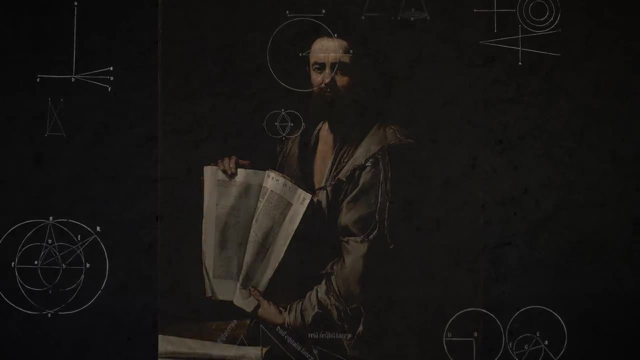 And then comes five out of left field And it's like an entire paragraph. What is he doing? This made mathematicians suspicious. It seemed like Euclid made them in. It seemed like Euclid made them in a mistake. Greek philosopher Proclus thought postulate 5 ought even to be struck out of the postulates. 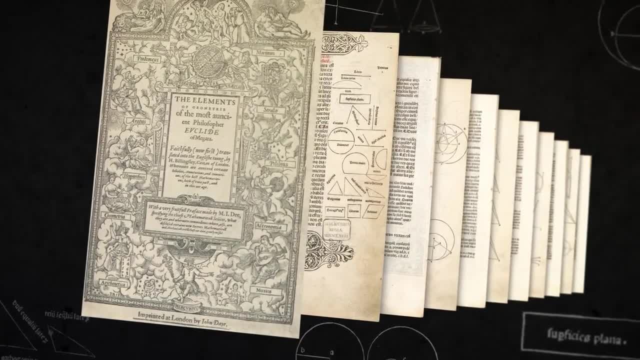 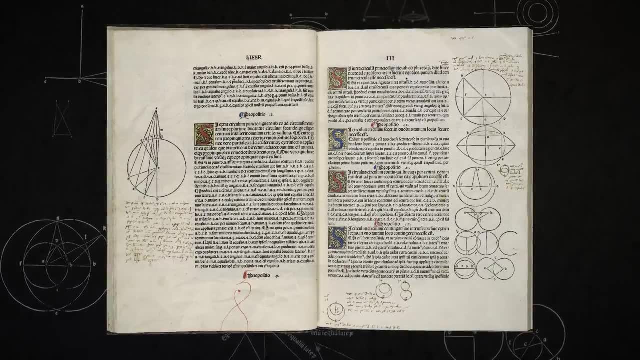 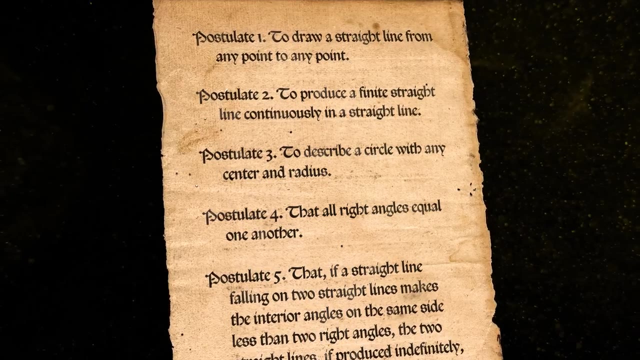 in which he proved 465 theorems covering almost all of mathematics known at the time, including geometry and number theory. And all these theorems depended on were some definitions, a few common notions and five postulates. We go right to book one, and book one starts with definitions. 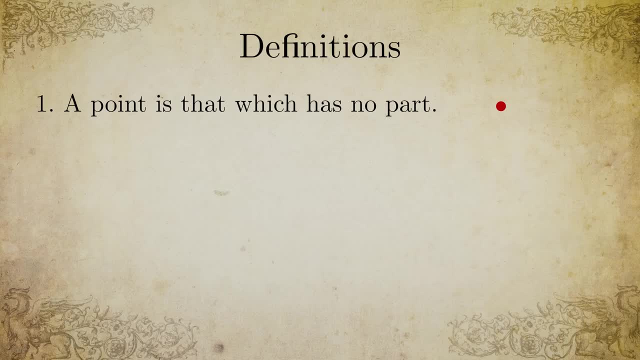 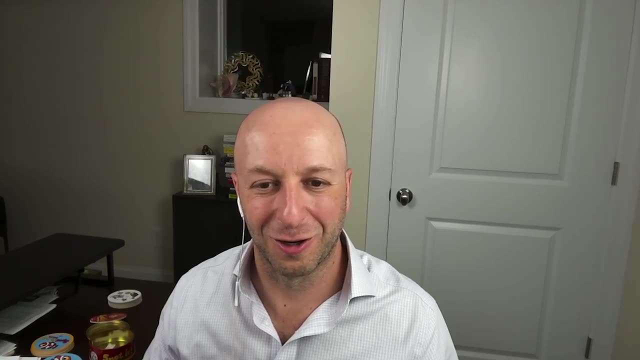 You got to start somewhere, And the definition is a point is that which has no part. A line is a breathless length and the ends of lines are points By line. he really means a curve, and then it has some ends. 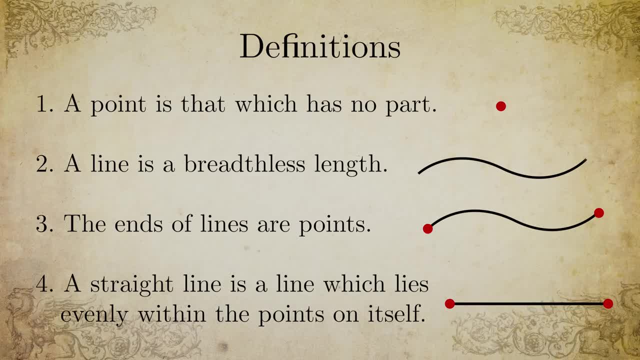 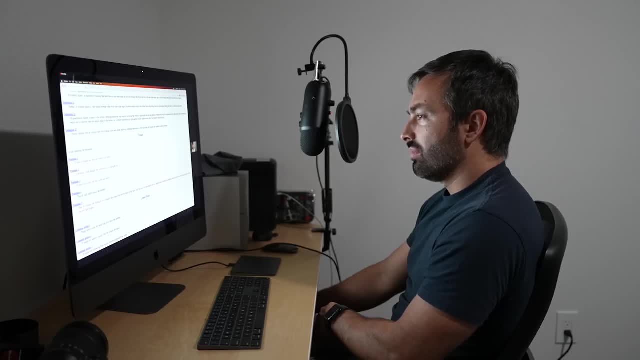 A straight line is a line that lies evenly within the points on itself, and then so on and so forth. He's got 23 definitions. Then he's got the five postulates. The first four are simple One: if you have two points, you can draw a straight line between them. 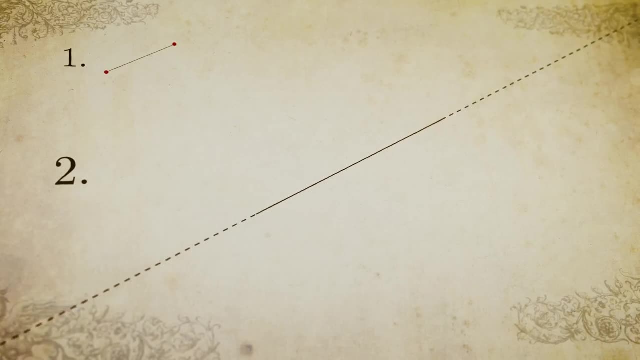 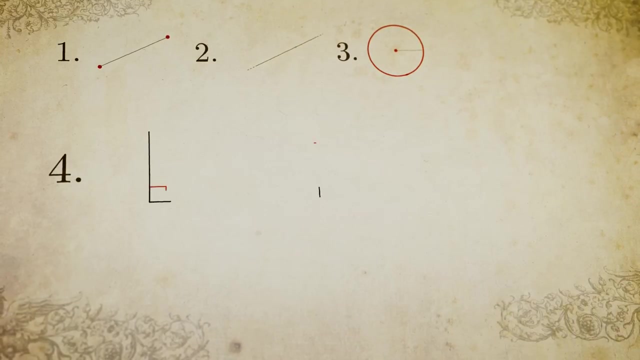 Two, if you have a straight line, you can extend it indefinitely. Three: given a center and a radius, you can draw a circle. And the fourth is that all right angles are equal to each other. But postulate five gets the big guns. 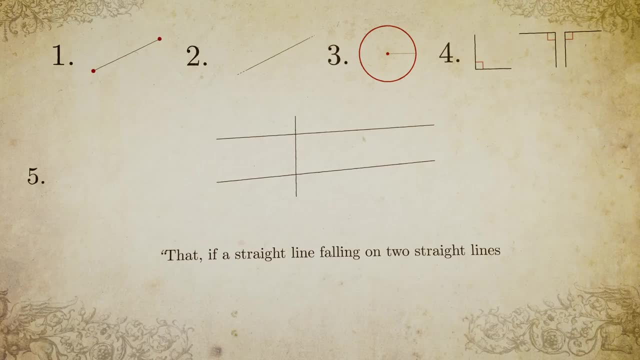 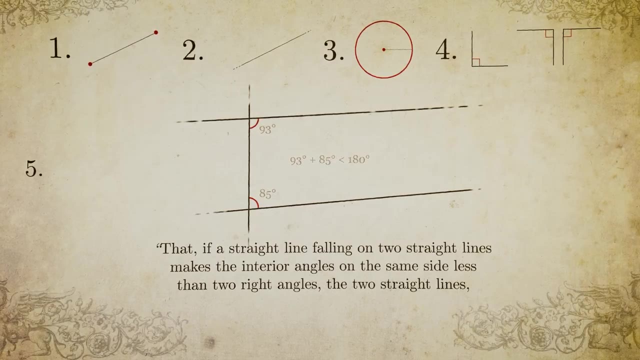 Which is that if a straight line falling on two straight lines makes the interior angles on the same side less than two right angles, the two straight lines, if produced indefinitely, meet on that side on which are the angles less than the two right angles. 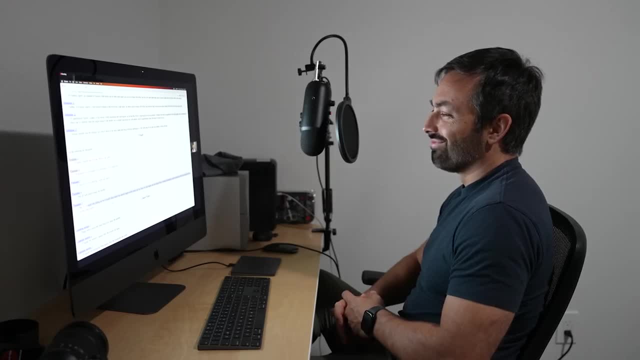 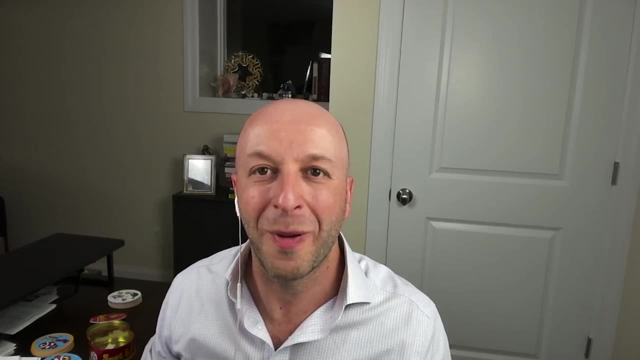 What the hell is he talking about? I don't know. That's a postulate, Like all of these are. you know half of a sentence and they're all blatantly obvious, And then comes five out of left field and it's like an entire paragraph. 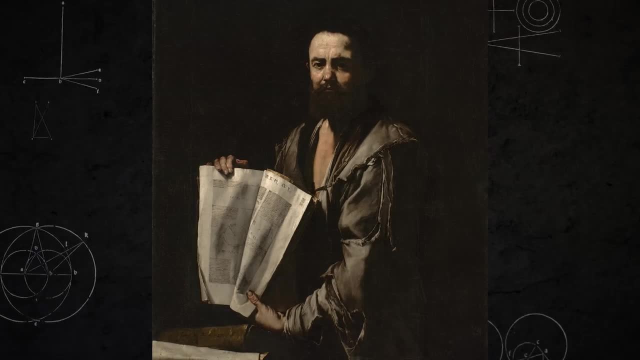 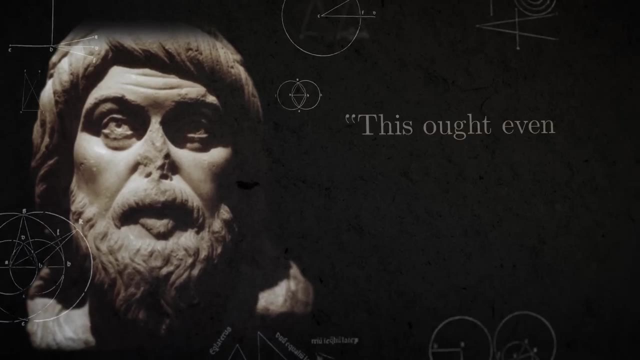 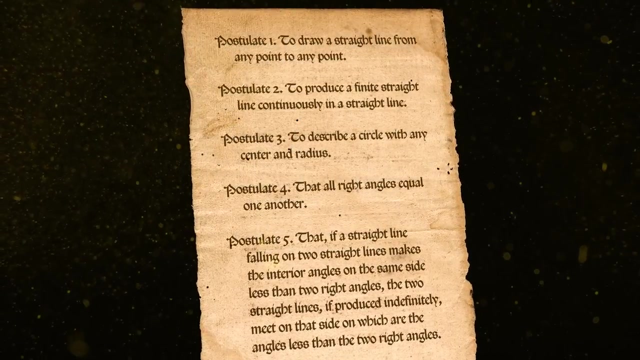 What is he doing? This made mathematicians suspicious. It seemed like Euclid made a mistake. Greek philosopher Proclus thought postulate five ought even to be struck out of the postulates altogether, for it is a theorem. But if it's a theorem we should be able to prove it from the first four postulates. 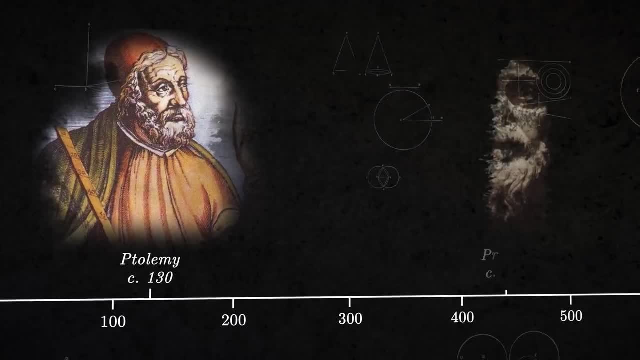 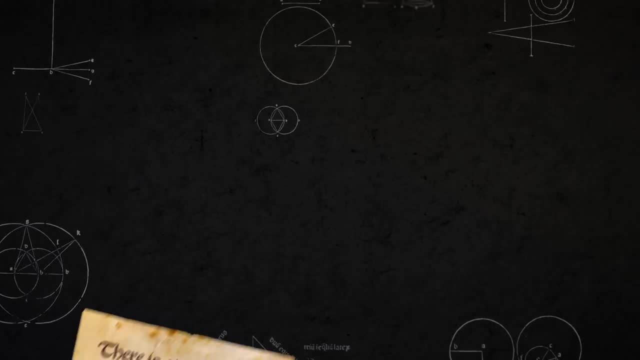 So that's what many people try. Some, including Ptolemy and Proclus, believed they had succeeded, But they hadn't In fact. all they managed to do was just restate postulate five in different words. Here's one formulation: 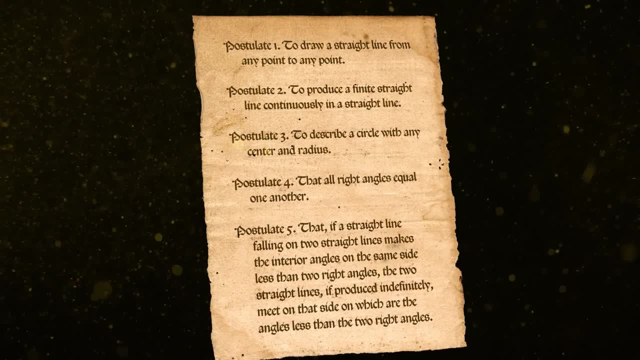 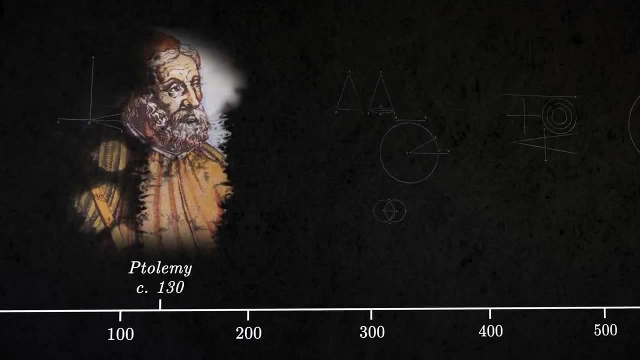 altogether, for it is a theorem. But if it's a theorem we should be able to prove it from the first four postulates. so that's what many people tried. Some, including Ptolemy and Proclus, believed they had succeeded. 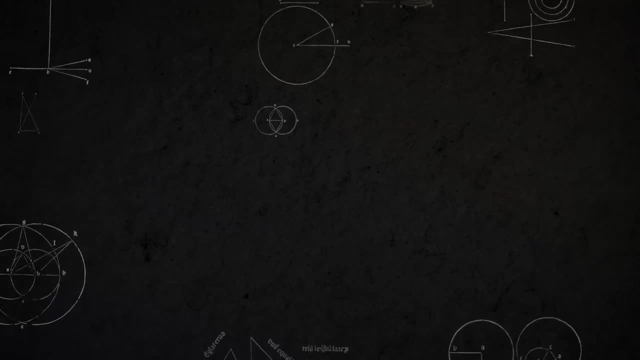 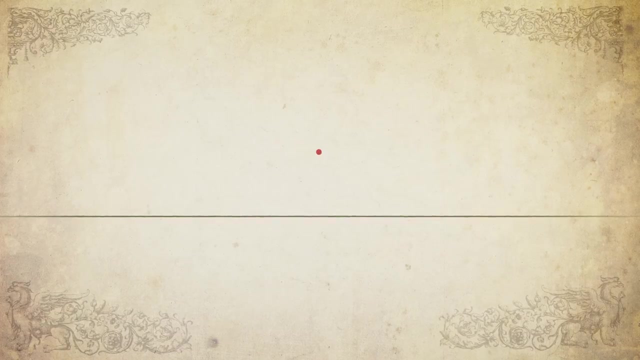 But they hadn't In fact. all they'd managed to do was just restate postulate 5 in different words. Here's one formulation: If you have a line and a point that is not on that line, then there is a single unique. 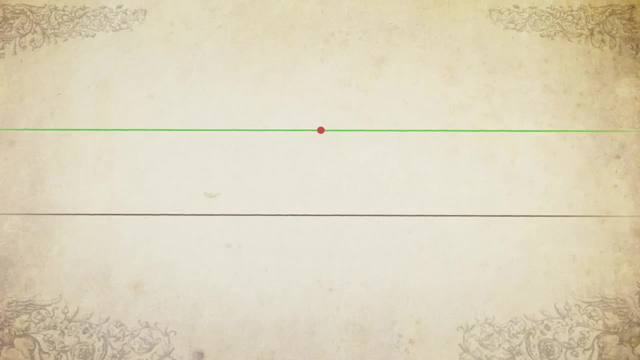 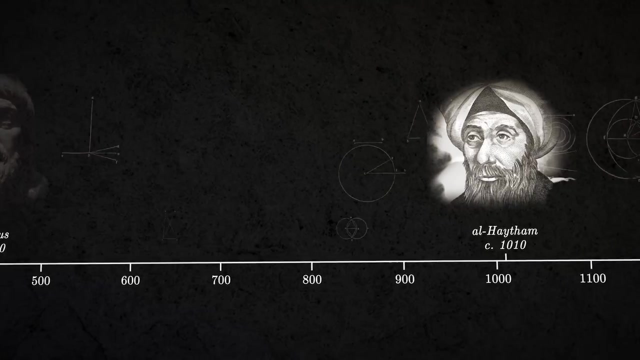 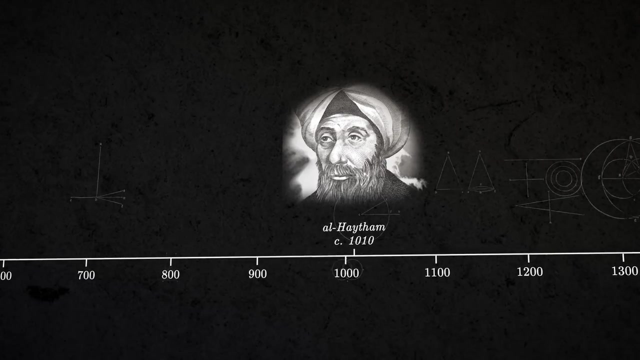 line which will be parallel to the first line. For this reason, the fifth postulate is often called the parallel postulate. When the method of direct proof failed, other mathematicians, including Al-Haytham and Omar Khayyam, tried a different approach: proof by contradiction. 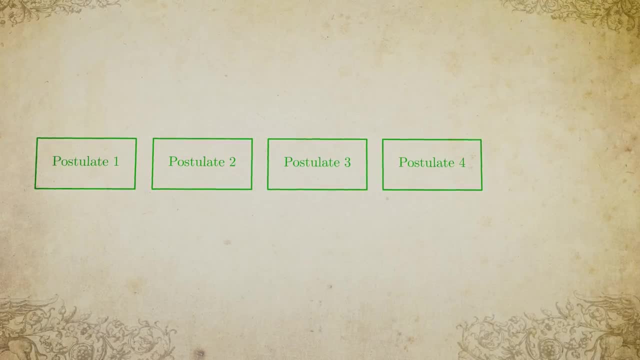 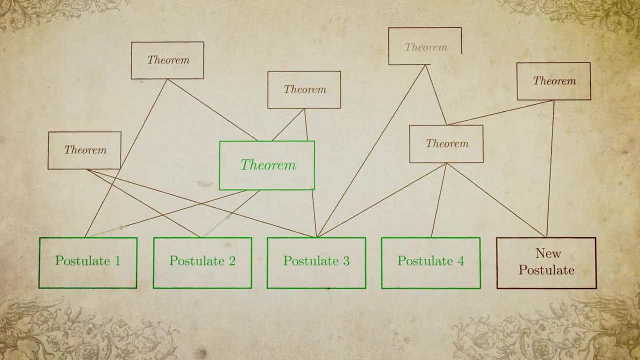 The idea is simple: You keep the first four postulates the same, but assume that the fifth postulate is false. Then you use those new postulates to prove theorems. If that leads to a contradiction- for example true equals false- then it means your new. 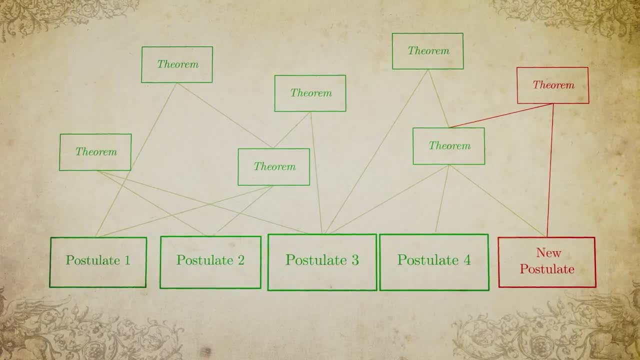 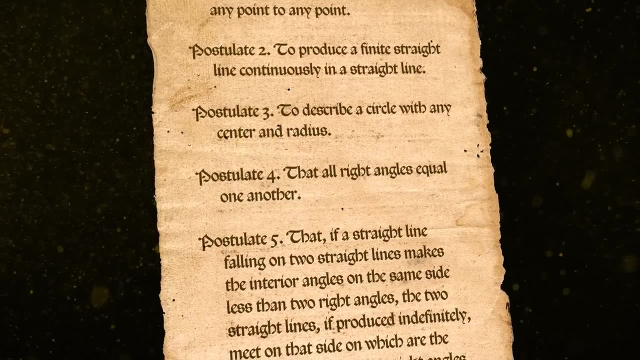 fifth postulate must be wrong. Therefore, the only remaining option would be that Euclid's version of the fifth postulate is correct, and you would have proven the fifth postulate. So what would it look like if the fifth postulate were false? 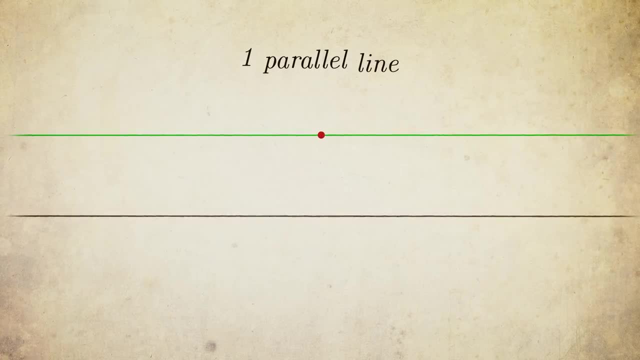 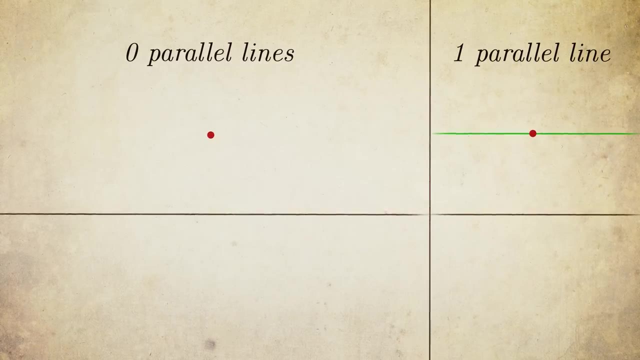 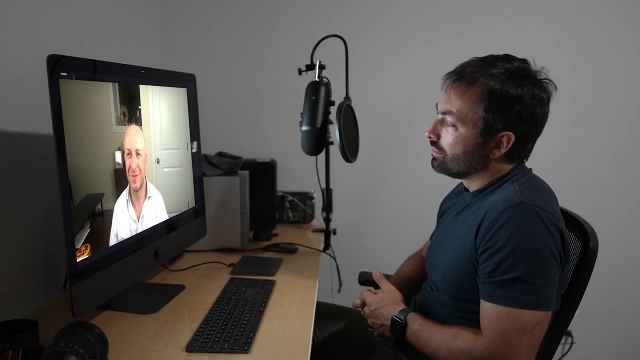 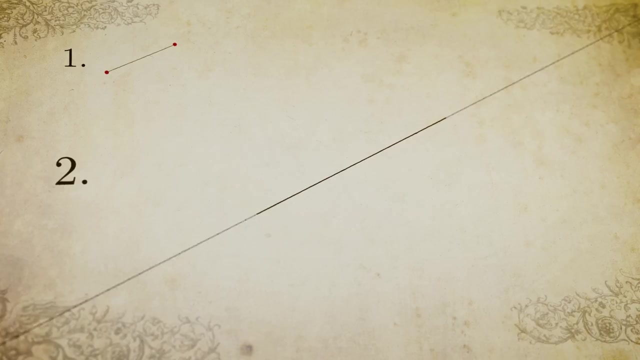 According to Euclid, through a point, not on a line, there could only be one line that is parallel to the first. One alternative is that there are no parallel lines that you could draw through that point, So this option was ruled out. It contradicted the second postulate, which states that lines can be extended indefinitely. 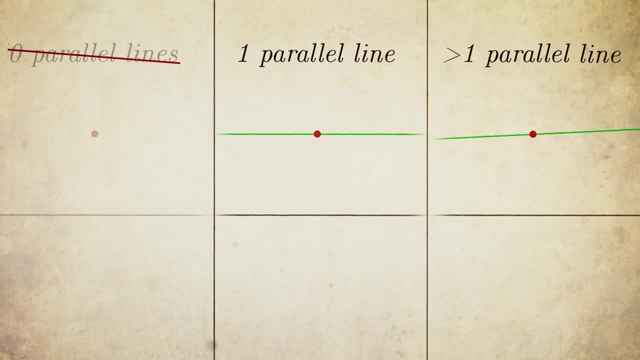 The other alternative is that you can draw more than one parallel line through a point, not on the first line. So that's what they would do. They would assume the postulate five fails And they're like. this has got to be wrong. 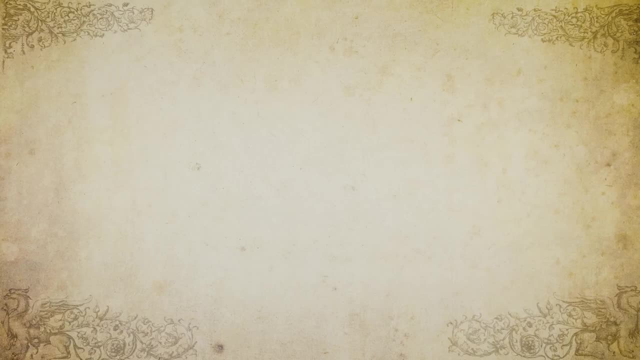 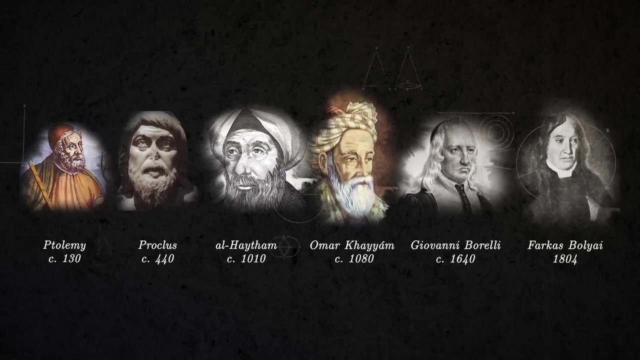 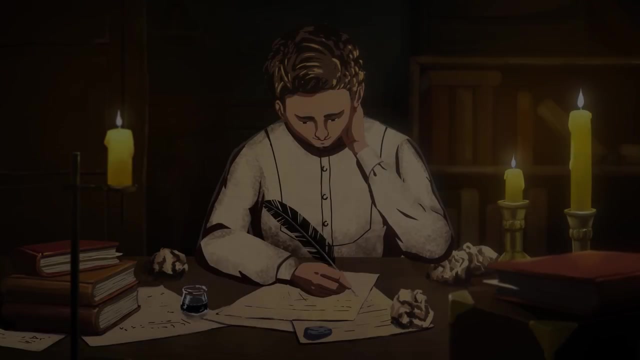 Where is the contra? They couldn't find the contradiction, So proof by contradiction also failed. In total, mathematicians spent more than 2,000 years trying to prove the fifth postulate, But everyone who tried failed. Then, around 1820, Janos Bolyai, a 17-year-old student, started spending his days and nights. 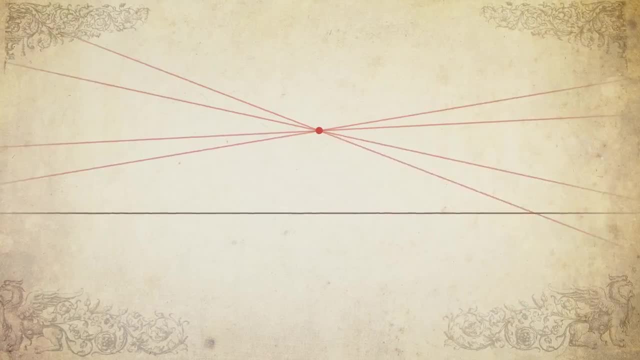 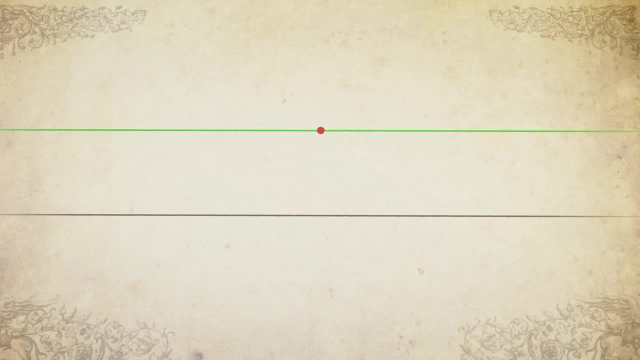 If you have a line and a point that is not on that line, then there is a single unique line which will be parallel to the first line. For this reason, the fifth postulate is often called the parallel postulate When The method of direct proof failed. 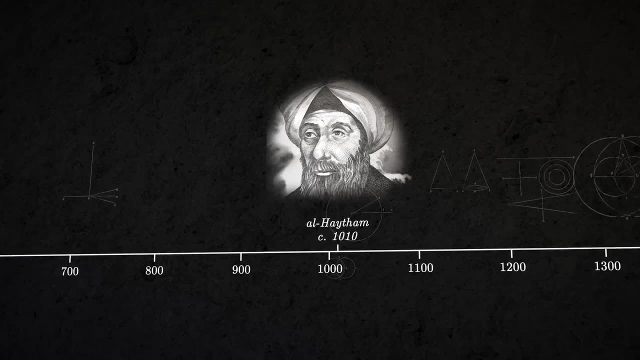 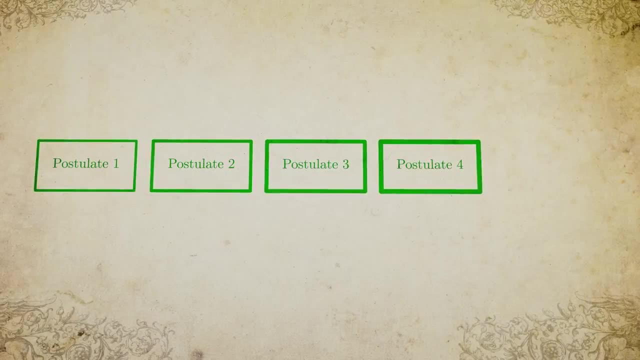 Other mathematicians, including Al-Haytham and Omar Khayyam, tried a different approach, Proof by contradiction. The idea is simple: You keep the first four postulates the same, but assume that the fifth postulate is false. 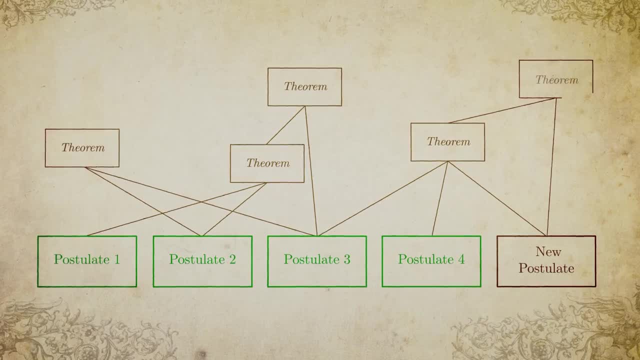 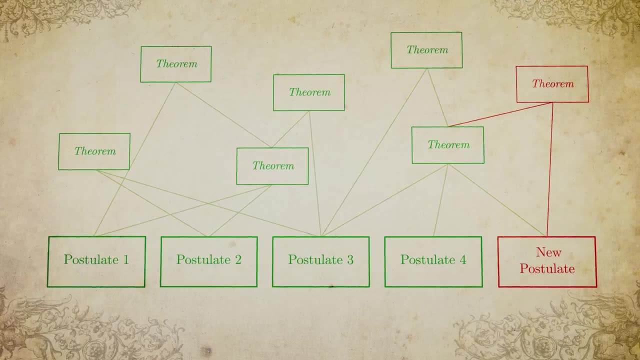 Then you use those new postulates to prove theorems, And if that leads to a contradiction- for example, true equals false- well then it means your new fifth postulate must be wrong. Therefore, the only remaining option would be that Euclid's version of the fifth postulate 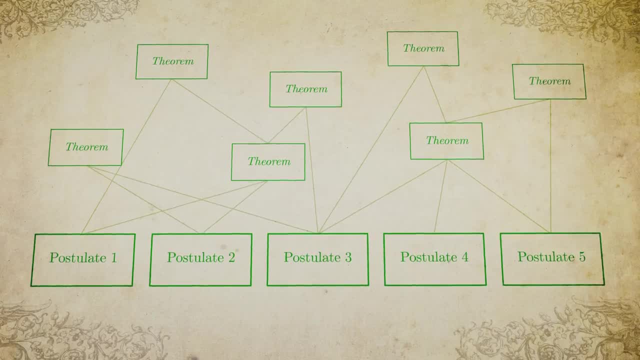 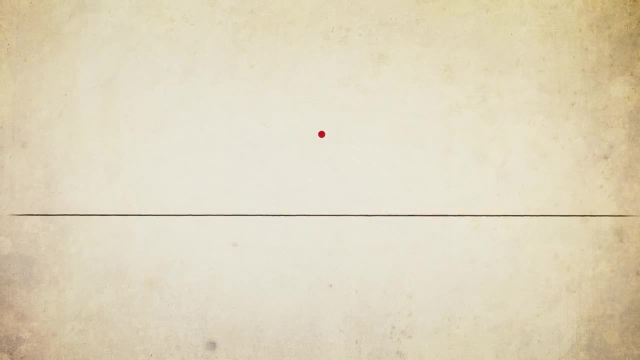 is correct and you would have proven the fifth postulate. So what would it look like if the fifth postulate were false? Well, according to Euclid, through a point, not on a line, there could only be one line that is parallel to the first. 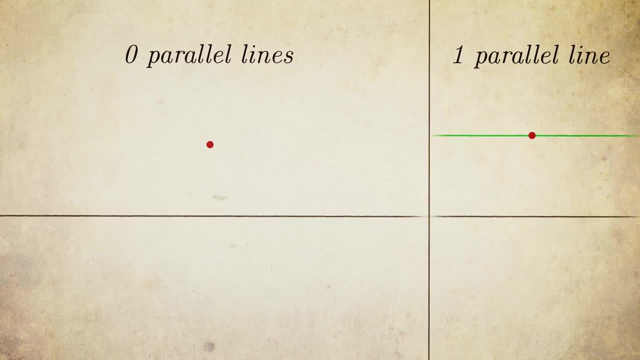 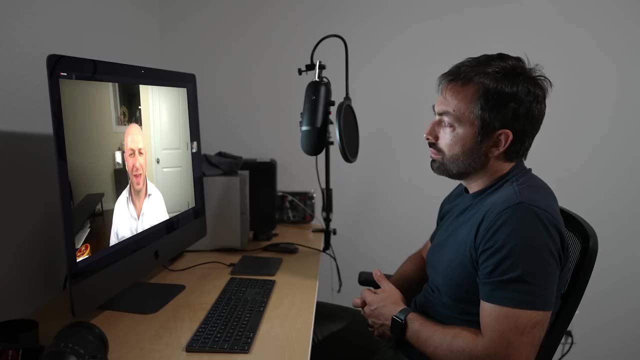 One alternative is that there are no parallel lines that you could draw through that point. Well, people tried that and they realized that then lines had to be finite in length And they're like: well, that can't be, So this option was ruled out. 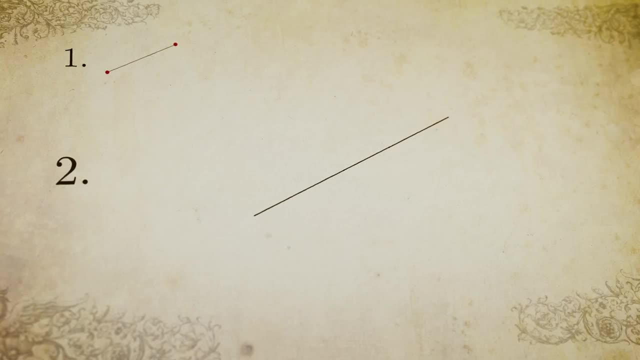 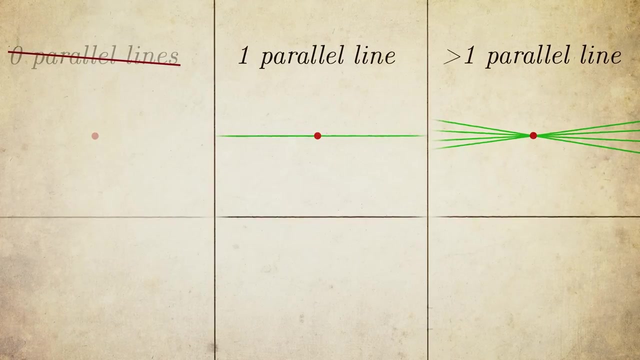 It contradicted the second postulate, which states that lines can't be parallel, Which states that lines can be extended indefinitely. The other alternative is that you can draw more than one parallel line through a point, not on the first line. So that's what they would do. They would assume the postulate five fails. 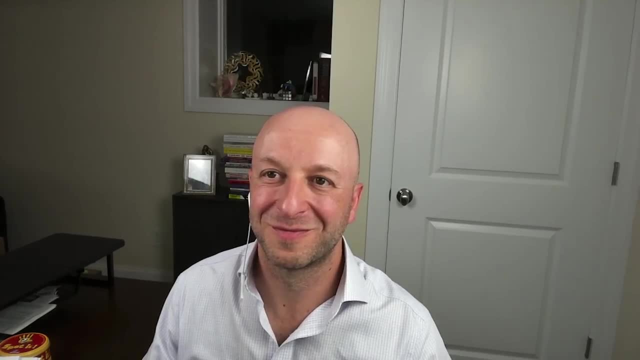 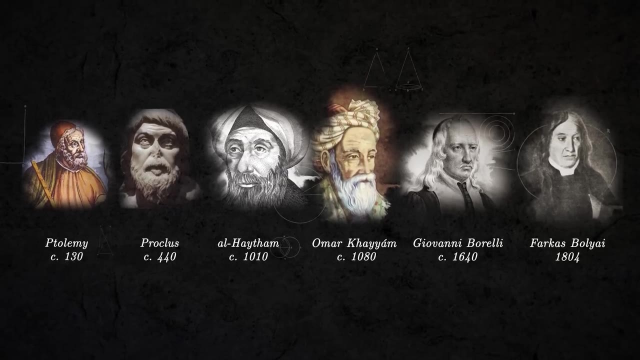 And they're like: this has got to be wrong. Where is the contra-? they couldn't find the contradiction, So proof by contradiction also failed. In total, mathematicians spent more than 2,000 years trying to prove the fifth postulate. 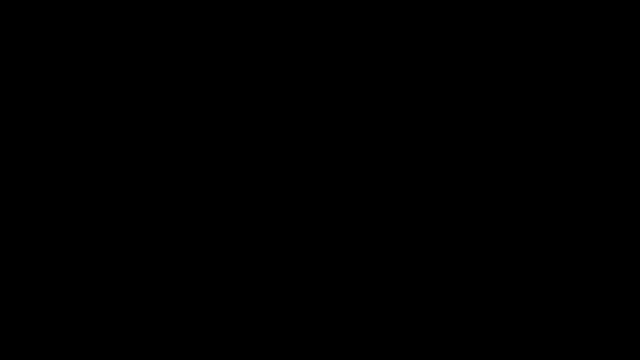 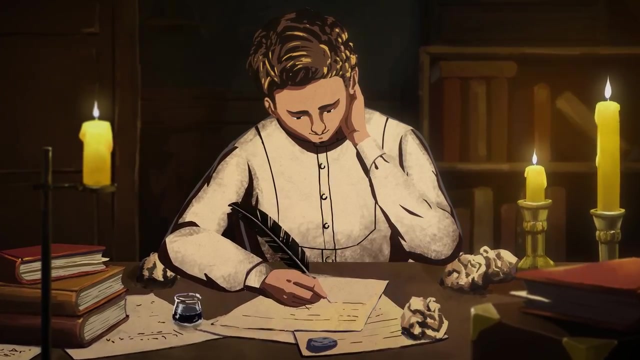 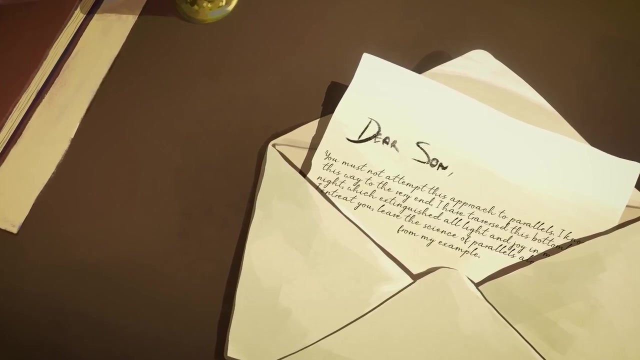 But everyone who tried failed. Then, around 1820, Janos Bolyai, a 17-year-old student, started spending his days and nights working on the mystery. His father became worried and he wrote to his son: You must not attempt this approach to parallels. I know this way to the very end. 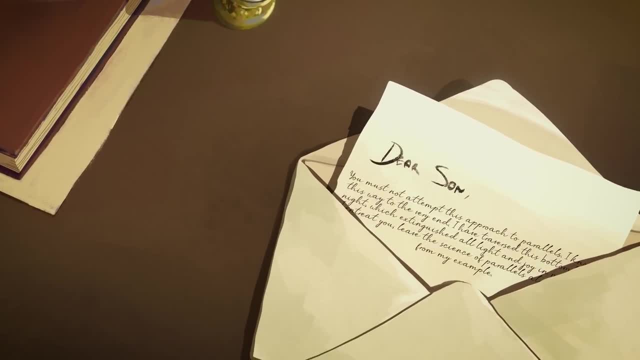 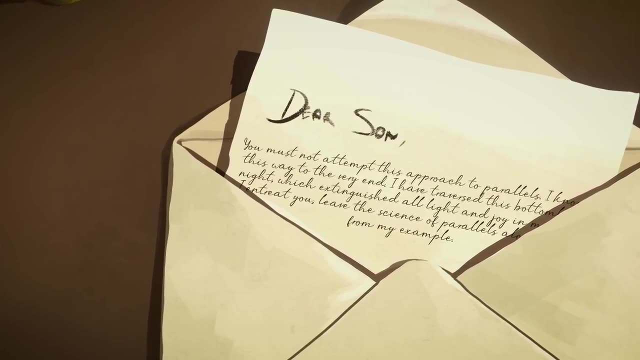 working on the mystery. His father became worried and he wrote to his son: You must not attempt this approach to parallels. I know this way. to the very end. I have traversed this bottomless night which extinguished all light and joy in my life. 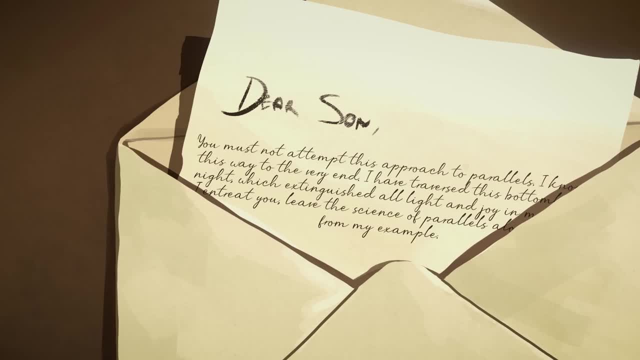 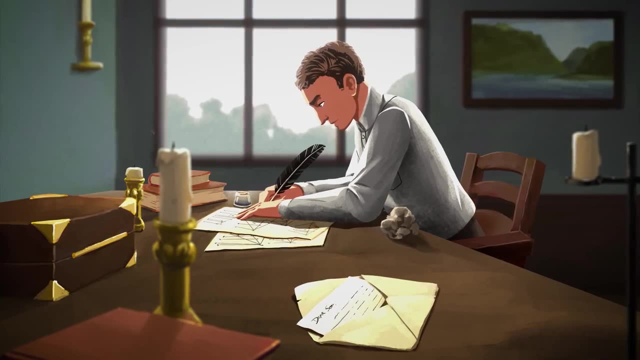 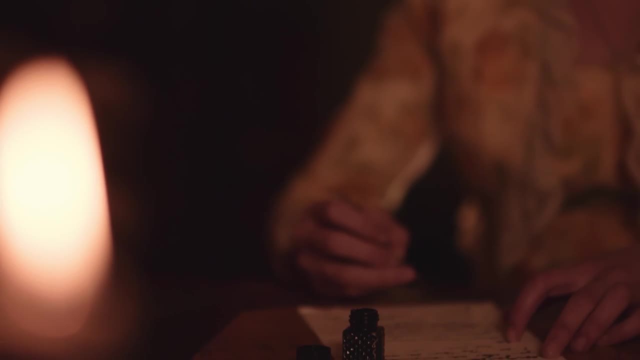 I entreat you, leave the science of parallels alone. Learn from my example. But the young Bolyai didn't listen to his father. He could not leave the science of parallels alone. After years of work he realized that maybe the fifth postulate can't be proven from the 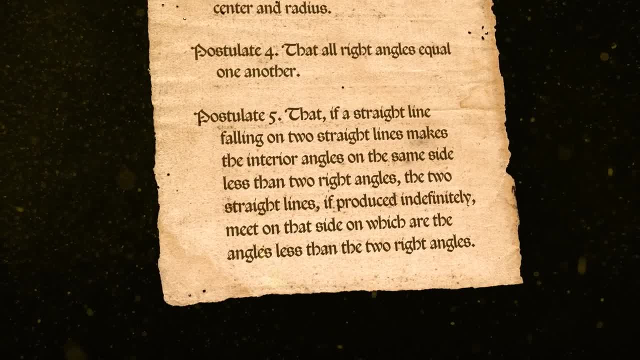 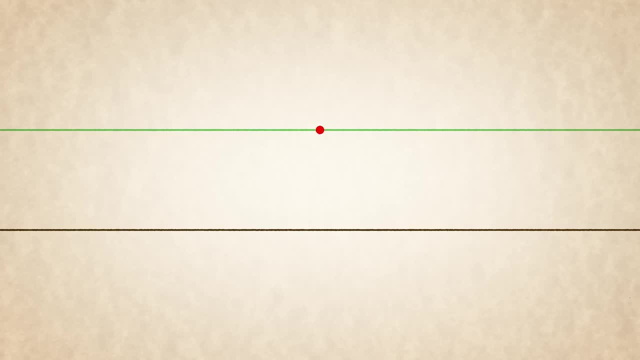 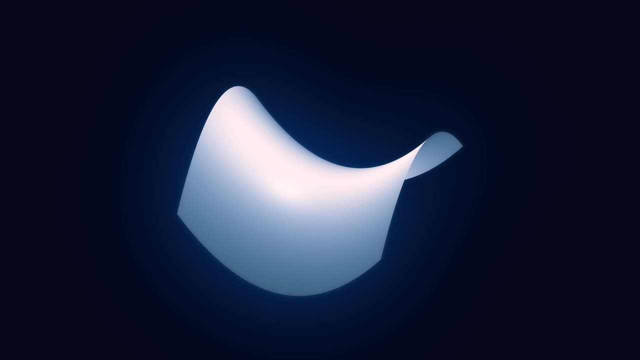 other four, It could be completely independent. See, according to Euclid, you could have only one parallel line through a point, but Bolyai imagined a world where there could be more than one parallel line through that point. But how Well. who said you needed to have a flat surface? 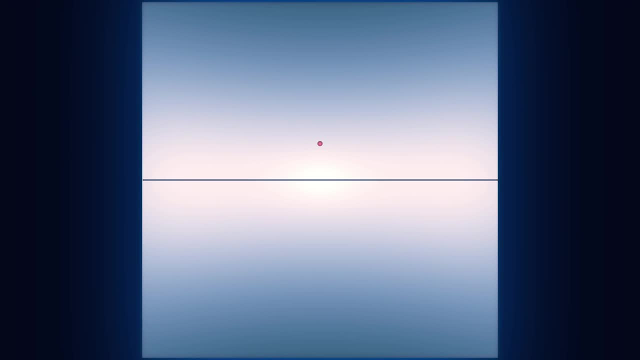 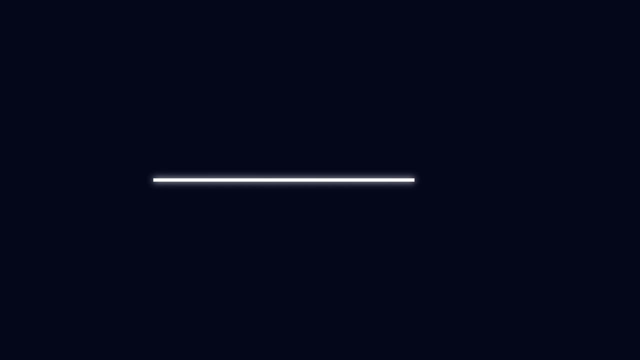 On a surface that is curved like this, you can draw more than one line that is parallel to the original line, But wait a second, those lines don't look straight. Well, What makes straight lines special is that they're the shortest paths between two points. 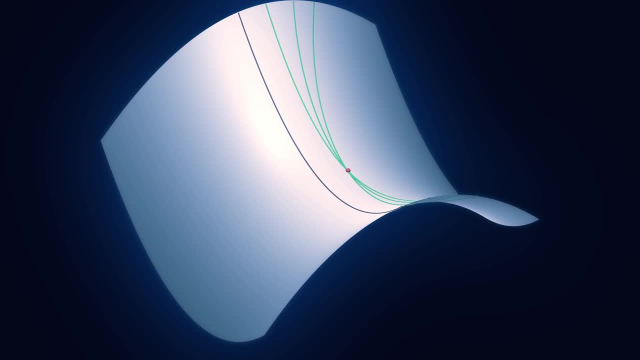 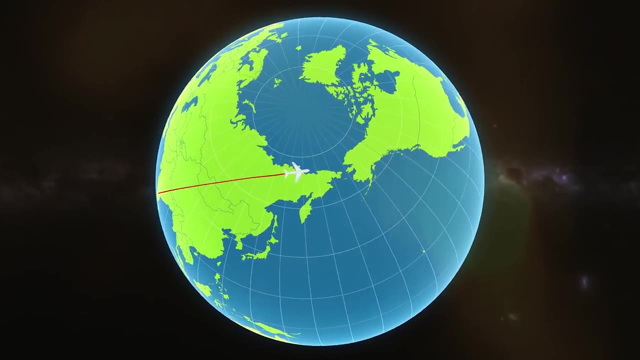 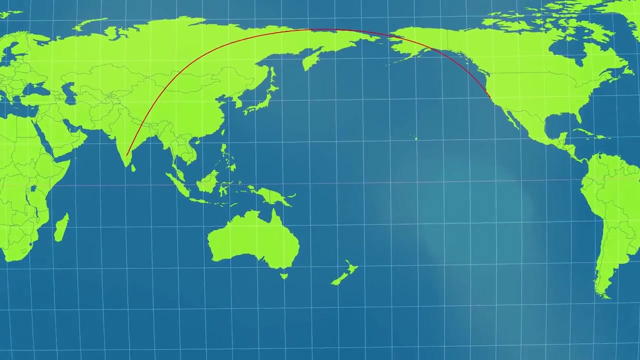 On this surface, those shortest paths just look bent because the surface is curved. Here's a more familiar example: Airplanes always try to fly the shortest path between two cities. They're basically flying in a straight line, But that line doesn't look straight on a map because the surface is curved. 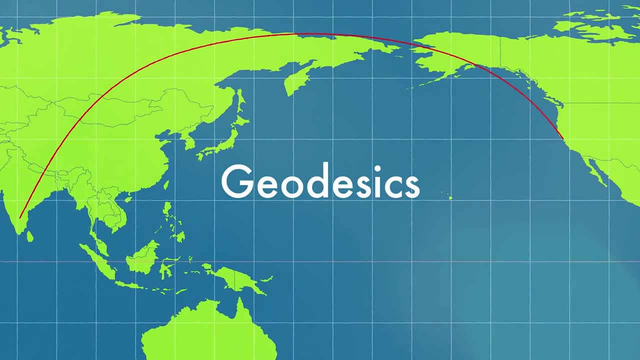 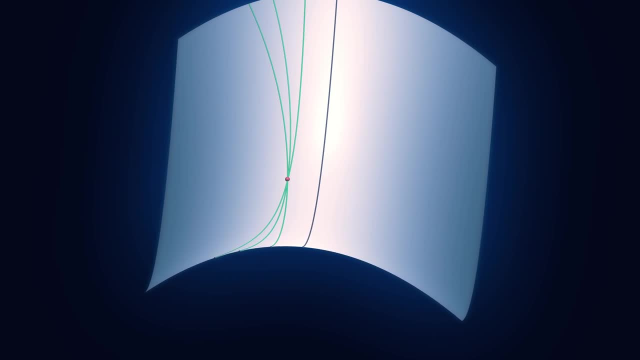 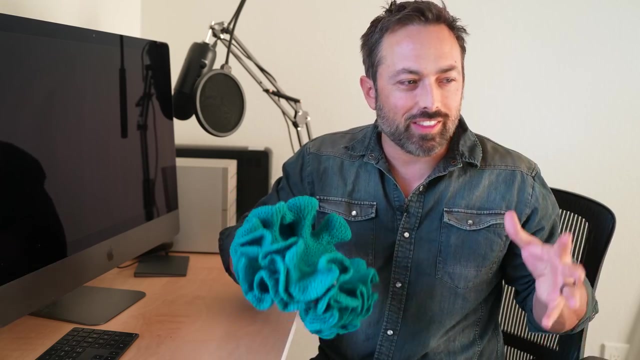 These shortest paths on curved surfaces are called geodesics. So all these lines are straight And they just don't look it, because the world Bolyai had imagined turned out to be curved. We now know this as hyperbolic geometry. You know, when I used to think of the hyperbolic plane, I would just imagine it as one giant. 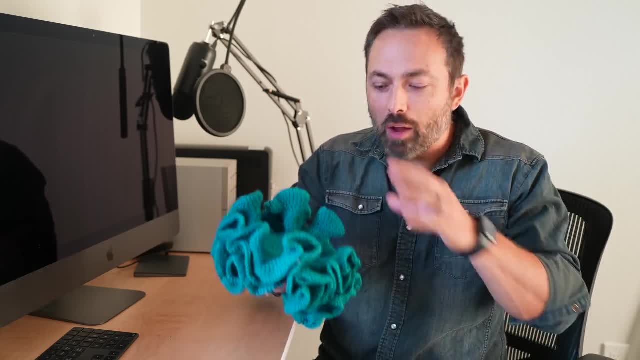 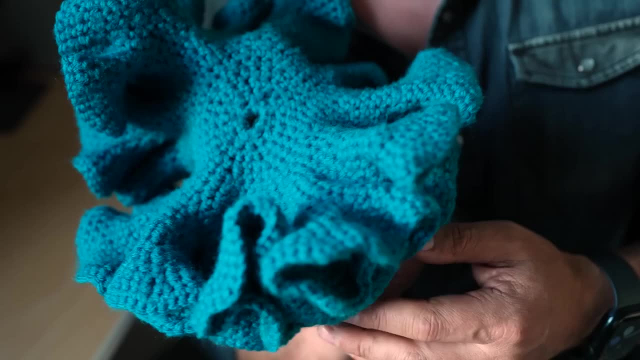 saddle, But that's not really what it is. The hyperbolic plane is much more like this piece of crocheting. So it starts out pretty flat and even in the middle, But as you move outwards, more and more fabric is created. 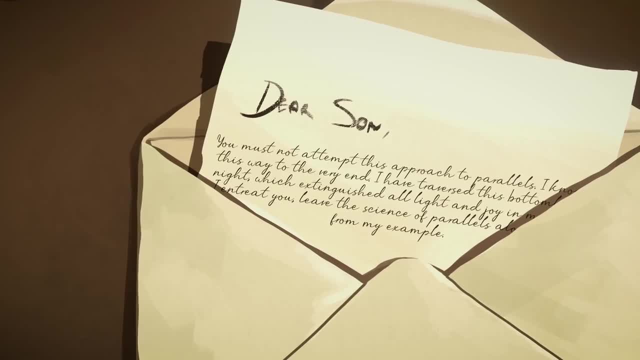 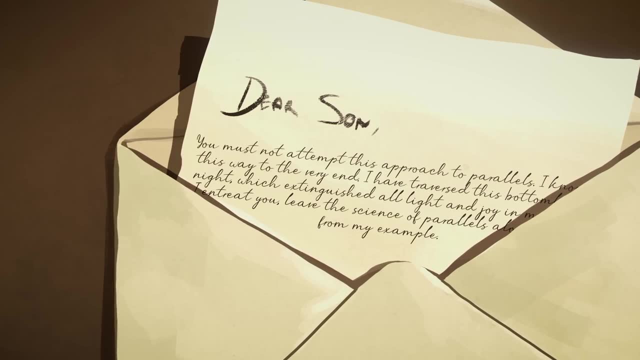 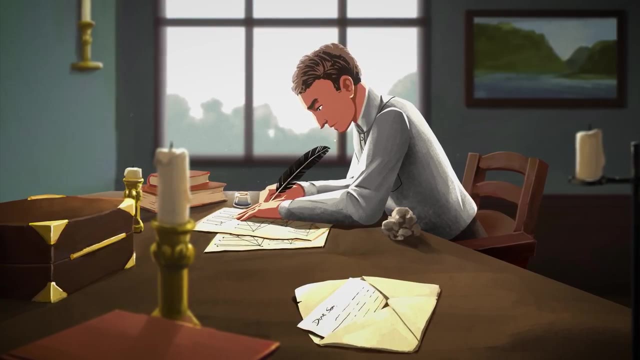 I have traversed this bottomless night which extinguished all light and joy in my life. I entreat you, leave the science of parallels alone. Learn from my example. But the young Bolyai didn't listen to his father. He could not leave the science of parallels alone. 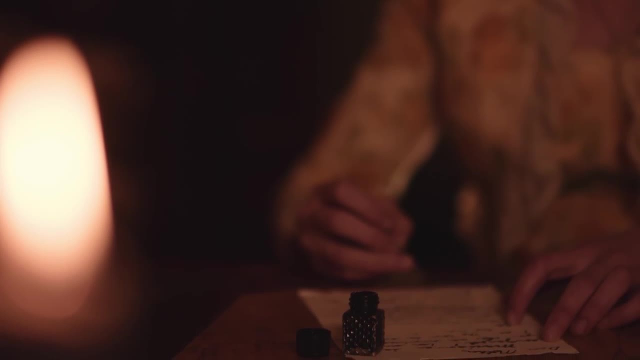 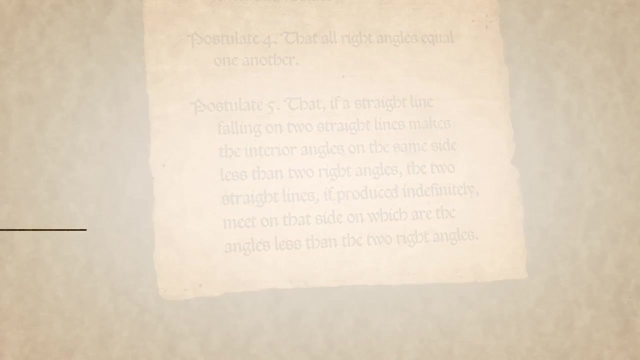 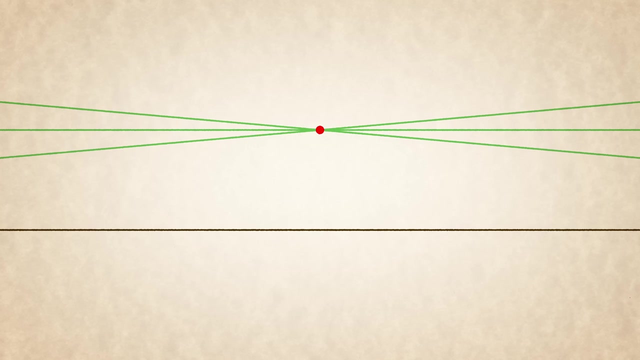 After years of work he realized that maybe the fifth postulate can't be proven from the other four. It could be completely independent. See, according to Euclid you could have only one parallel line through a point, But Bolyai imagined a world where there could be more than one parallel line through that point. 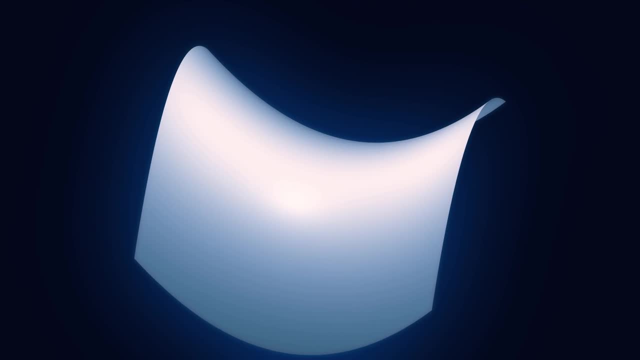 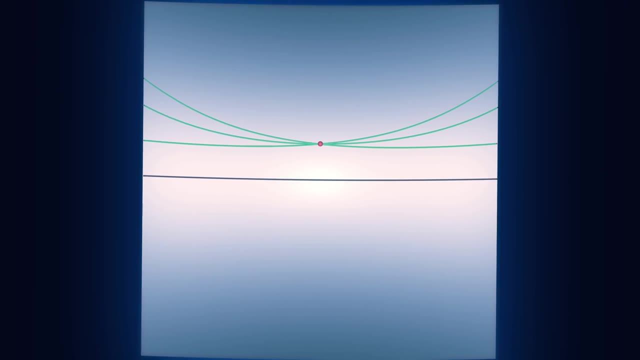 But how Well. who said you needed to have a flat surface? On a surface that is curved like this, you can draw more than one line that is parallel to the original line. But wait a second, those lines don't look straight. 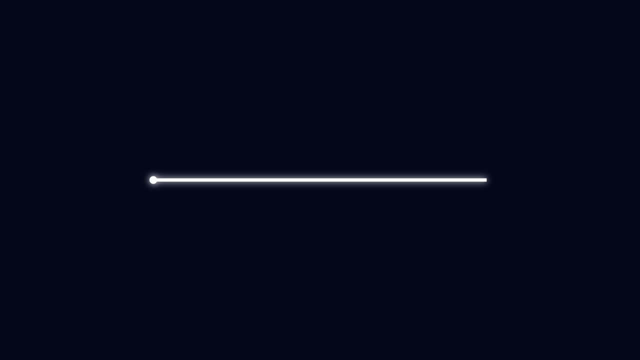 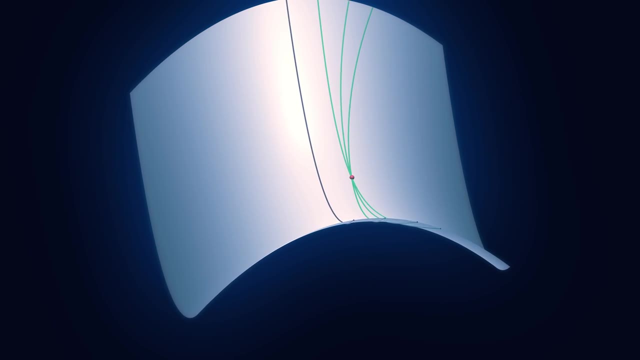 Well, what makes straight lines special is that they're the shortest paths between two points. On this surface, those shortest paths just look bent because the surface is curved. Here's a more familiar example: Airplanes always try to fly the shortest path between two cities. 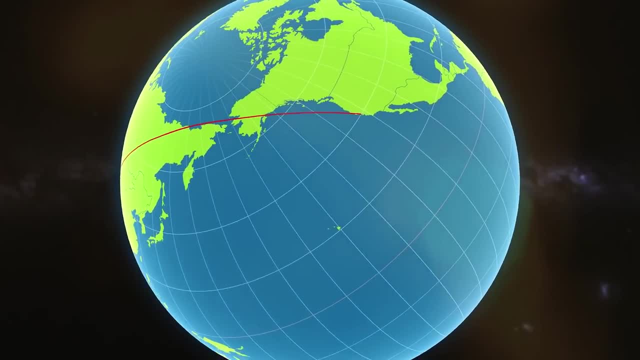 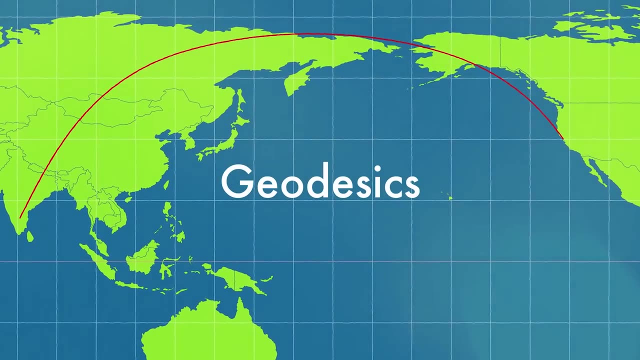 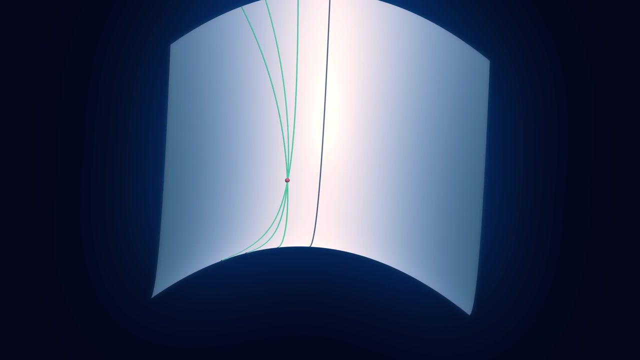 They're basically flying in a straight line, But that line doesn't look straight on a map because the surface is curved. These shortest paths on curved surfaces are called geodesics. So all these lines are straight. They just don't look it because the world Bolyai had imagined turned out to be curved. 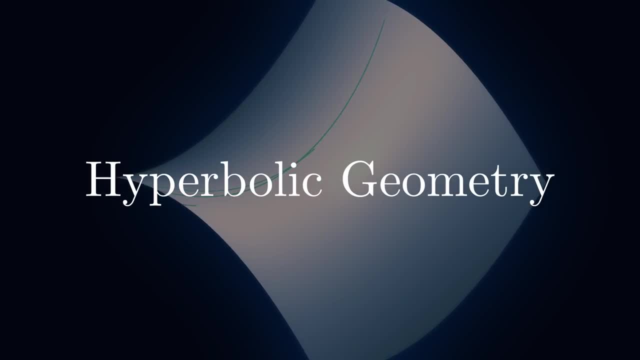 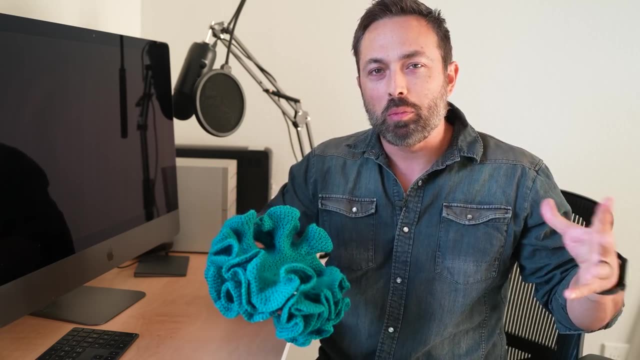 We now know this as hyperbolic geometry. You know, when I used to think of the hyperbolic plane, I would just imagine it as one giant saddle, But that's not really what it is. The hyperbolic plane is much more like this piece of crocheting. 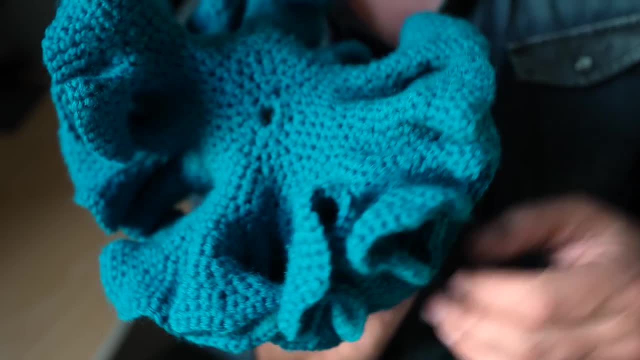 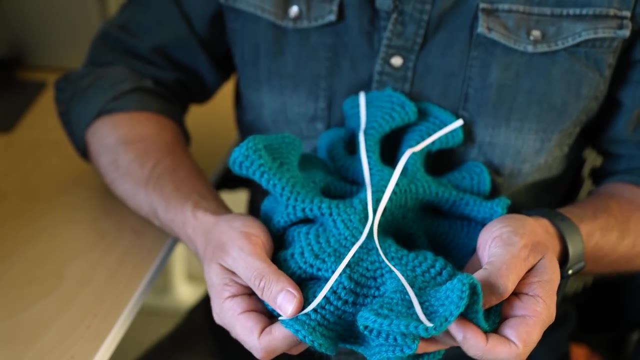 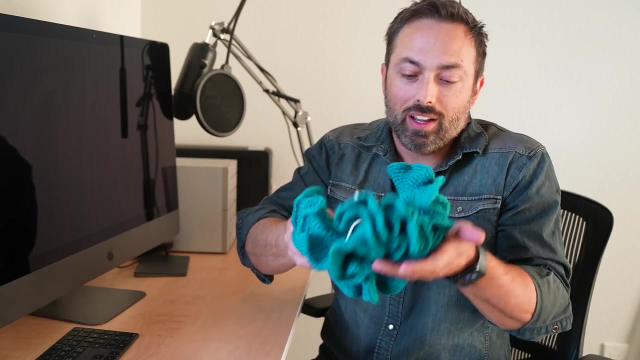 So it starts out pretty flat and even in the middle. But as you move outwards, more and more fabric is created, And that would push parallel lines apart. And the further and further out you go, the amount of fabric grows exponentially And that ends up causing this crumpling effect. 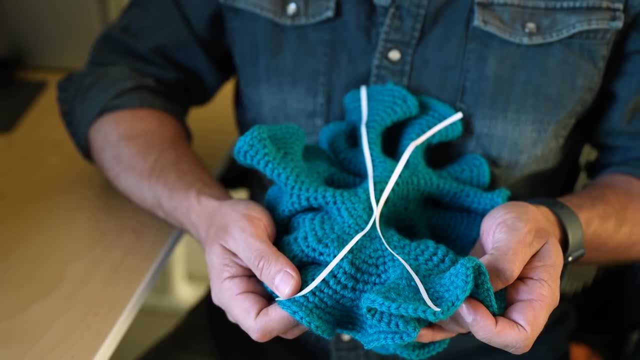 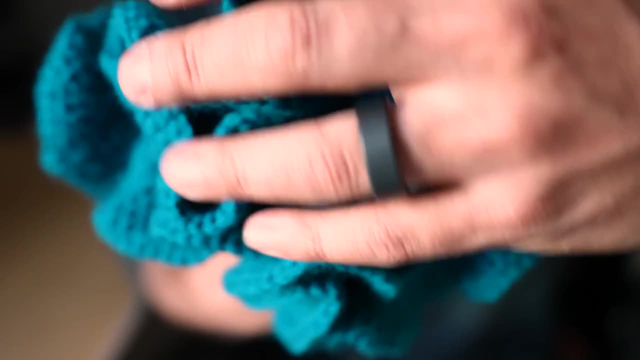 And that would push parallel lines apart. And the further and further out you go, the amount of fabric grows exponentially And that ends up causing this crumpling effect. So if you really want to think about the hyperbolic plane, I think you've got to think about saddles. 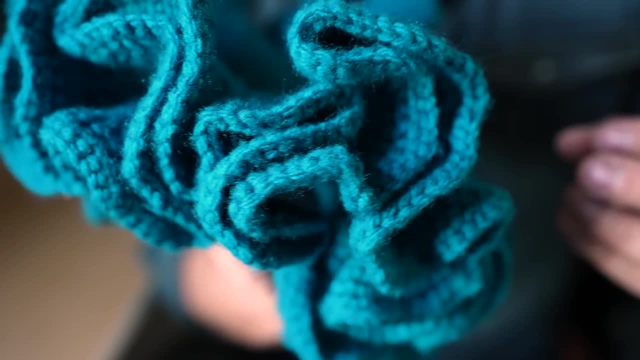 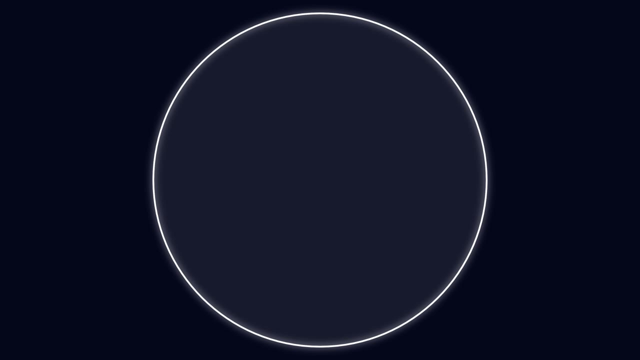 on saddles, on saddles, like it's an infinite crumpling mess. But that little piece of crochet isn't the full hyperbolic plane. To show that we need to make a map, One that fits the entire plane, One that fits the entire plane into a disc. 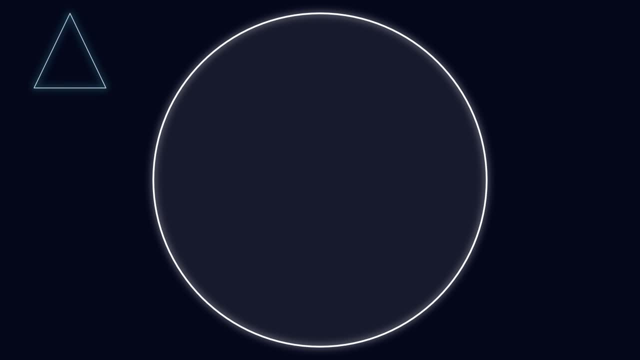 To show how this works, we're going to fill the entire plane with these triangles Starting in the middle, just as with the crochet. things look pretty normal, But as you go farther out from the center, you get all this extra space, so you can fit. 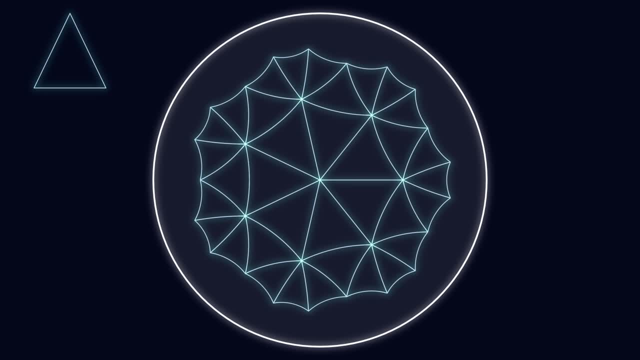 more and more triangles, So they appear smaller, but they are actually the same size. Now, since the hyperbolic plane is infinite, you can keep adding triangles forever And they all need to fit on the disc. So as you get closer to the center, you can add more triangles. 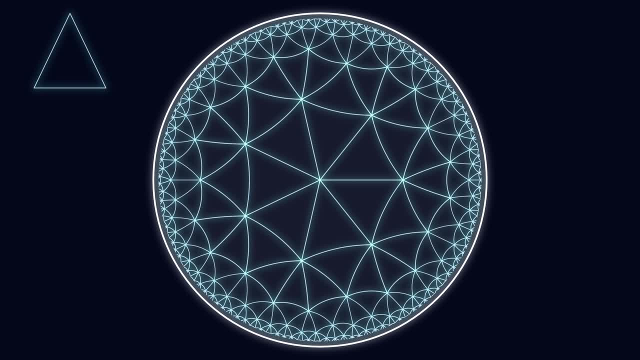 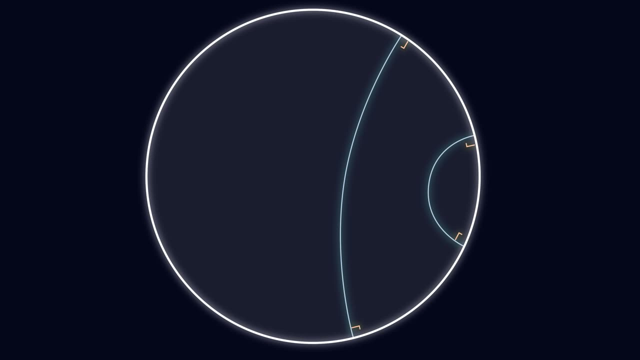 And as you get closer to the edge, the triangles will appear smaller and smaller and smaller, Infinitely smaller, never ending, and you can never quite reach the edge. This is known as the Poincaré disc model. Here, straight lines are arcs of circles that intersect the disc at 90 degrees. 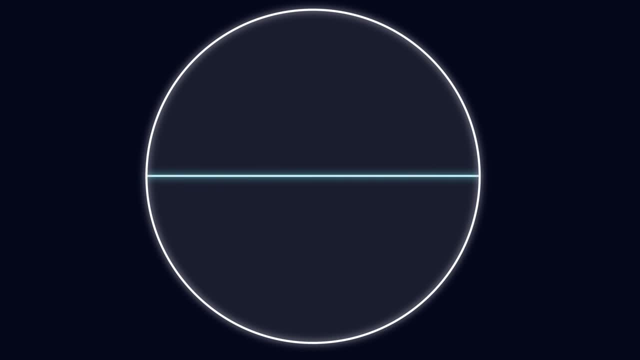 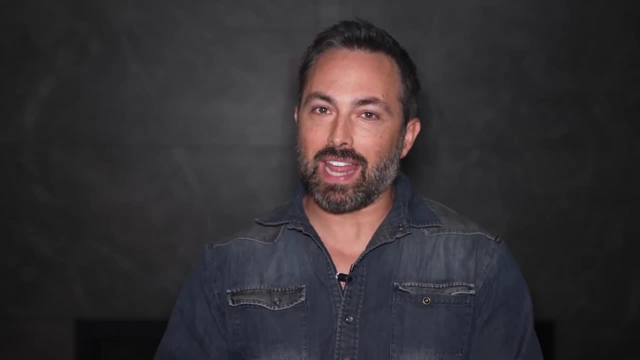 And, just like on our original shape, a straight line down the middle appears straight, while straight lines next to it appear to curve away. What's remarkable is that Bollii didn't have a model like this in the first place. They didn't have a model like this in the first place. 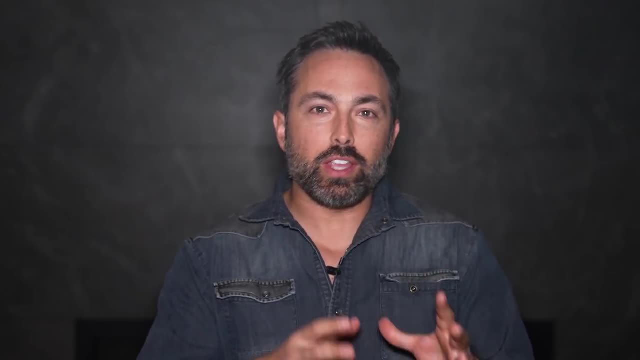 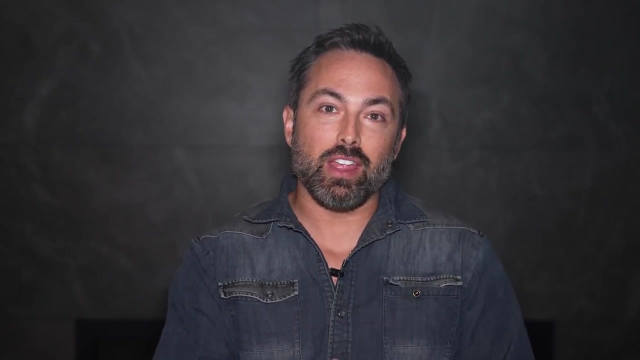 They didn't have a model of hyperbolic geometry yet. He was just drawing Euclidean triangles with the assumption that Euclid's fifth postulate didn't hold, And while Bollii found that the behavior in hyperbolic geometry is very different than 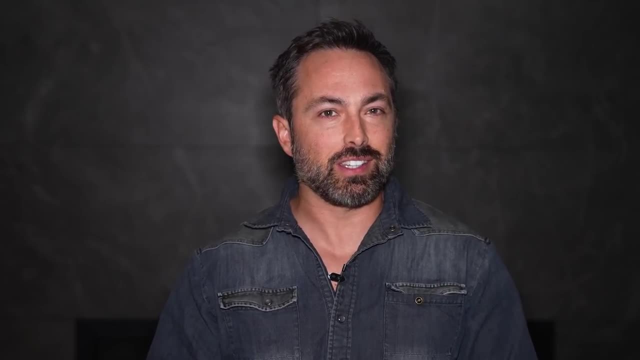 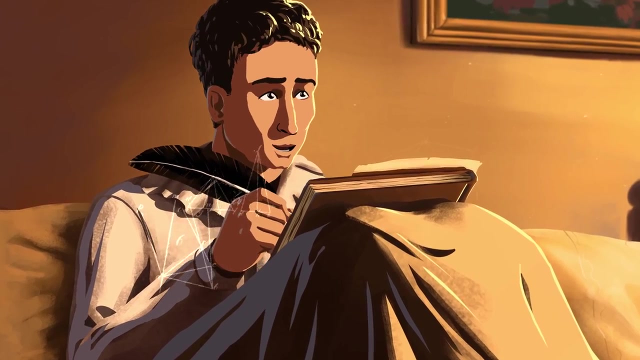 Euclid's. mathematically, it seemed just as consistent. In 1823, the 20-year-old Janos wrote to his dad: I have discovered such wonderful things that I was amazed Out of nothing, Out of nothing, Out of nothing. 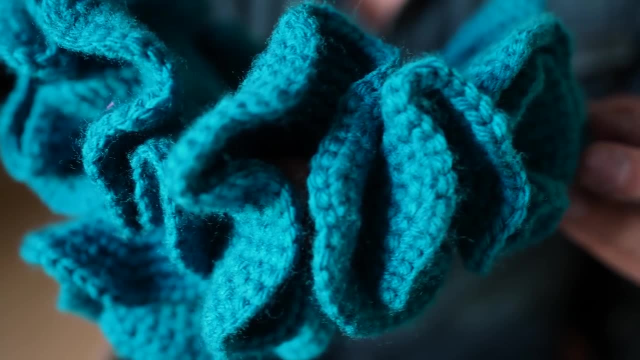 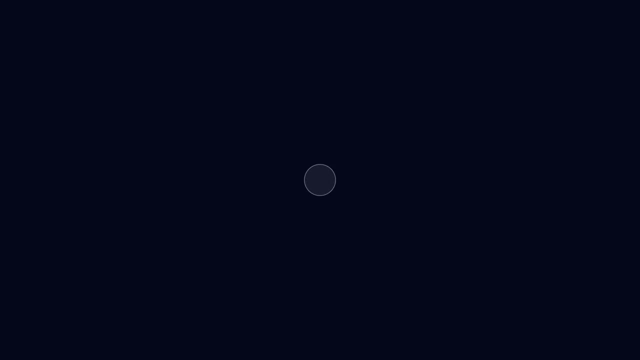 So if you really want to think about the hyperbolic plane, I think you've got to think about saddles on saddles, on saddles- Like it's an infinite crumpling mess. But that little piece of crochet isn't the full hyperbolic plane. 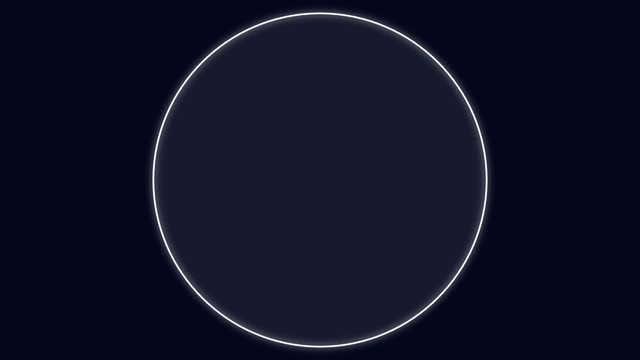 To show that we need to make a map, One that fits the entire plane into a disc, To show how this works. we're going to fill the entire plane with these triangles Starting in the middle, just as with the crochet. things look pretty normal. 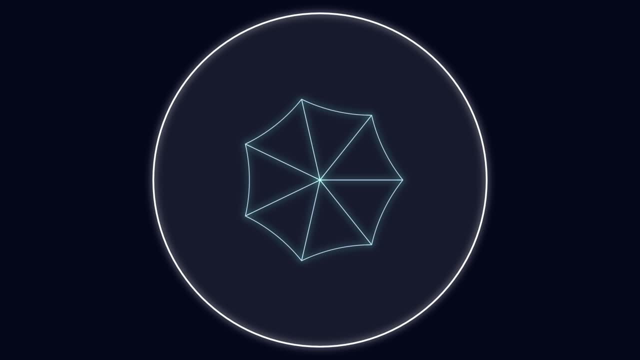 But as you go farther out from the center, you get all this extra space, So you can fit more and more triangles. So they appear smaller, but they are actually the same size. Now, since the hyperbolic plane is infinite, you can keep adding triangles forever. 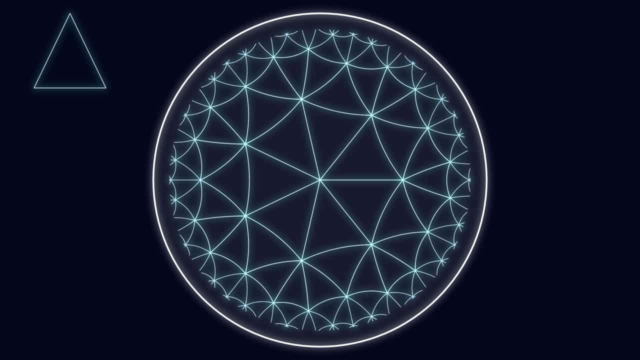 And they all need to fit on the disc. So as you get closer to the edge, the triangles will appear smaller and smaller and smaller, Infinitely smaller, never ending, And you can never quite reach the edge. This is known as the Poincaré Disc Model. 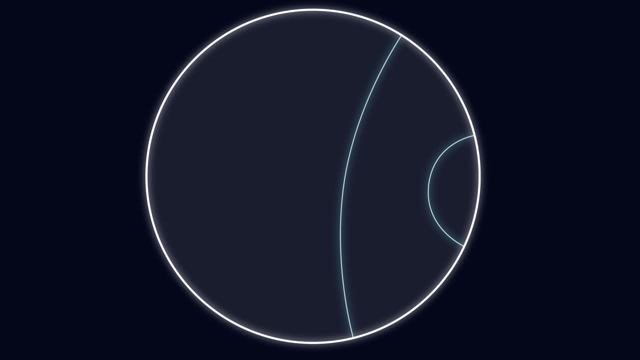 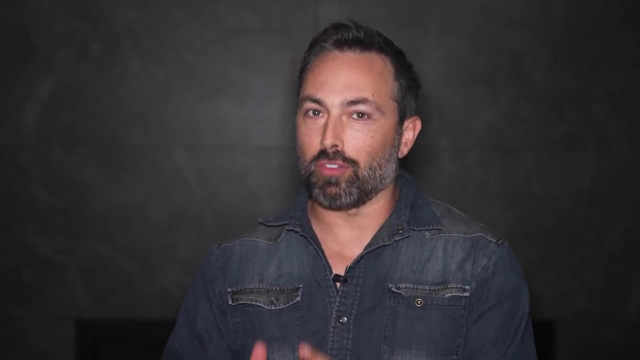 Here, straight lines line up. Straight lines are arcs of circles that intersect the disc at 90 degrees And, just like on our original shape, a straight line down the middle appears straight, While straight lines next to it appear to curve away. What's remarkable is that Baliai didn't have a model of hyperbolic geometry yet. 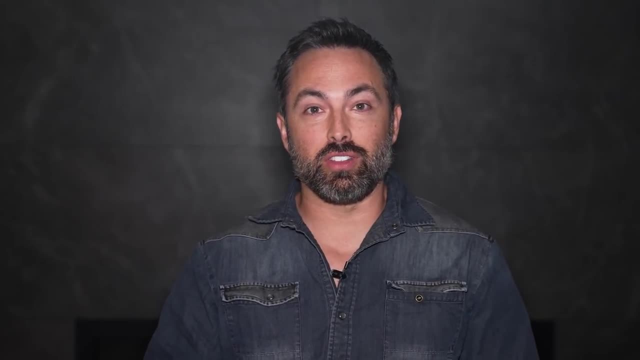 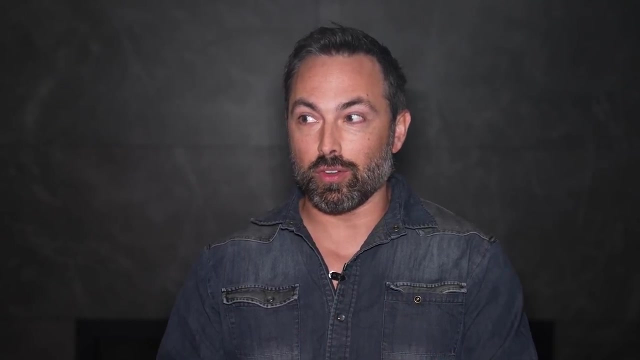 He was just drawing Euclidean triangles with the assumption that Euclid's Fifth Postulate didn't hold, And while Baliai found that the behavior in hyperbolic geometry is very different than Euclid's, mathematically it seemed just as consistent. 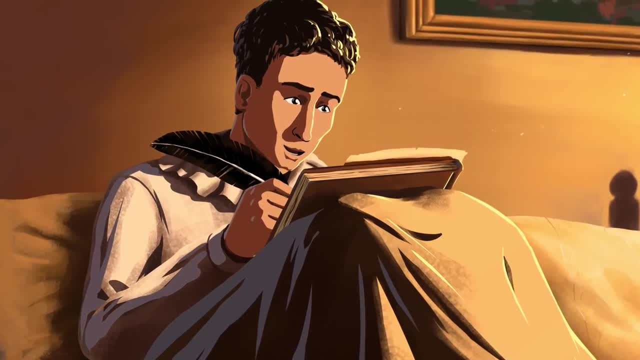 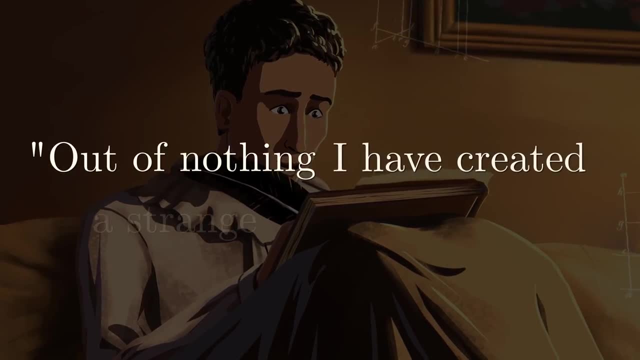 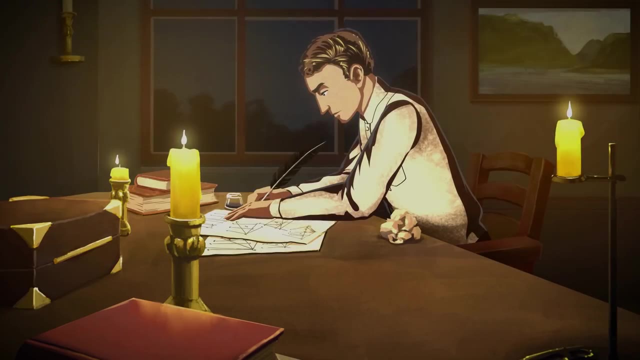 In 1823, the 20-year-old Janos wrote to his dad: I have discovered such wonderful things that I was amazed. Out of nothing I have created a strange new universe. But Baliai had been doing more than just tackling ancient math mysteries. 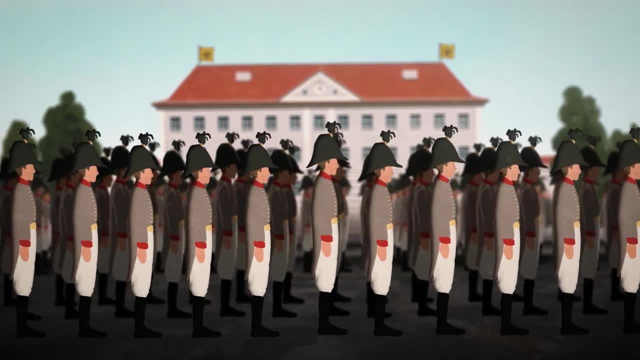 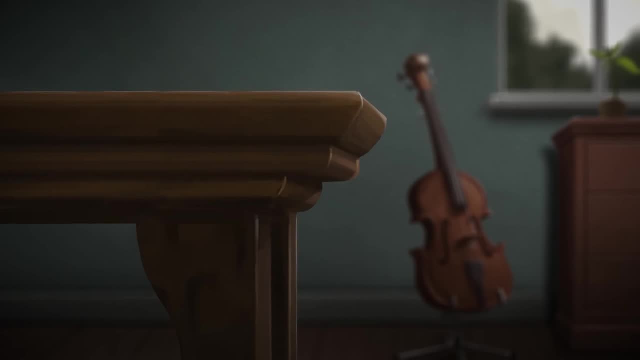 In his 20s he joined the army, where he continued developing two of his own, Two of his other passions: Playing the violin and dueling. He had mastered both, but with a sword in particular, he was unmatched, Perhaps because of his many talents. 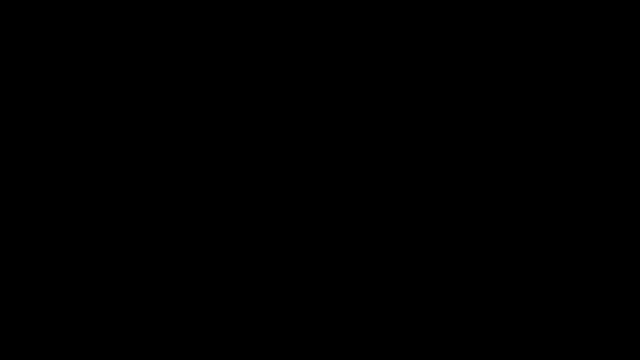 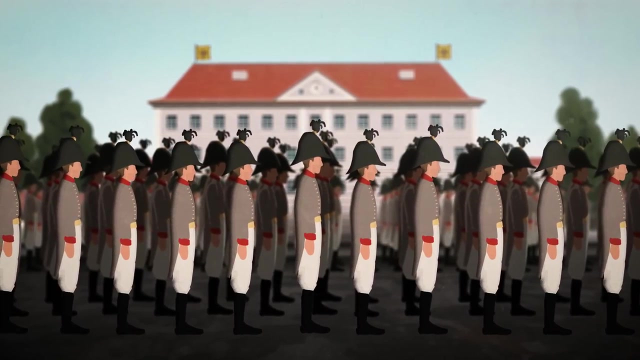 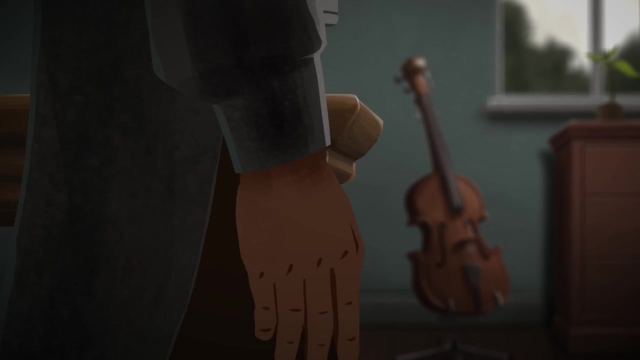 Out of nothing I have discovered a strange new universe. But Bollii had been doing more than just tackling ancient math mysteries. In his twenties he joined the army, where he continued developing two of his other passions — playing the violin and dueling. 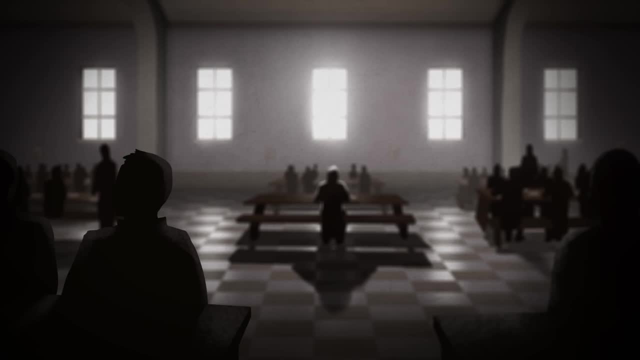 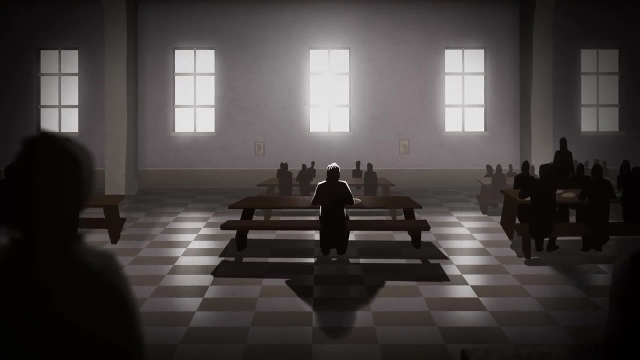 He had mastered both, but with a sword in particular, he was unmatched. Perhaps because of his many talents, Bollii grew arrogant and found it difficult to accept him, hard to get along with. This reached a peak when, during one of his deployments. 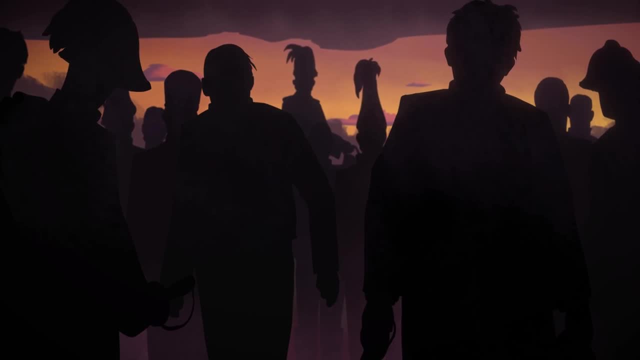 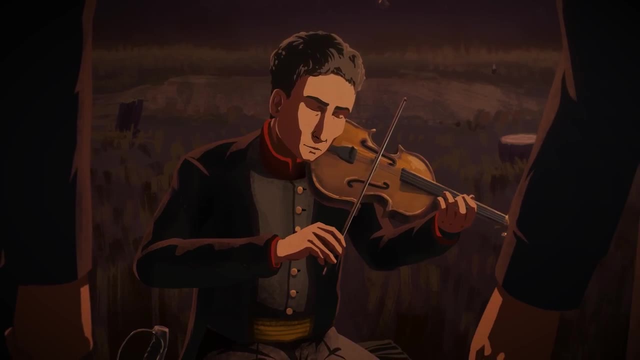 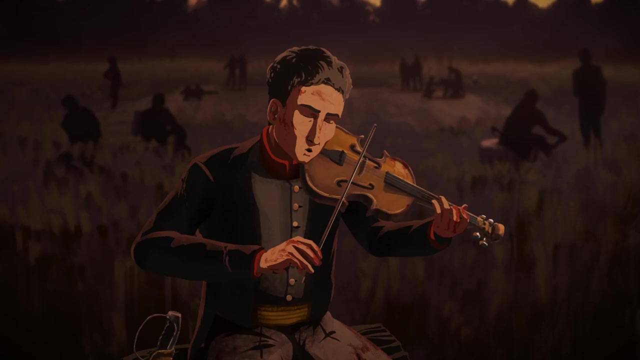 13 cavalry officers from his garrison challenged him to a duel. Boliai accepted their challenge on the condition that after every two duels, he could play for a little while on his violin. Boliai fought each of them in succession, winning all 13 duels and leaving behind all his adversaries. on the square. While Boliai loved dueling, his first love was still mathematics. In 1832, nine years after he discovered his strange new universe, he published his findings as a 24-page appendix to his father's textbook, Extremely proud and excited about his son's work. 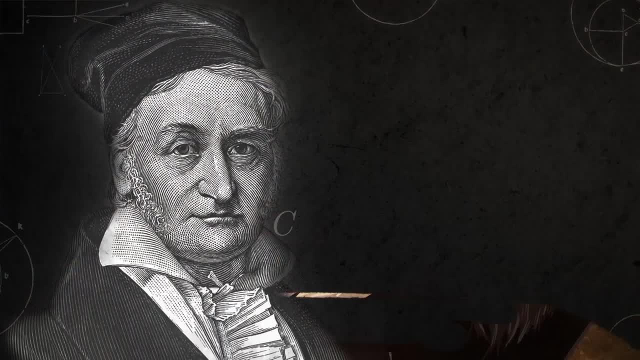 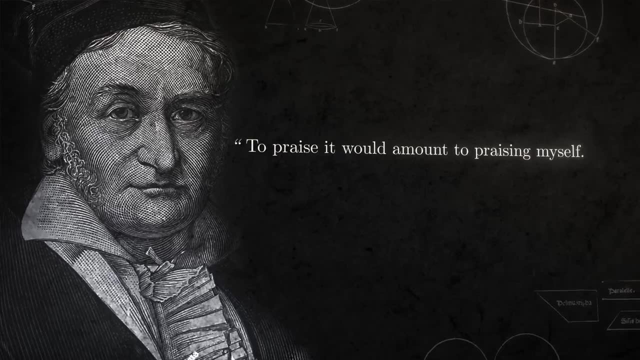 Farkas Boliai sent it to perhaps the greatest mathematician of all time, Carl Friedrich Gauss. After careful examination, Gauss replied a few months later. To praise it would amount to praising myself, for the entire content of the work coincides. 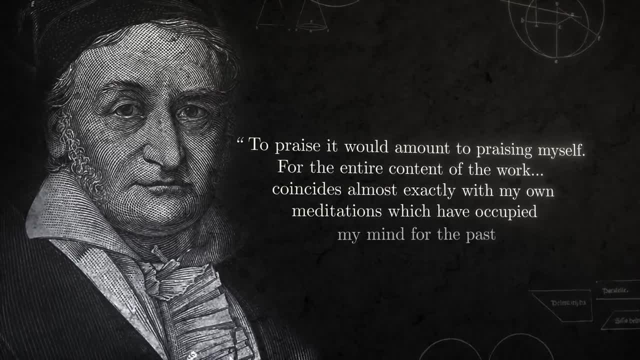 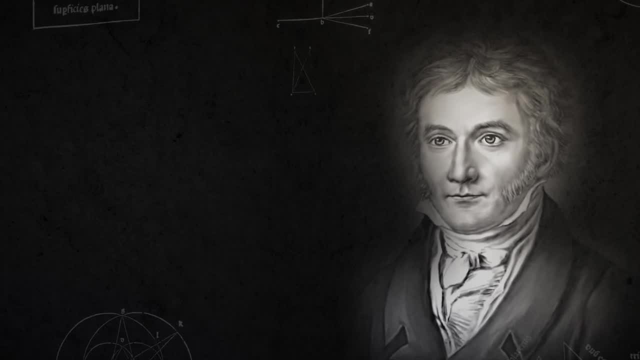 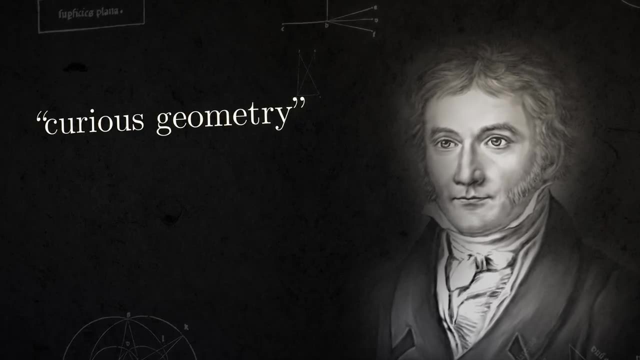 almost exactly with my own meditations which have occupied my mind for the past 30 or 35 years. Years earlier, Gauss had wandered a similar path. In 1824, he wrote a private letter to one of his friends in which he describes discovering a curious geometry, one with 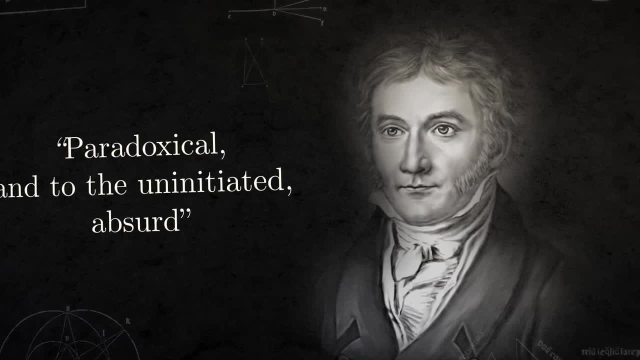 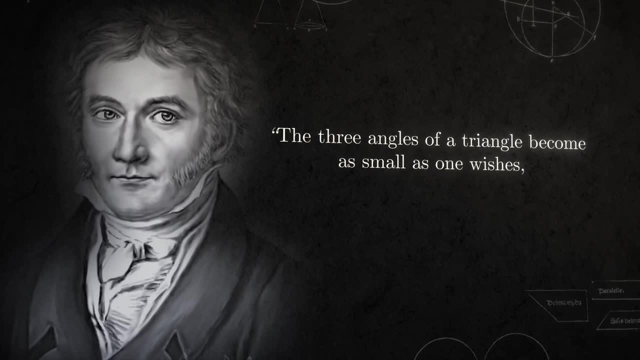 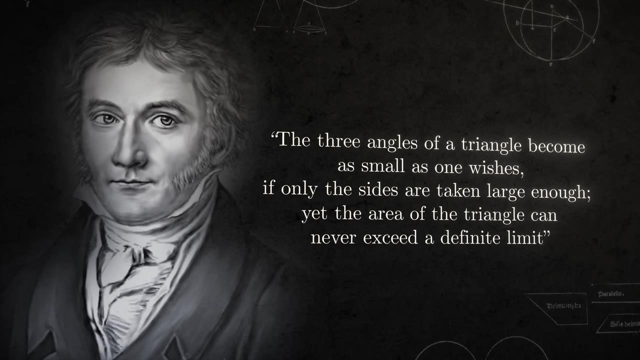 paradoxical and to the uninitiated absurd theorems. For example, Gauss writes: The three angles of a triangle become as small as one wishes, if only the sides are taken large enough. Yet the area of the triangle can never exceed a definite limit. In other words, you can. 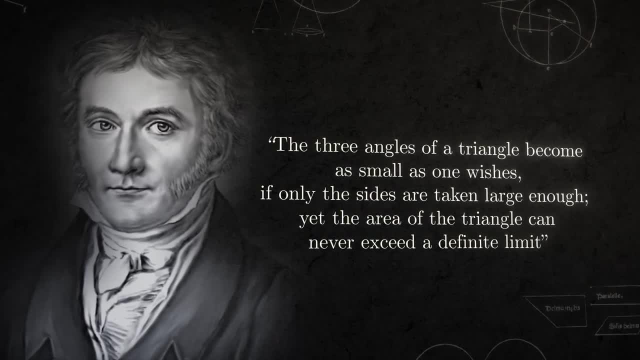 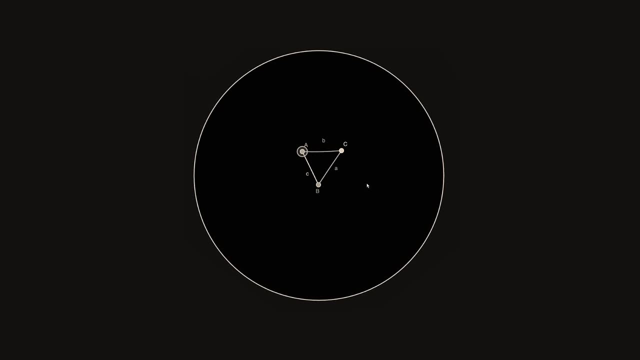 have a triangle that's infinitely long, but the area is finite. You can see why by using the Poincaré disk model. A small triangle looks pretty ordinary, but as you make it bigger, the angles start to become smaller. Eventually all those angles go to zero, because all these lines intersect the disk at 90 degrees. 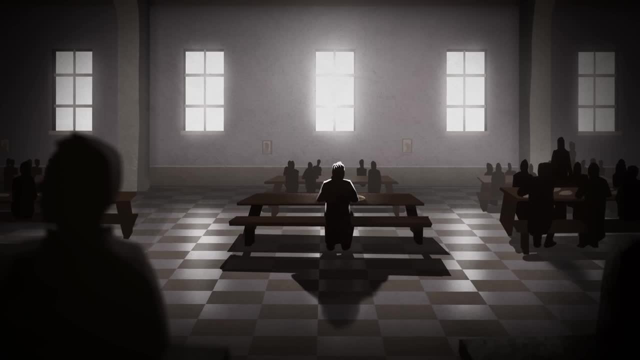 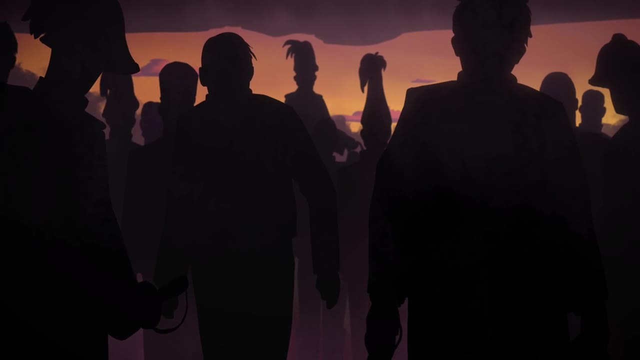 Baliai grew arrogant and found it difficult to accept authority from his superiors. That made him hard to get along with. This reached a peak when, during one of his deployments, 13 cavalry officers from his garrison challenged him to a duel. 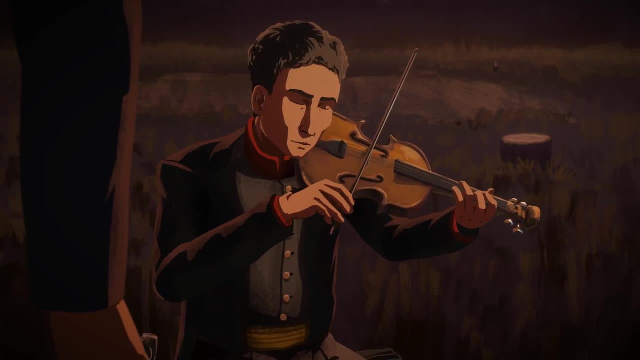 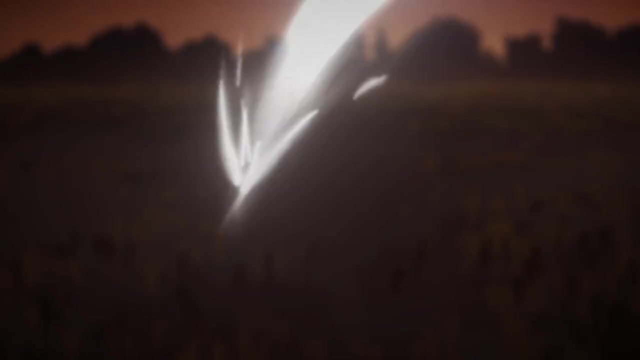 Baliai accepted their challenge on the condition that after every two duels, he could play for a little while on his violin. Baliai fought each of them in succession, winning all 13 duels and leaving behind all his adversaries on the square. While Baliai loved dueling, his first love was still mathematics. In 1832, nine years after he discovered his strange new universe, he published his findings as a 24-page appendix to his father's textbook, Extremely proud and excited about his son's work. 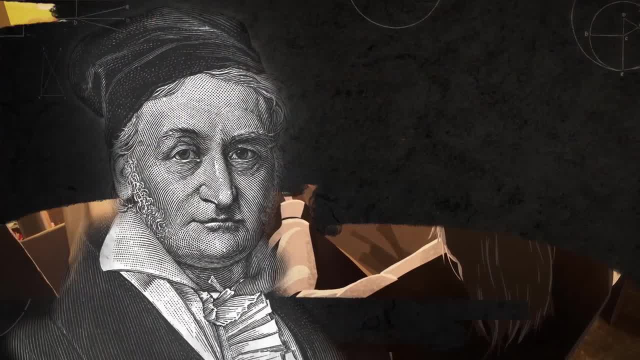 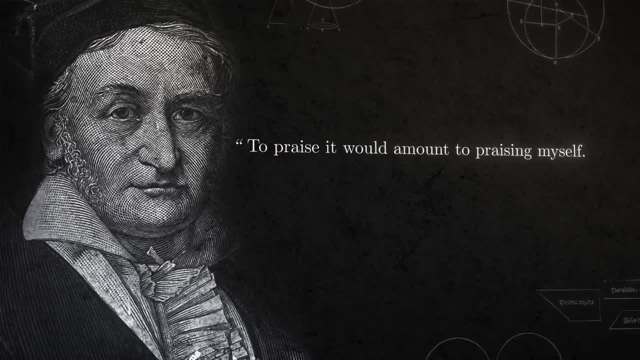 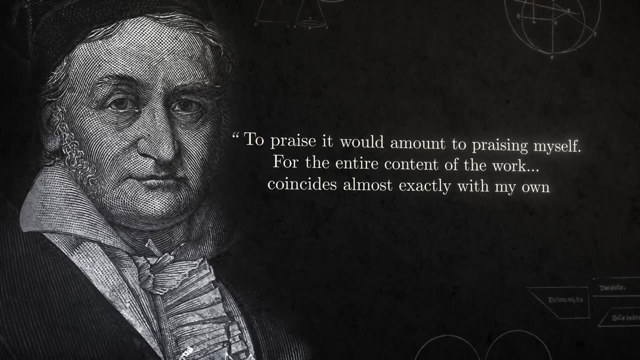 Farkas Baliai sent it to perhaps the greatest mathematician of all time, Carl Friedrich Gauss. After careful examination, Gauss replied a few months later. To praise it would amount to praising myself, for the entire content of the work coincides almost exactly with my own meditations. 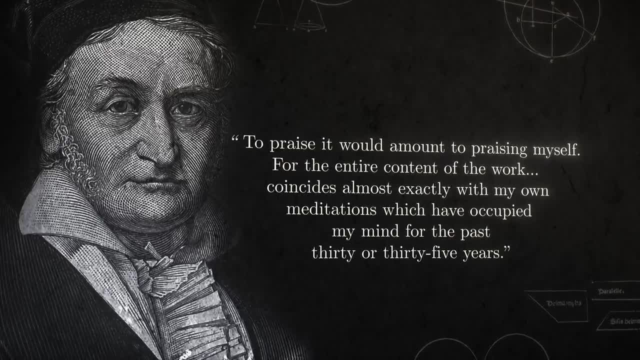 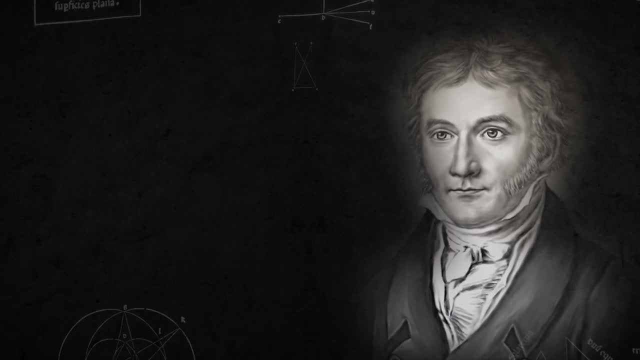 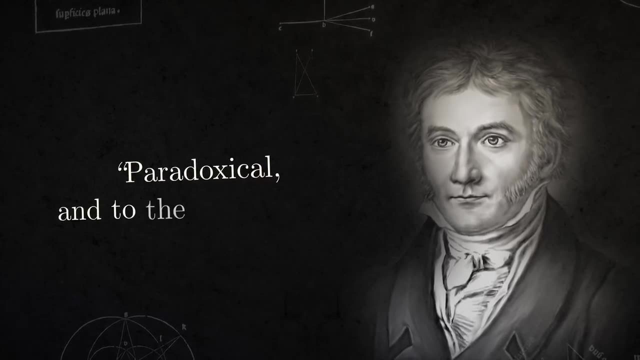 which have occupied my mind for the past 30 or 35 years. Years earlier, Gauss had wandered a similar path. In 1824, he wrote a private letter to one of his friends in which he describes discovering a curious geometry, one with paradoxical and to the uninitiated absurd theorems. 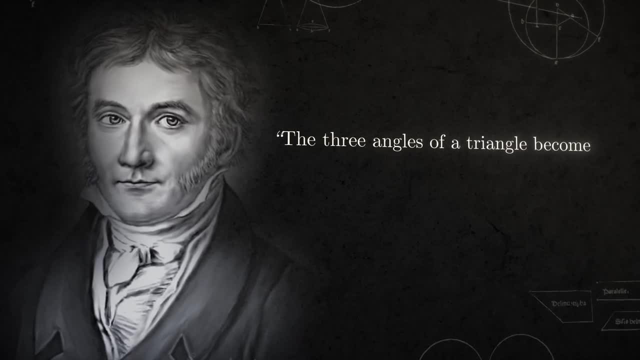 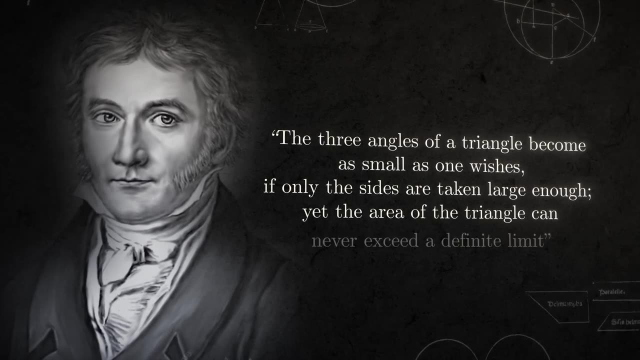 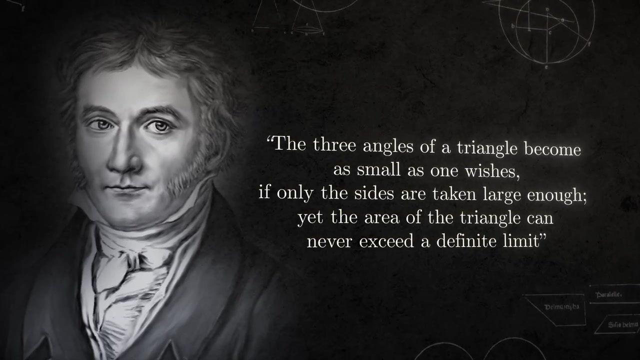 For example, Gauss writes: The three angles of a triangle become as small as one wishes, if only the sides are taken large enough. yet the area of the triangle can never exceed a definite limit. In other words, you can have a triangle that's infinitely long. 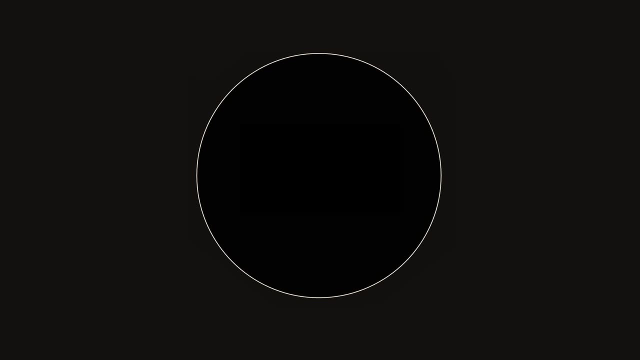 but the area is finite. You can see why by using the Poincaré disk model. A small triangle looks pretty ordinary, but as you make it bigger, the angles start to become smaller and smaller. Eventually, all those angles go to zero. 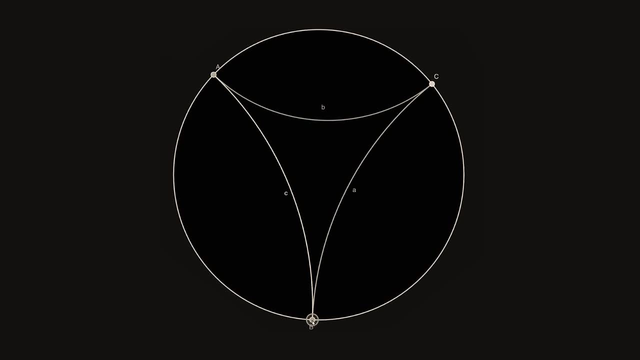 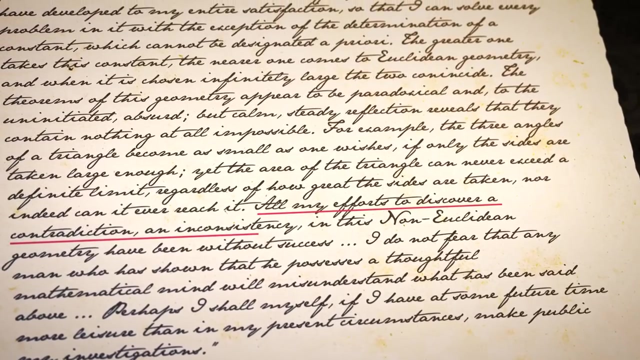 because all these lines intersect the disk at 90 degrees. Now these lines are infinitely long, but because of the geometry the area is finite. In the same private letter, Gauss wrote: All my efforts to discover a contradiction and inconsistency in this non-Euclidean geometry have been without success. 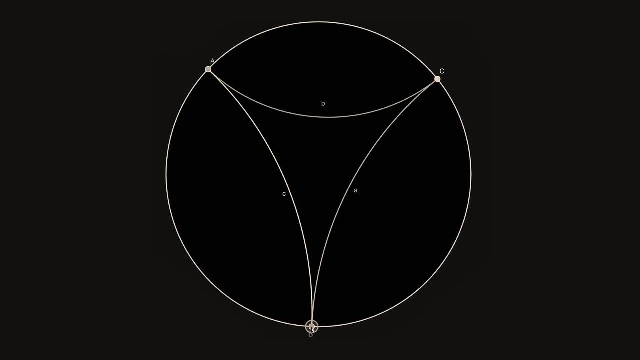 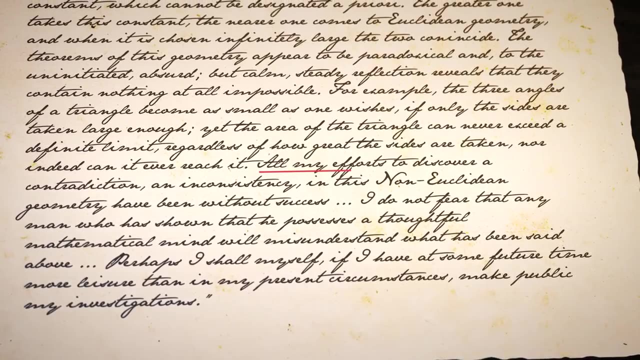 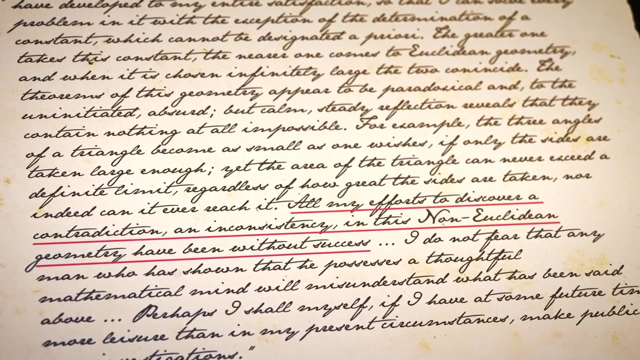 Now these lines are infinitely long, but because of the geometry, the area is finite. In the same private letter, Gauss wrote: All my efforts to discover a contradiction and inconsistency in this non-Euclidean geometry have been without success, Just like Bolyai Gauss had found that this geometry 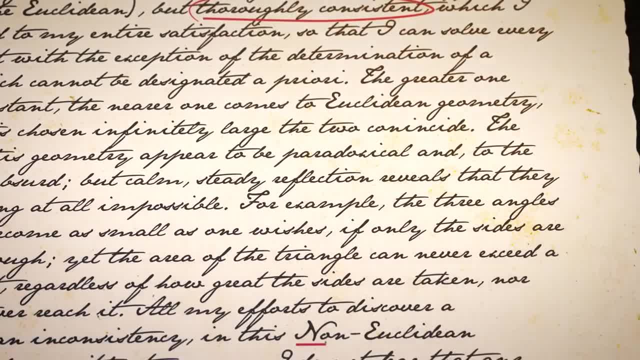 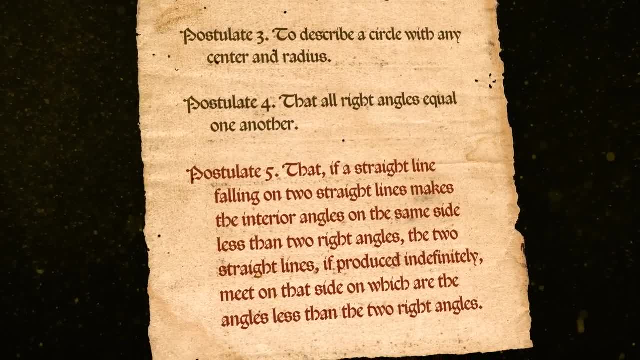 seemed thoroughly consistent. He named it non-Euclidean geometry, a name that stuck. It describes geometries where Euclid's first four postulates hold but the fifth doesn't. But Gauss decided not to publish his findings for fear of ridicule. 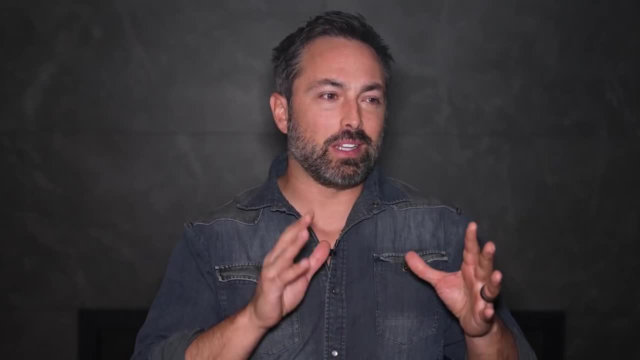 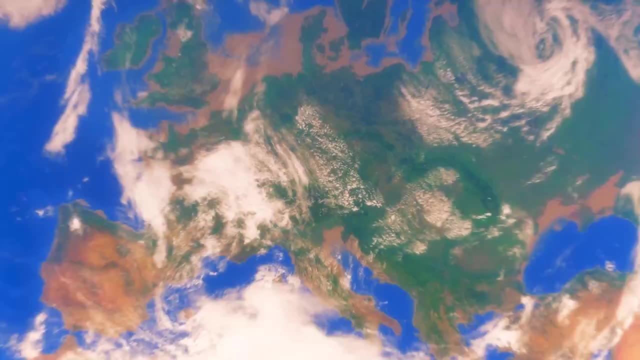 This aversion to a different kind of geometry should at least be a little surprising, because there is one other geometry that we should be very familiar with: spherical geometry, since we all live on a sphere. On a sphere, straight lines are parts of great circles. 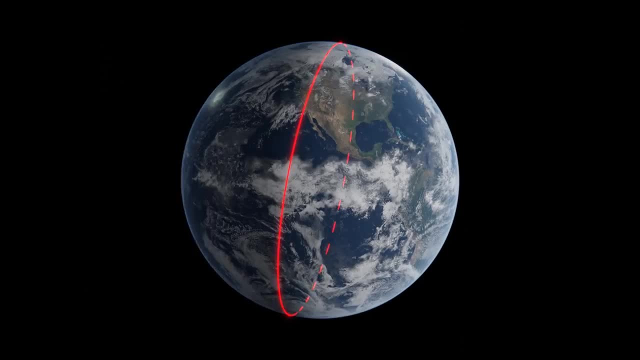 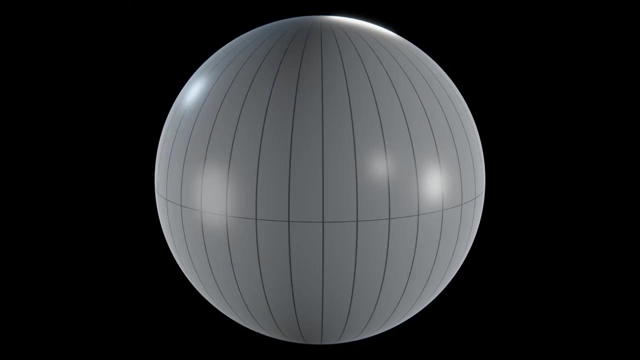 These are the circles with the largest possible circumference On Earth. the equator and circles of longitude are examples of great circles, And we can use this to see how straight lines behave. These lines seem to go in the same direction, but as you keep extending them, 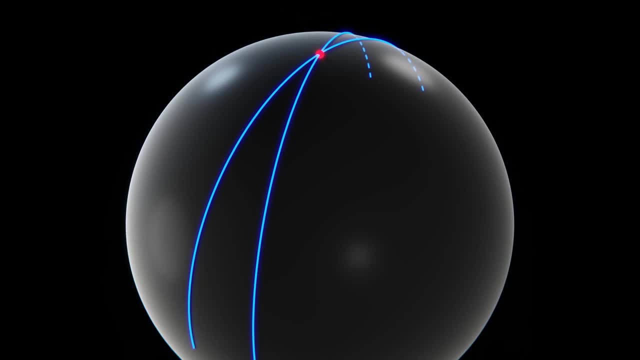 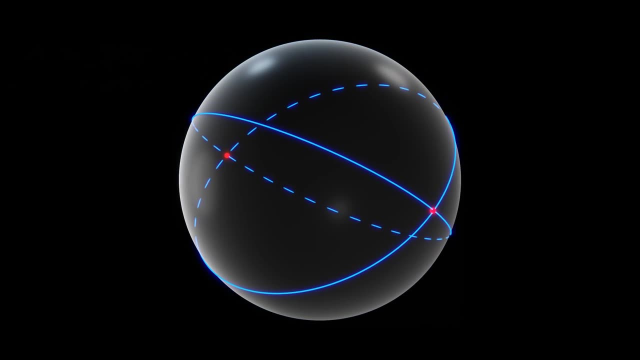 you find that they intersect once and then again on the other side of the Earth, And this will always happen for any two great circles, because they must each have the largest possible circumference. So on a sphere there are no parallel lines. 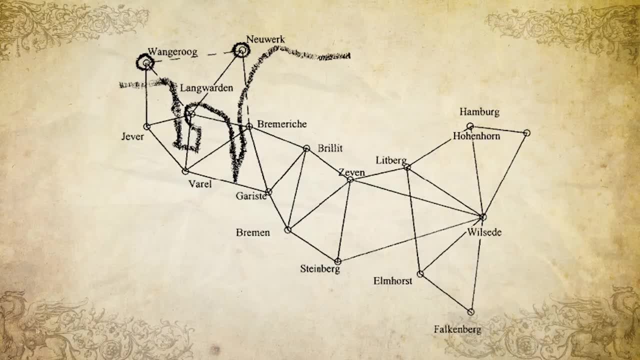 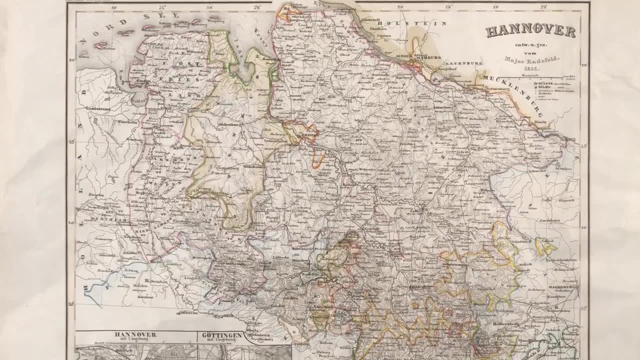 Gauss had long been fascinated by spherical geometry. He was also a geodesist and frequently took measurements of the Earth. In the 1820s, he was tasked with surveying the Kingdom of Hanover to help make a map. As part of this survey, he climbed the mountains near Göttingen. 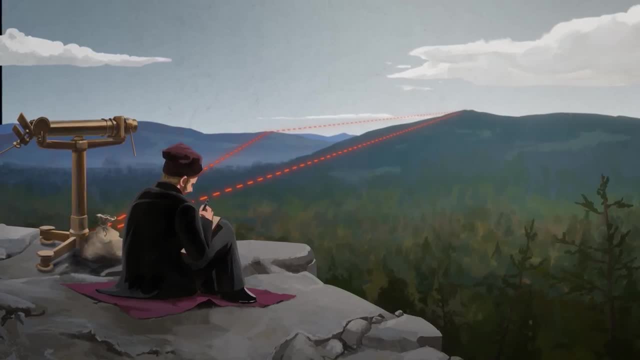 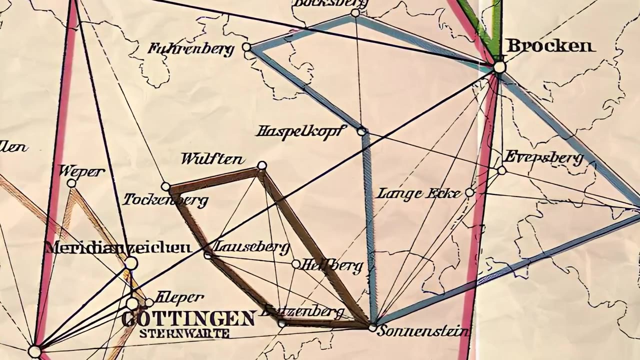 With the help of people situated on other landmarks, they were able to carefully measure the angles of several triangles, Which would then be used to determine the position of one place relative to another As a reference for the survey and to help determine the roundness of the Earth. 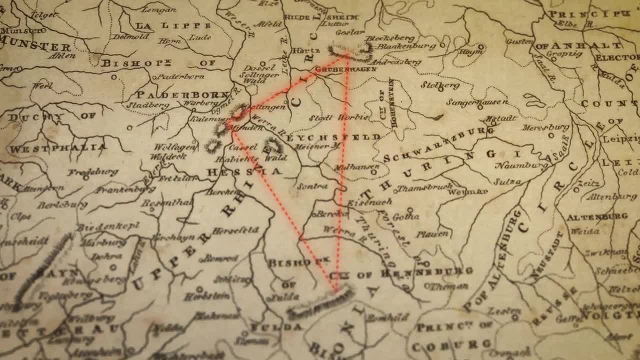 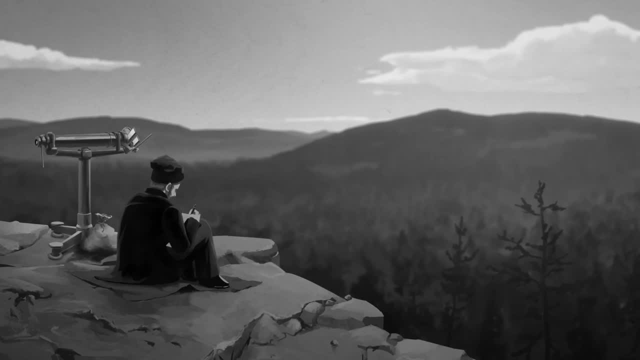 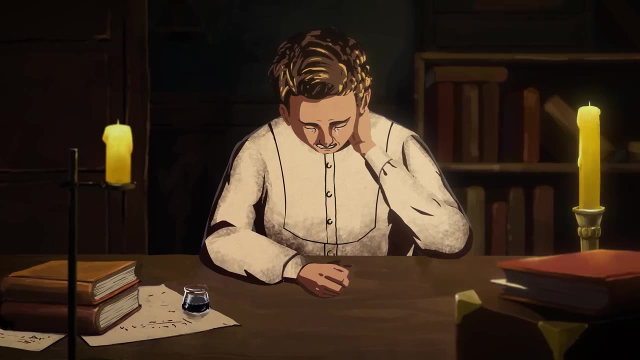 they also precisely measured the angles of a large triangle formed by three mountains. But for all of Gauss's romantic notions of taking measurements on top of mountains, he was not the kindest correspondent. When Bolyai received his hero's response, he was devastated. 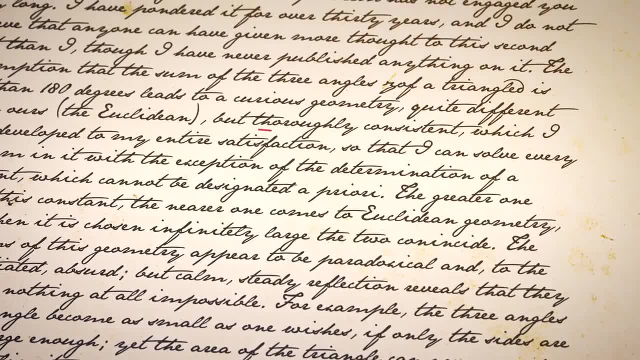 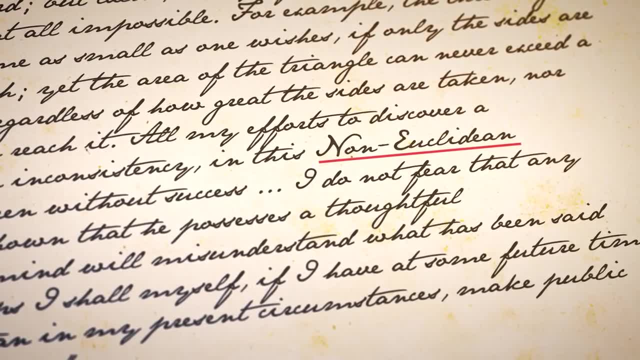 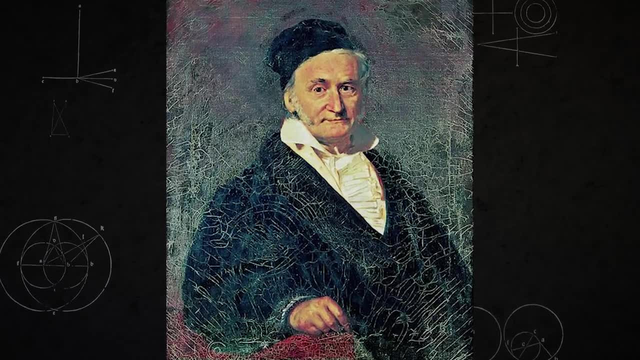 Just like Bolyai, Gauss had found that this geometry seemed thoroughly consistent, He named it non-Euclidean geometry, a name that stuck. It describes geometries where Euclid's first four postulates hold but the fifth doesn't. But Gauss decided not to publish his findings for fear of ridicule. 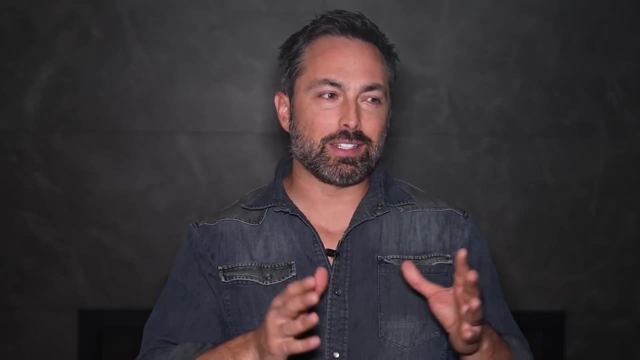 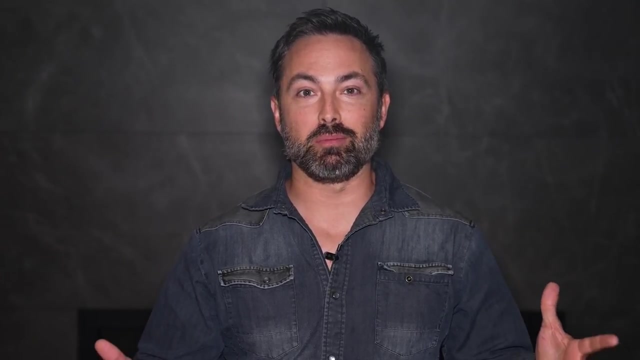 This aversion to a different kind of geometry should at least be a little surprising, because there is one other geometry that we should be very familiar with: spherical geometry, since we all live on a sphere. On a sphere, straight lines are parts of great circles. 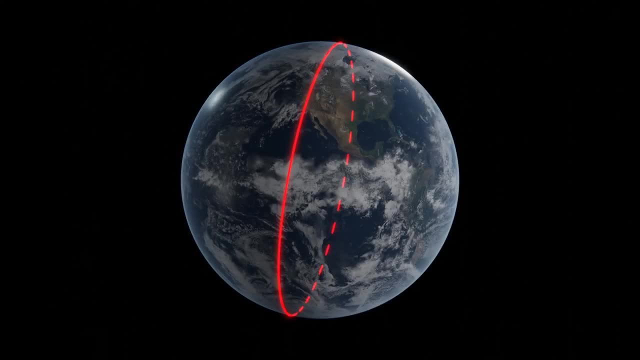 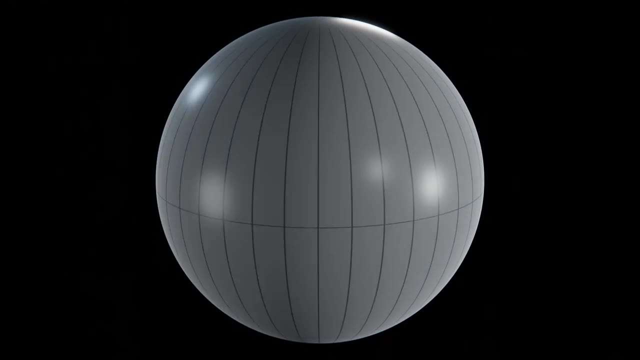 These are the circles with the largest possible circumference On Earth. the equator and circles of longitude are examples of great circles, And we can use this to see how straight lines behave. These lines seem to go in the same direction, but as you keep extending them, 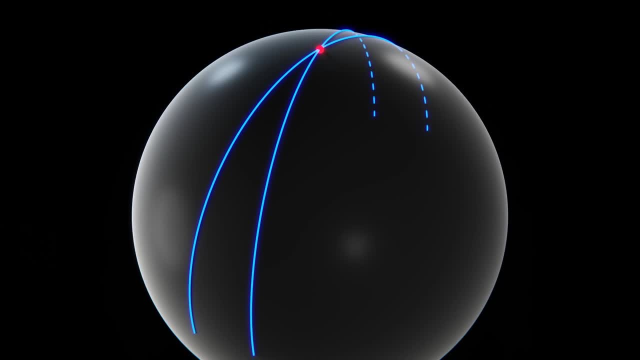 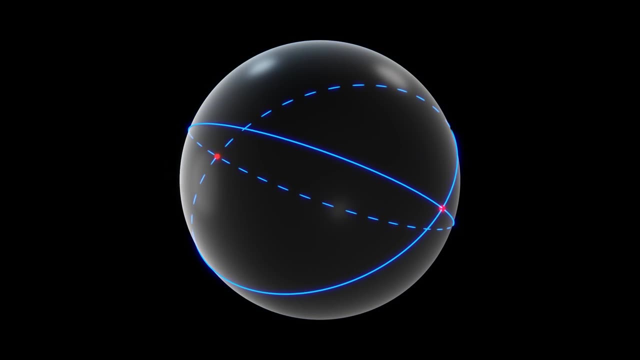 you find that they intersect once and then again on the other side of the Earth, And this will always happen for any two great circles, because they must each have the largest possible circumference. So on a sphere there are no parallel lines. 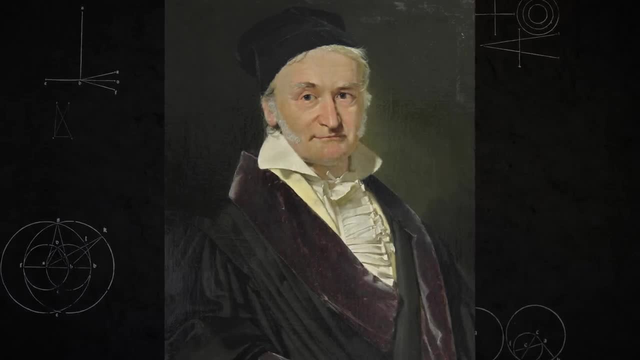 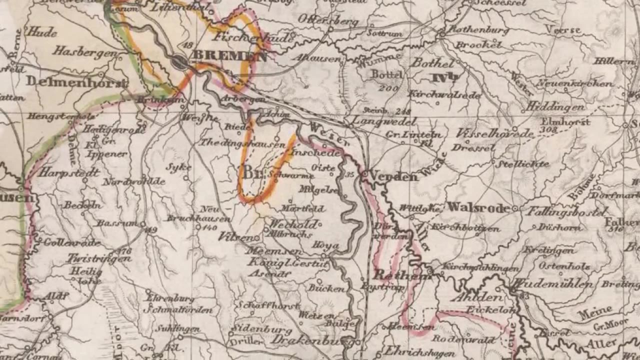 Gauss had long been fascinated by spherical geometry. He was also a geodesist and frequently took measurements of the Earth. In the 1820s he was tasked with surveying the kingdom of Hanover to help make a map. As part of this survey, he climbed the mountains near Göttingen. 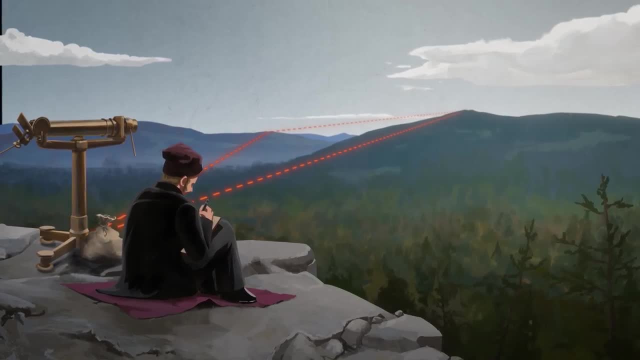 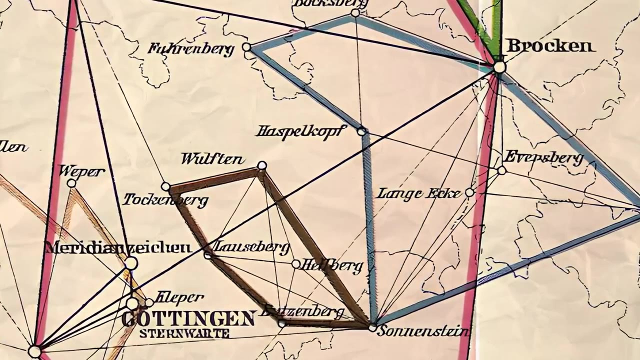 With the help of people situated on other landmarks, they were able to carefully measure the angles of several triangles, which would then be used to determine the position of one place relative to another As a reference for the survey and to help determine the roundness of the Earth. 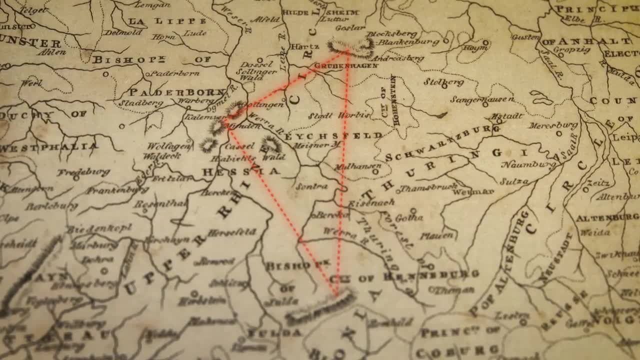 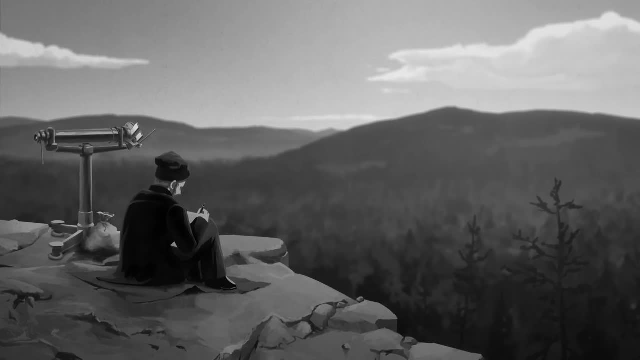 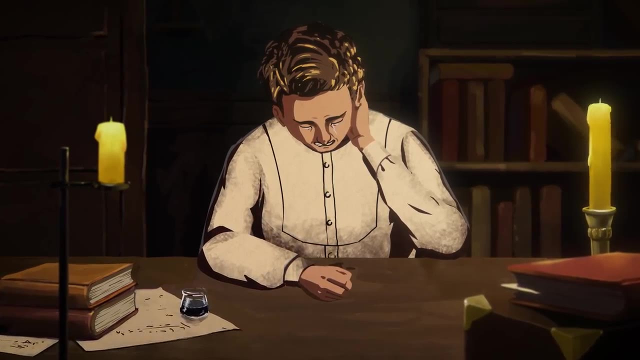 they also precisely measured the angles of a large triangle formed by three mountains. But for all of Gauss's romantic notions of taking measurements on top of mountains, he was not the kindest correspondent. When Bolyai received his hero's response, he was devastated. 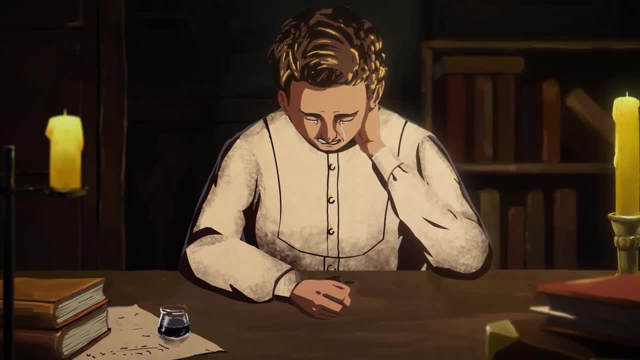 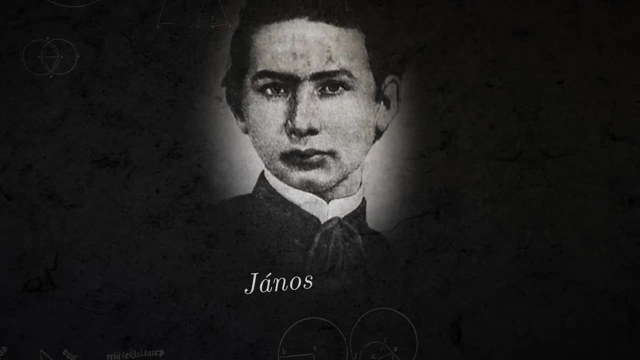 believing that Gauss was trying to undermine him and steal his ideas. He was so embittered by Gauss's response that he never published again In 1848,. Bolyai had to endure another hardship when he found out that Russian mathematician Nikolai Lobachevsky 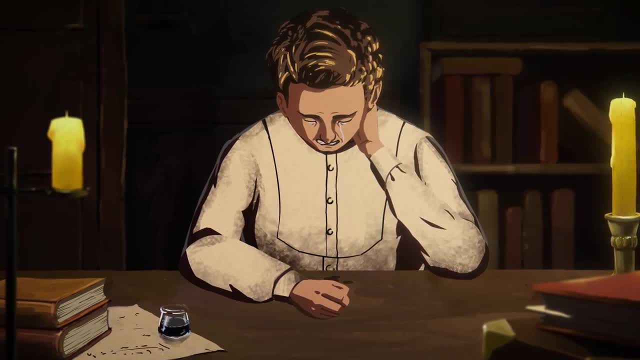 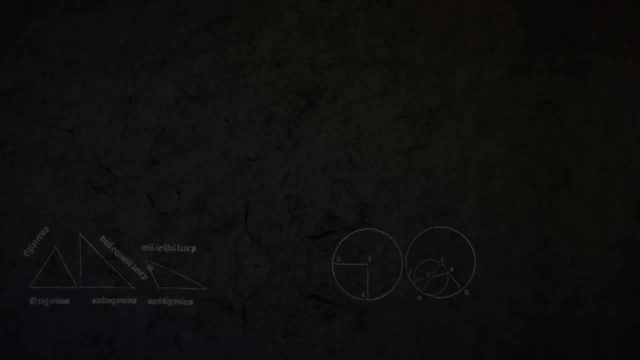 Believing that Gauss was trying to undermine his own vision, trying to undermine him and steal his ideas. He was so embittered by Gauss's response that he never published again. In 1848, Bolyai had to endure another hardship when he found out that Russian mathematician 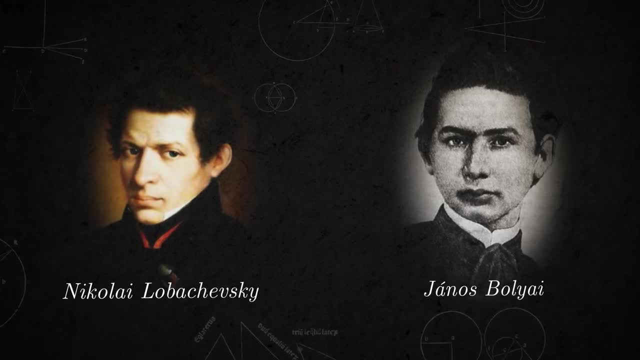 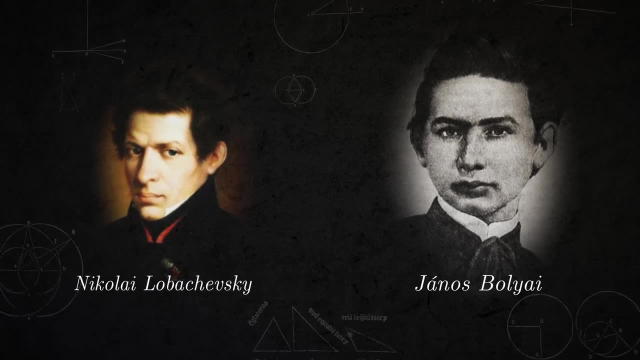 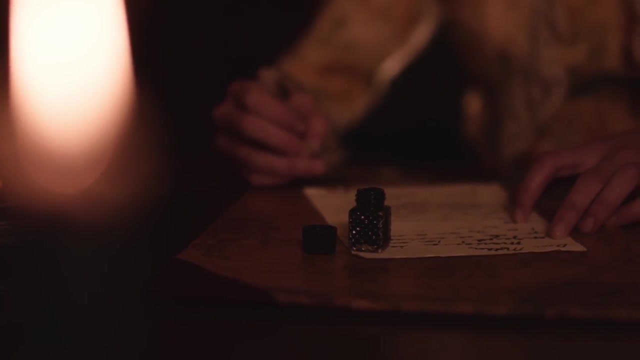 Nikolai Lobachevsky had independently discovered non-Euclidean geometry several years before Bolyai had published his 24-page long appendix. When Bolyai died in 1860, he left behind 20,000 pages of published mathematical manuscripts. 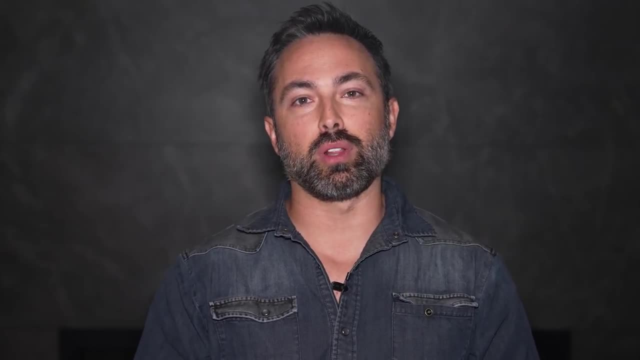 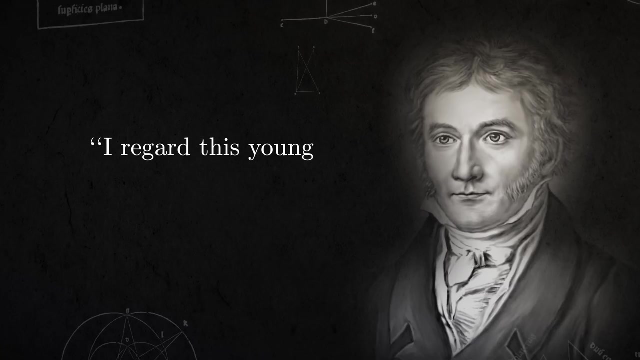 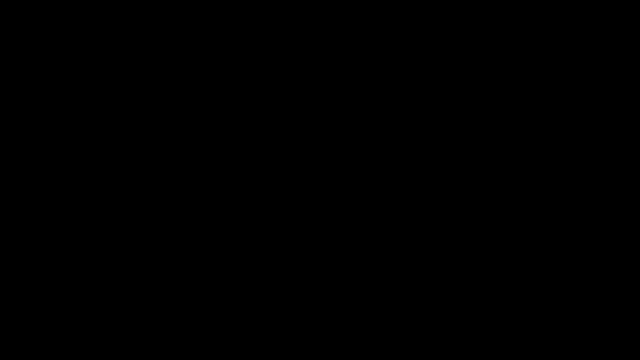 He would not know that Gauss did independently discover non-Euclidean geometry. nor would he know that, upon receiving the appendix, Gauss had written to a friend. I regard this young geometer, Bolyai, as a genius of the first order. While Bolyai was embittered, non-Euclidean geometries continued to develop. 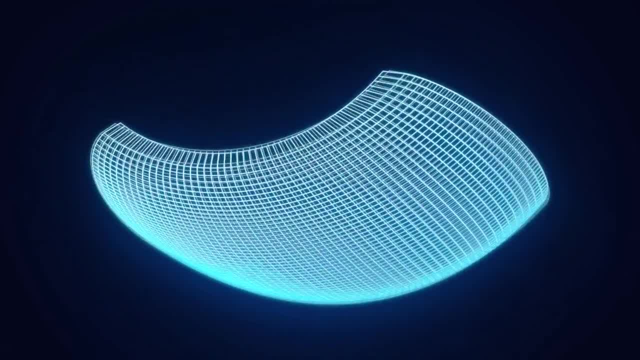 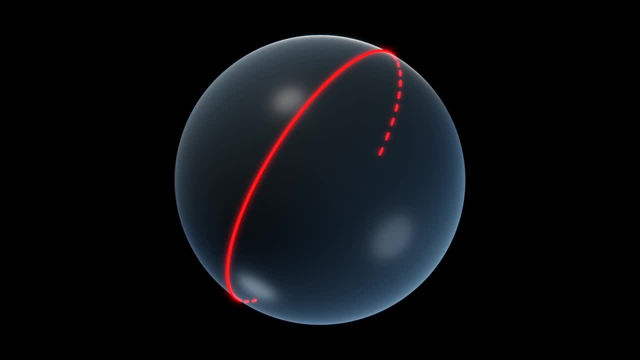 Until 1854, spherical geometry wasn't actually considered a non-Euclidean. The first postulate was that. the second postulate was not a non-Euclidean geometry. That's because on a sphere, lines can't be extended indefinitely. This is what earlier mathematicians had stumbled upon and therefore dismissed this geometry. 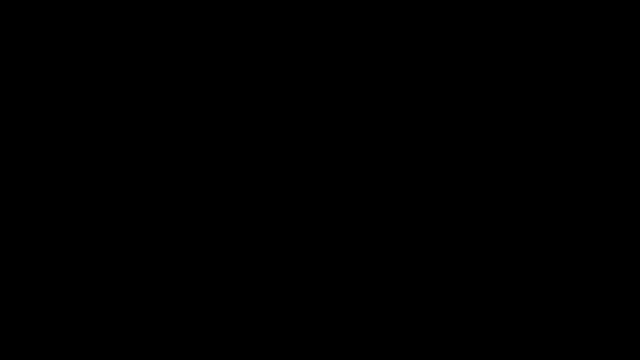 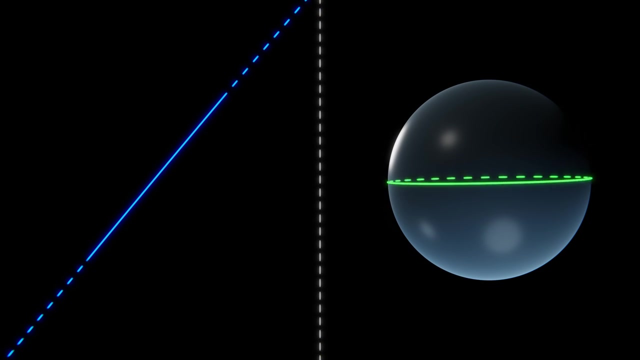 since Euclid's second postulate wouldn't hold. But in 1854, Riemann changed the second postulate from an infinite extension to something that is- quote unbounded, so that the second postulate still holds on a sphere With this change. 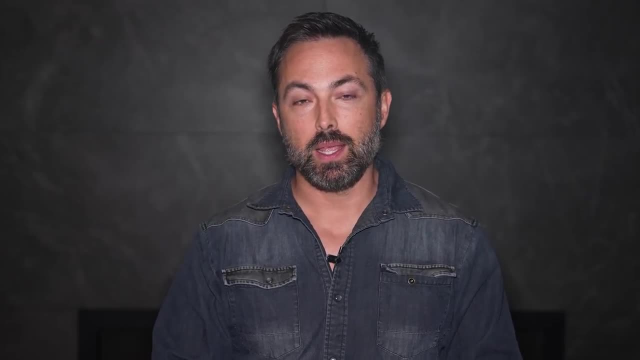 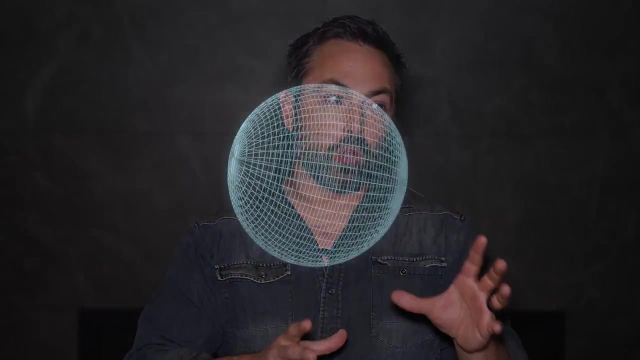 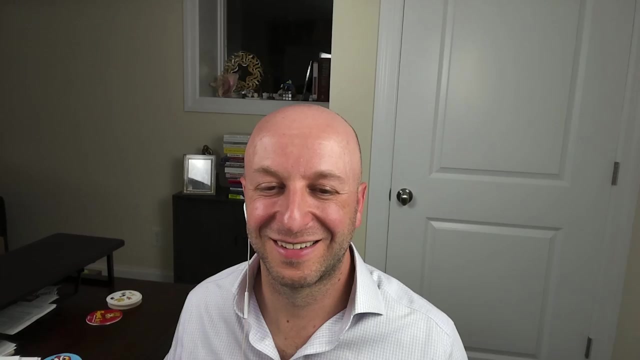 non-Euclidean geometry became another valid non-Euclidean geometry. By using the generalized four postulates and taking the fifth as there being no parallel lines, you could now derive spherical or elliptic geometry. Would you consider the fifth postulate a mistake? 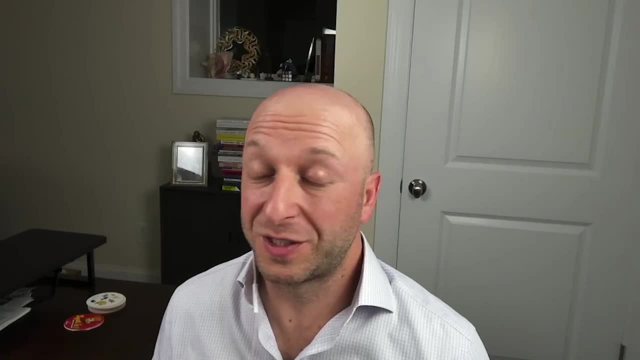 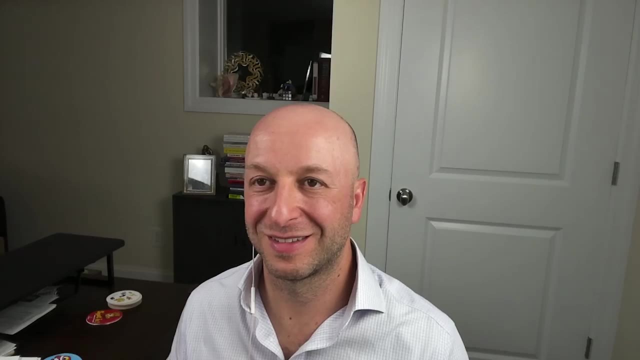 Would it have been better if he just never wrote that down? If he never wrote that down, he would have stunted his geometry because he wouldn't be able to prove a lot of the things that he claimed to have. It's beautiful that he wrote this. 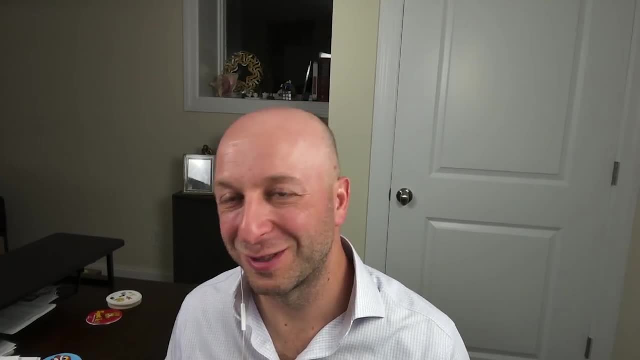 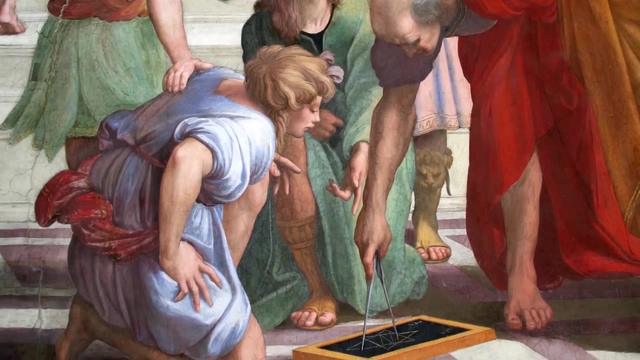 It's beautiful that people spent 2000 years trying to refute him, only to discover that, in fact, he was right in writing this in the first place. So while Euclid was right to write down the fifth postulate, he did make a different mistake. 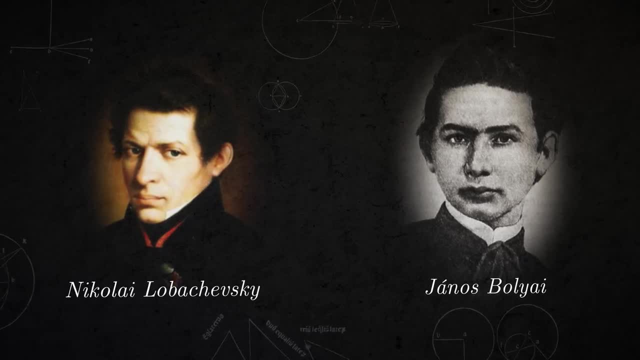 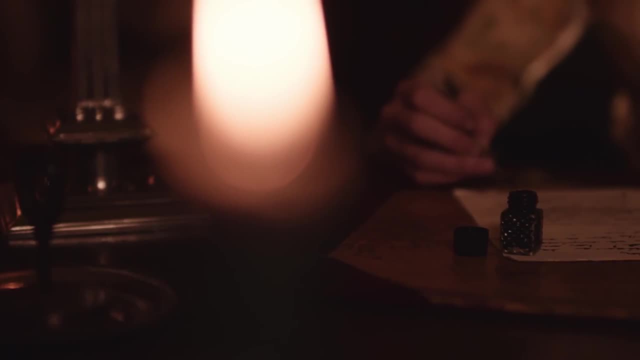 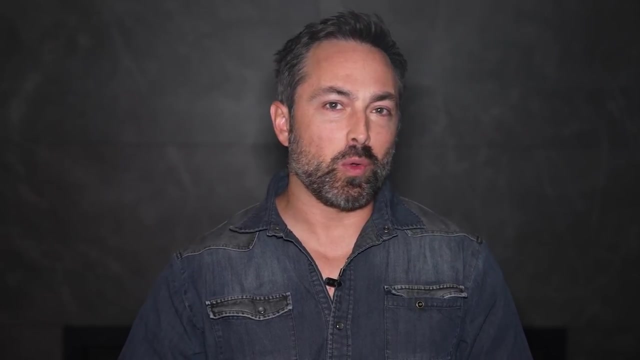 had independently discovered non-Euclidean geometry several years before Bolyai had published his 24-page long appendix. When Bolyai died in 1860, he left behind 20,000 pages of unpublished mathematical manuscripts. He would not know that Gauss did independently discover non-Euclidean geometry. 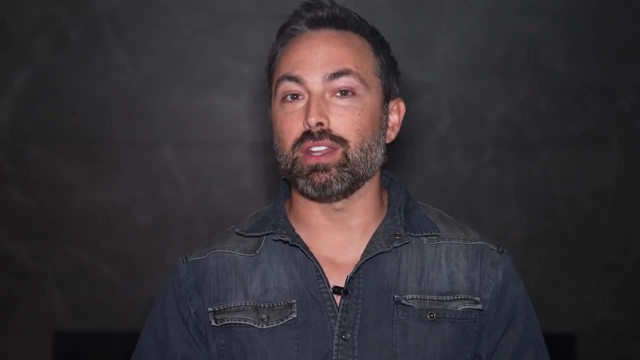 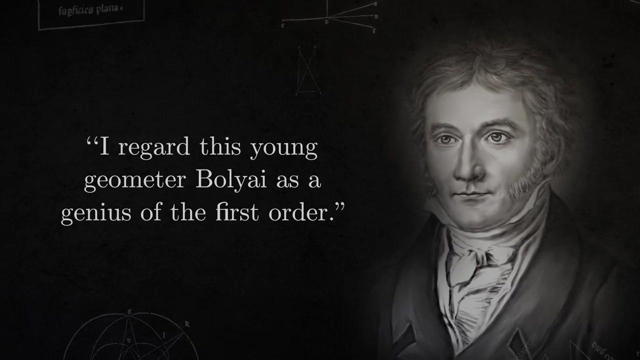 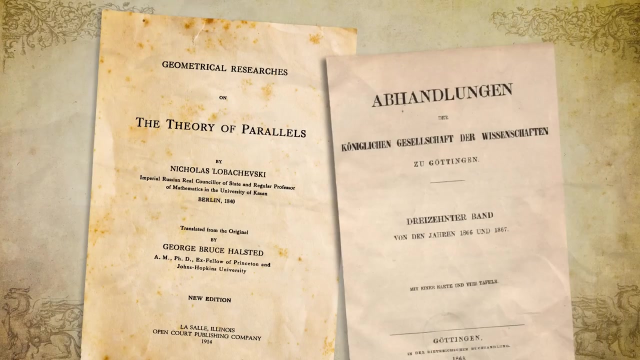 nor would he know that, upon receiving the appendix, Gauss had written to a friend. I regard this young geometer, Bolyai, as a genius of the first order. While Bolyai was embittered, non-Euclidean geometries continued to develop. 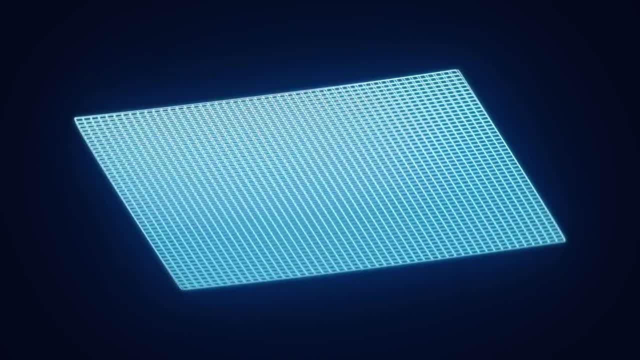 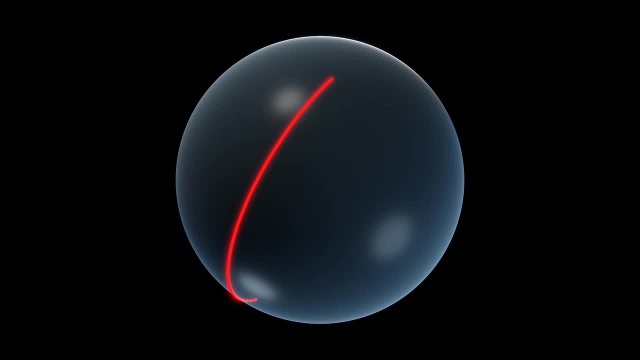 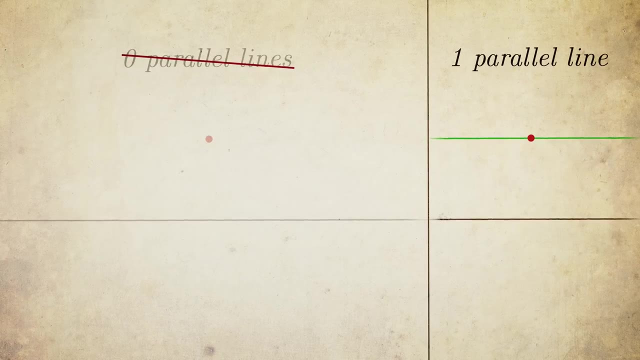 Until 1854, spherical geometry wasn't actually considered a non-Euclidean geometry. That's because on a sphere, lines can't be extended indefinitely. This is what earlier mathematicians had stumbled upon and therefore dismissed this geometry, since Euclid's second postulate wouldn't hold. 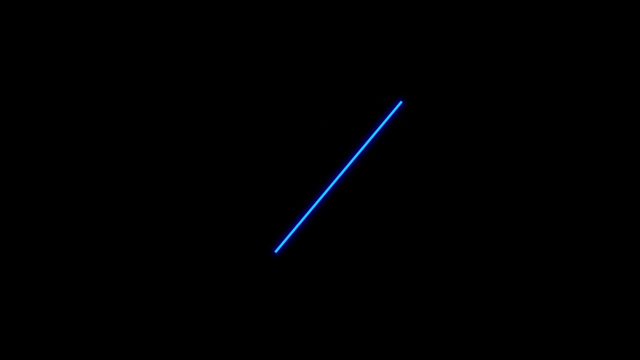 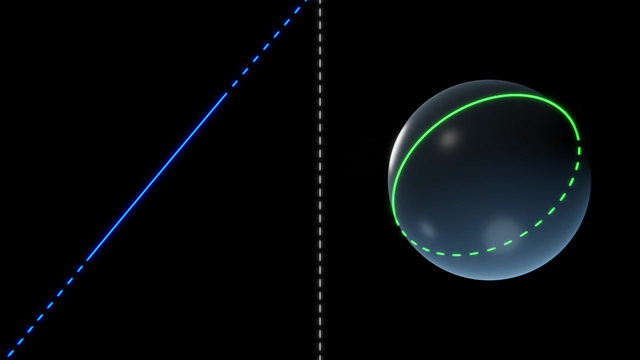 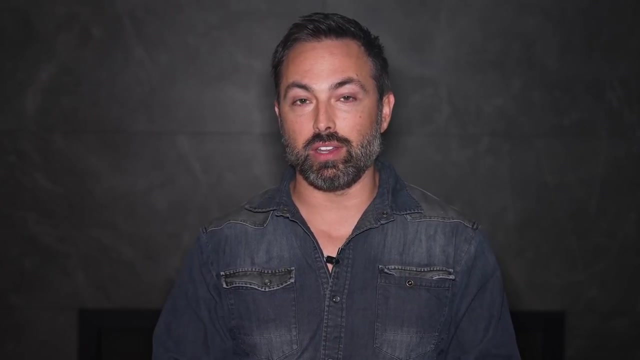 But in 1854, Riemann changed the second postulate from an infinite extension to something that is- quote- unbounded, so that the second postulate still holds on a sphere. With this change, spherical geometry became another valid non-Euclidean geometry. 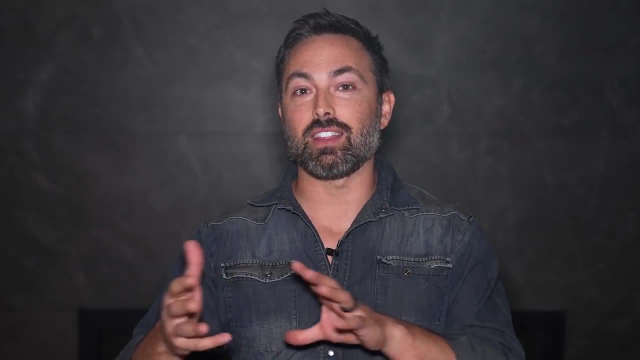 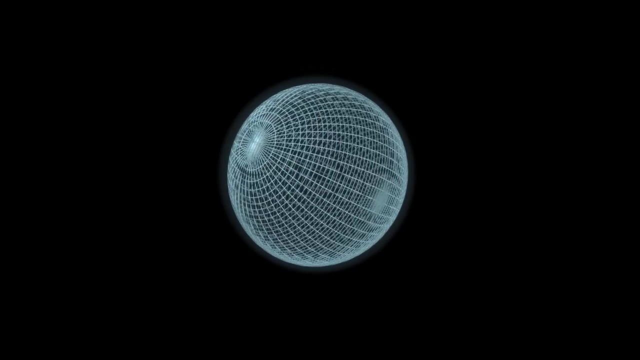 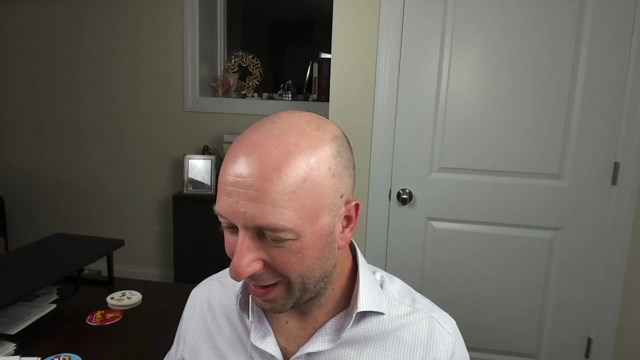 By using the generalized four postulates and taking the fifth as there being no parallel lines, you could now derive spherical or elliptic geometry. Would you consider the fifth postulate a mistake? Would it have been better if he just never wrote that down? 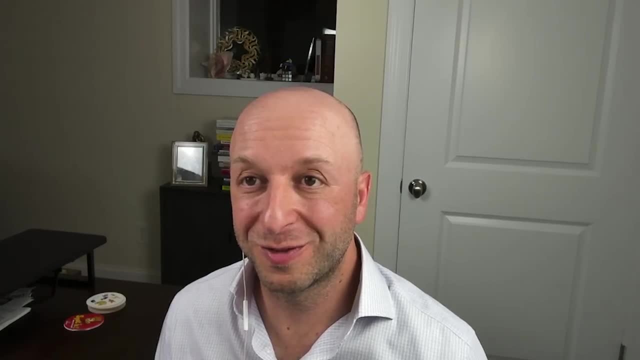 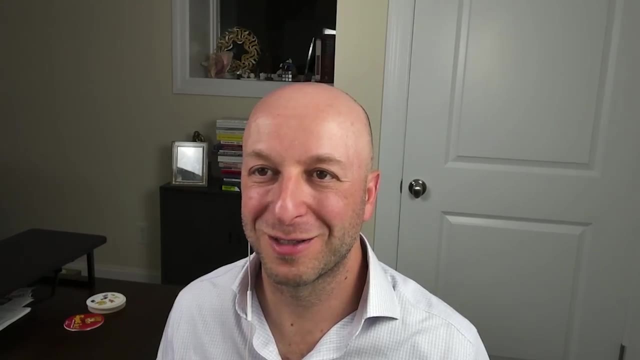 If he never wrote that down, he would have stunted his geometry because he wouldn't be able to prove a lot of the things that he claimed to have. It's beautiful that he wrote this. It's beautiful that people spent 2,000 years trying to refute him. 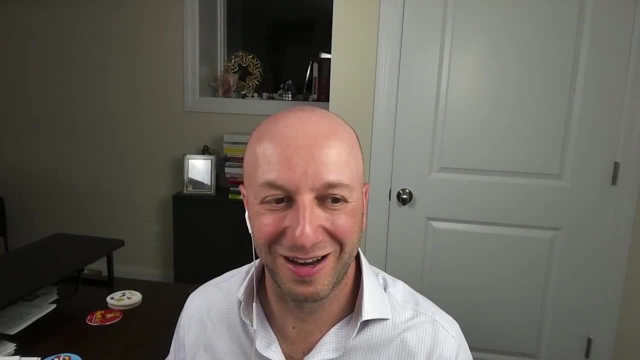 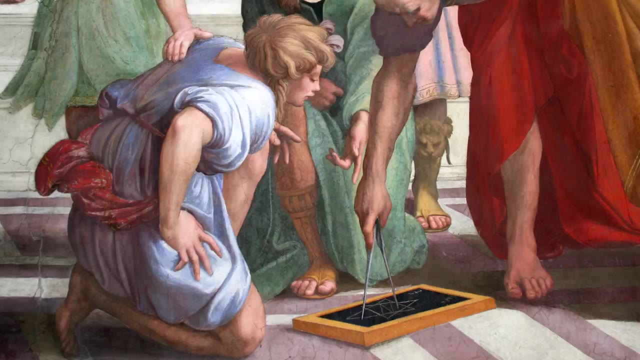 only to discover that, in fact, he was right In writing this in the first place. So while Euclid was right to write down the fifth postulate, he did make a different mistake. So here's the problem with what Euclid was doing. 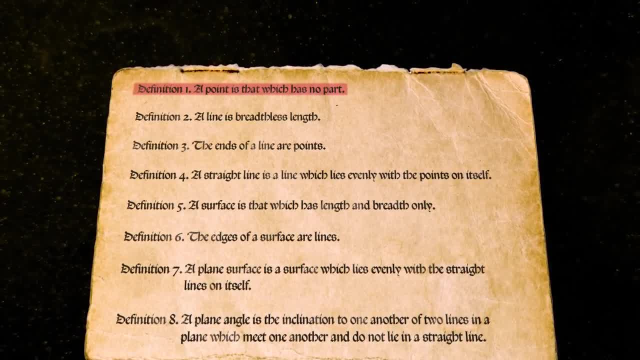 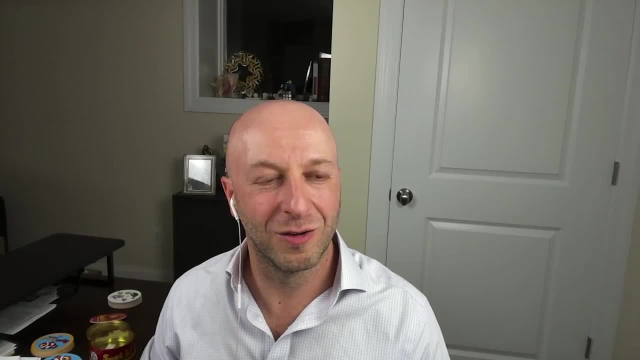 Definition. one A point is that which has no part. What does it mean to have a part? What is a part? What does it mean not to have a part? A line is a breathless length. What does it mean to have breath? 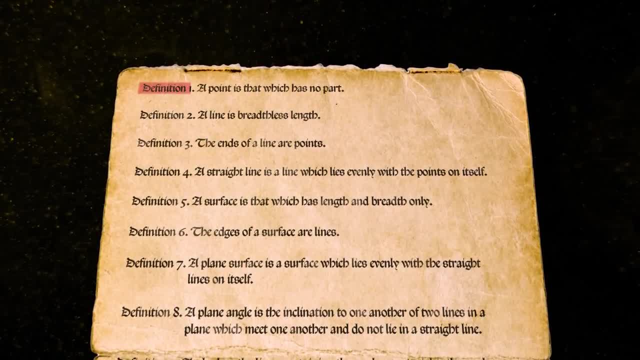 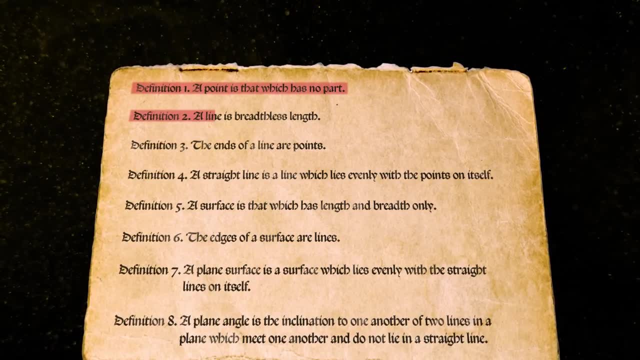 So here's the problem with what Euclid was doing. Definition: one A point is that which has no part. What does it mean to have a part? What is a part? What does it mean not to have a part? A line is a breathless length. 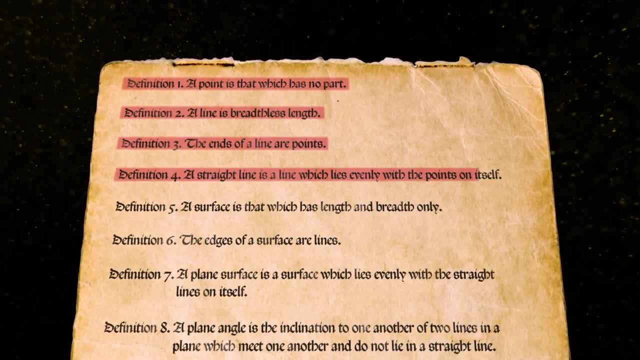 What does it mean? to have breath Lying evenly within itself, Within the points in itself? What the hell is he talking about? We read this two minutes ago and we were nodding along like yeah, it completely makes sense what he's saying. 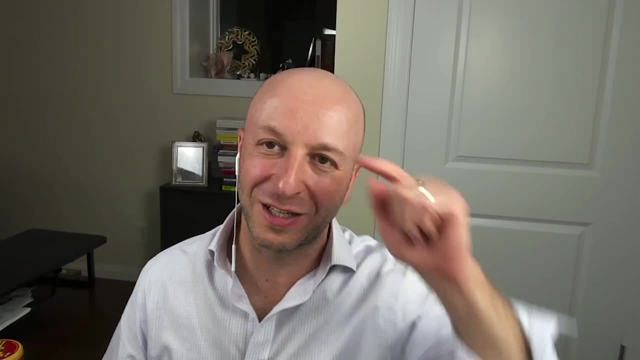 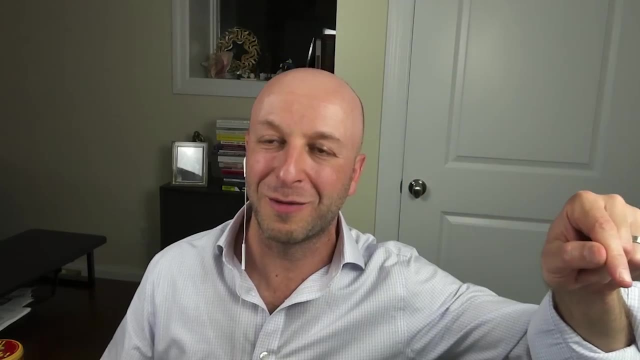 It's all nonsense. Don't give me a definition. that's going to have an infinite recursion. If you give me a definition in terms of other things, then you have to tell me what those things are. If you tell me what that is, you have to tell me what the thing before it is. 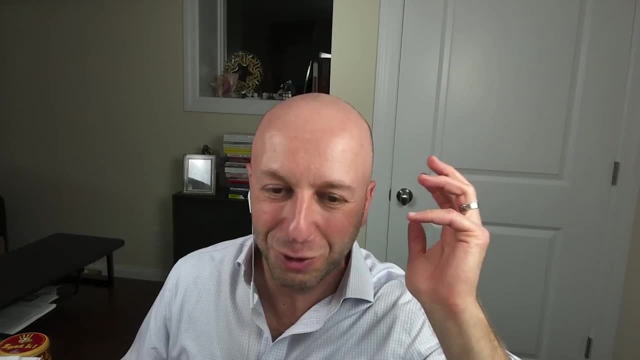 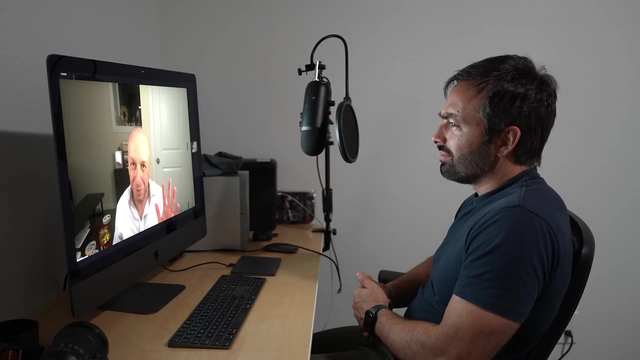 Are the definitions a bad idea? You shouldn't have definitions. You should have undefined terms. I'm not going to tell you what a point is. I'm not going to tell you what a line is. I'm not going to tell you what a plane is. 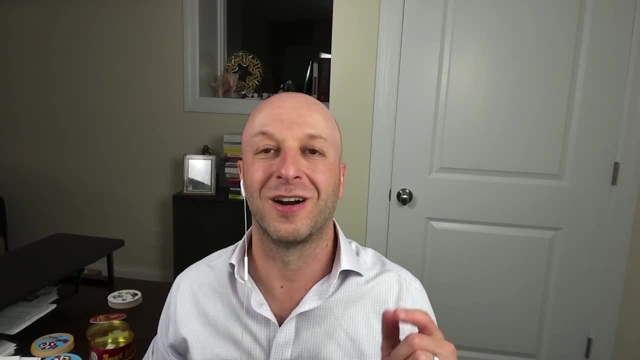 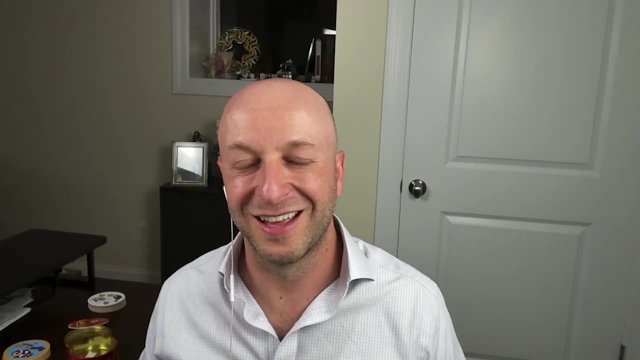 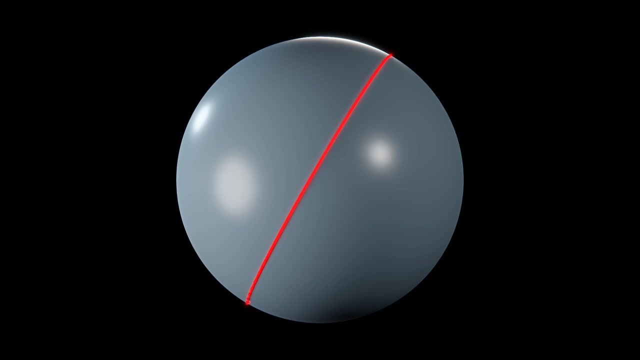 All I'm going to tell you is what the postulates are that they're assumed to satisfy. It's the relationships between the objects that's important, not the definitions of the objects themselves. And once you free your mind to that possibility, all of a sudden you realize that there is a perfectly good geometric world. 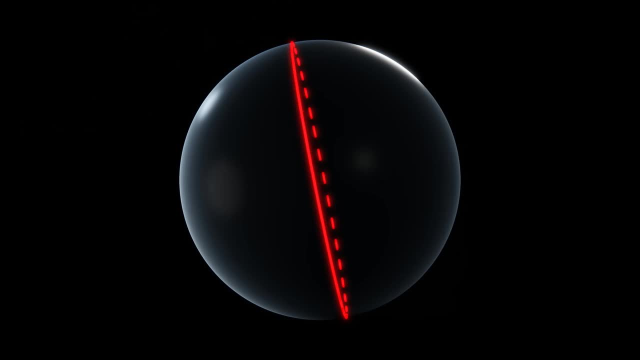 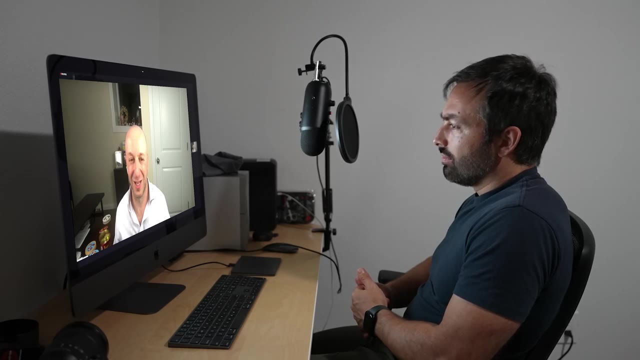 in which by line you mean great circle and by plane you mean sphere, and by point you mean a point on a sphere, and then four of those axioms are satisfied, Just not this one. The fifth, And similarly, there's another model. 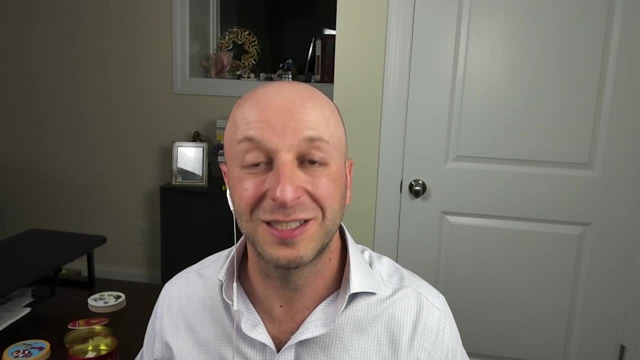 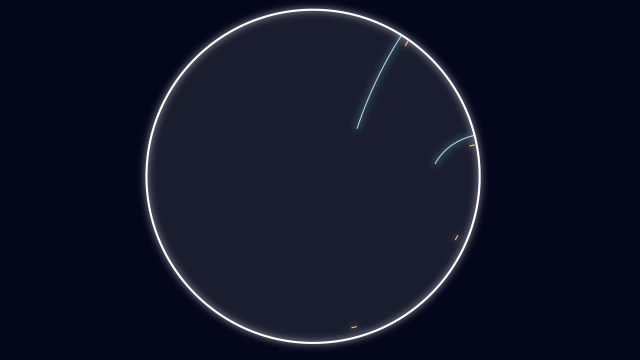 something called the disc model for hyperbolic space, which the disc is the plane. What I mean by straight lines is arcs of circles that are orthogonal to the disc, and then points are points inside the disc, and the disc is the plane. 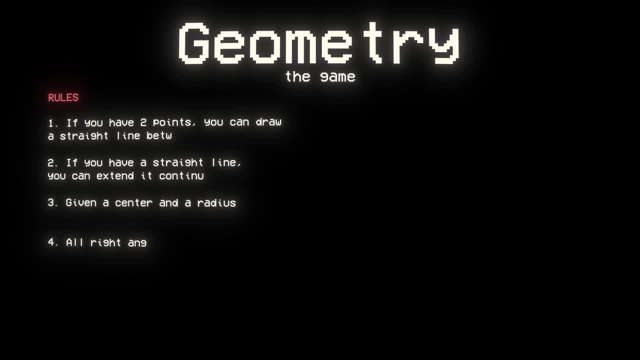 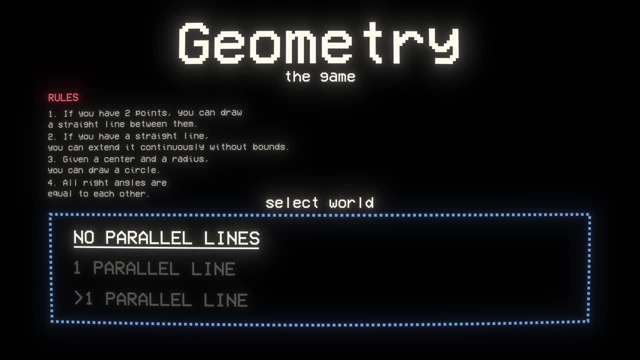 See, you can think of geometry as a game. The first four postulates are like the minimum rules required to play that game, and then the fifth postulate selects the world that you'll play in. If you pick that there are no parallel lines, you're playing in spherical geometry. 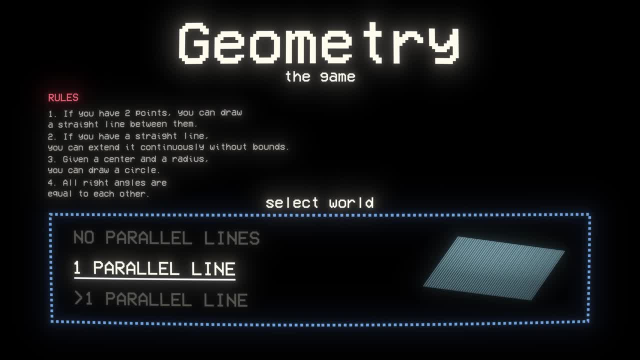 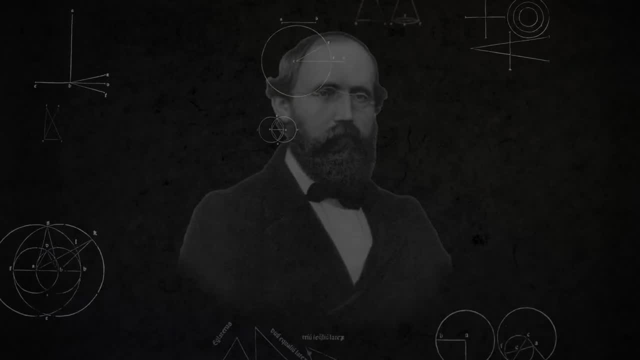 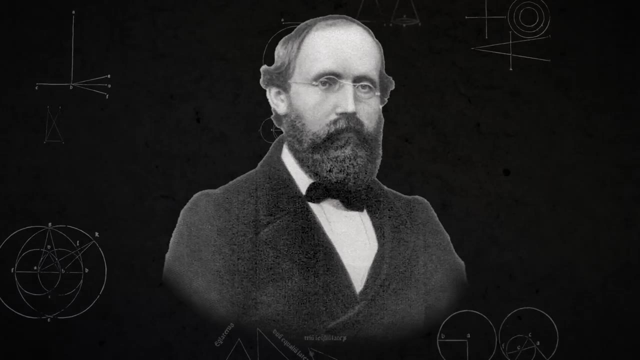 If you choose one parallel line, you're playing in flat geometry, And if you go for more than one parallel line, then you're playing in hyperbolic geometry. But Riemann decided to take it one step further. Instead of selecting just one world to play in, why not combine them all into one? 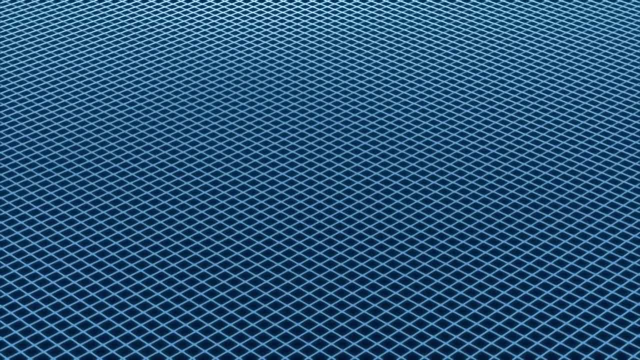 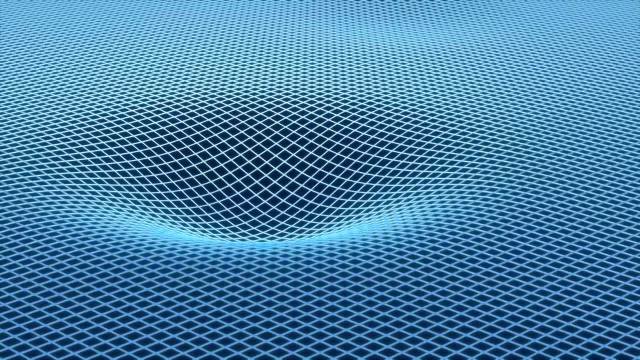 During his inaugural speech in 1854,, he laid out the groundwork for a geometry where the curvature could differ from place to place. One part might be flat, another part might be slightly curved and yet another part might have a very strong curvature. 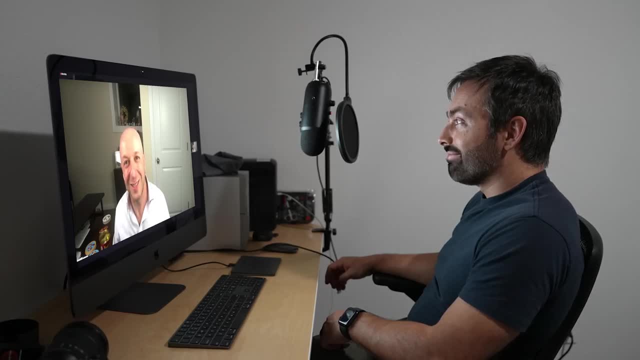 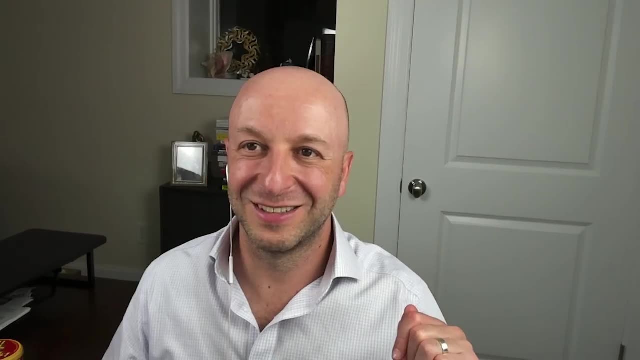 Lying evenly within itself, within the points in itself. What the hell is he talking about? It was just two minutes ago and we were nodding along like, yeah, it completely makes sense what he's saying. It's all nonsense. Don't give me a definition. that's going to have an infinite recursion. 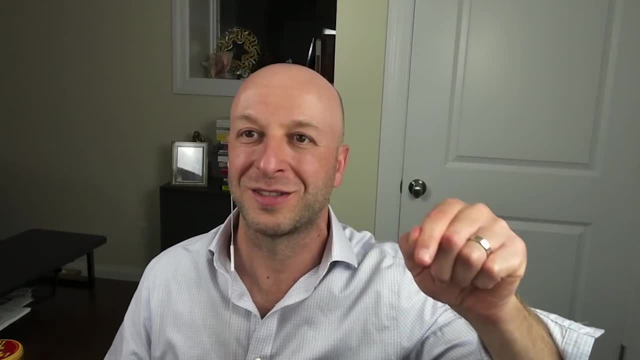 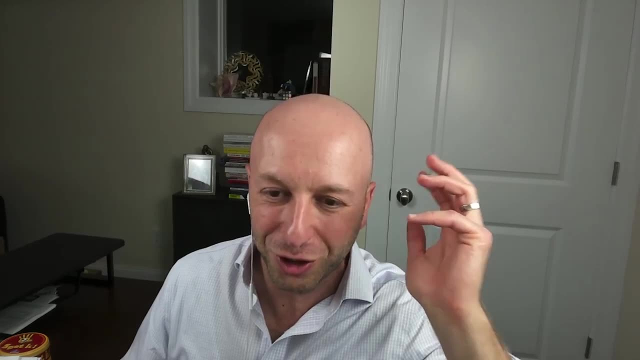 If you give me a definition in terms of other things, then you have to tell me what those things are. If you tell me what that is, you have to tell me what the thing before it is. Are the definitions a bad idea? You shouldn't have definitions. 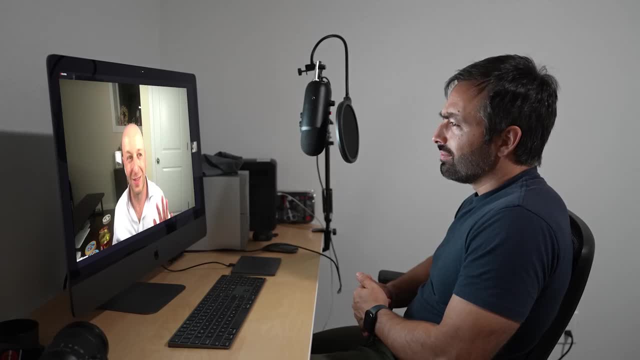 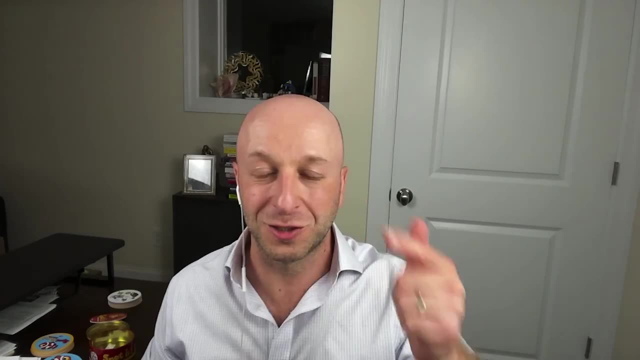 You should have undefined terms. I'm not going to tell you what a point is. I'm not going to tell you what a line is. I'm not going to tell you what a plane is. All I'm going to tell you is what the postulates are that they're assumed to satisfy. 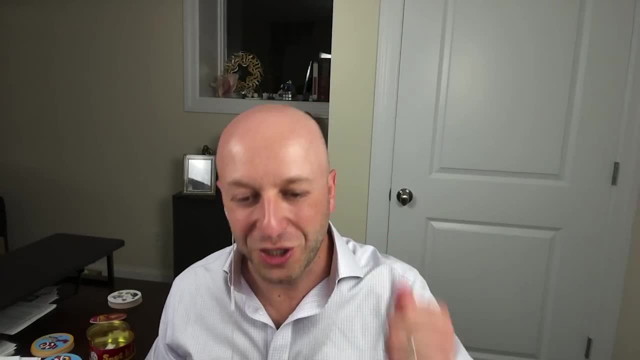 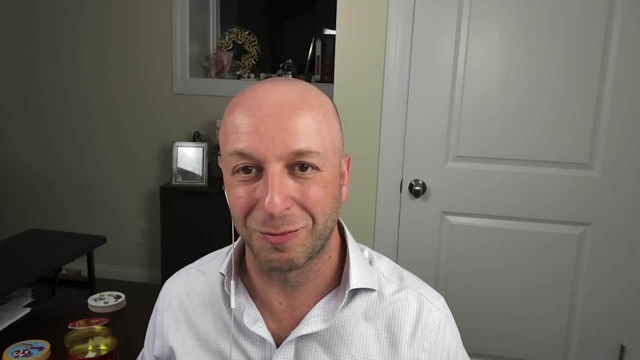 It's the relationships between the objects that's important, not the definitions of the objects themselves. And once you free your mind to that possibility, all of a sudden you realize that there is a perfectly good geometric world in which by line you mean great circle. 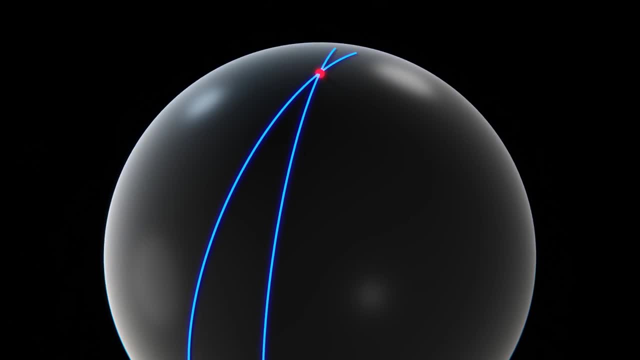 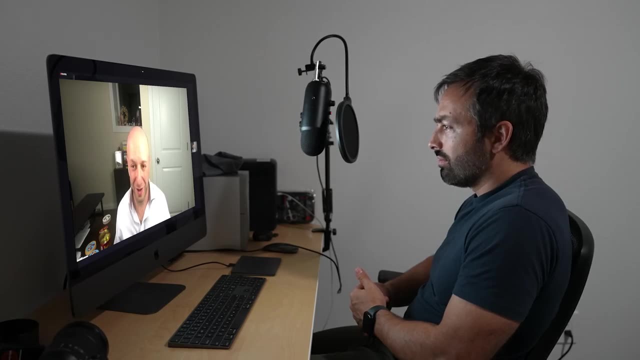 and by plane you mean sphere, and by point you mean a point on a sphere. and then four of those axioms are satisfied, just not the fifth. And similarly, there's another model, something called the disc model, for hyperbolic space. 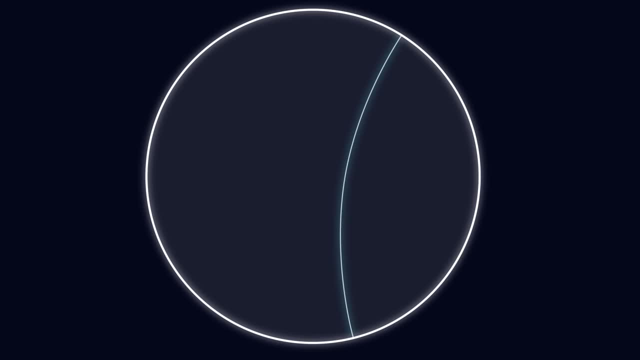 which the disc is the plane. What I mean by straight lines is arcs of circles that are orthogonal to the disc, and then points are points inside the disc, and the disc is the plane. See, you can think of geometry as a game. 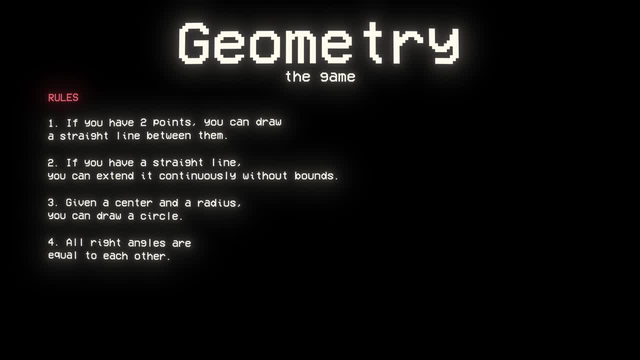 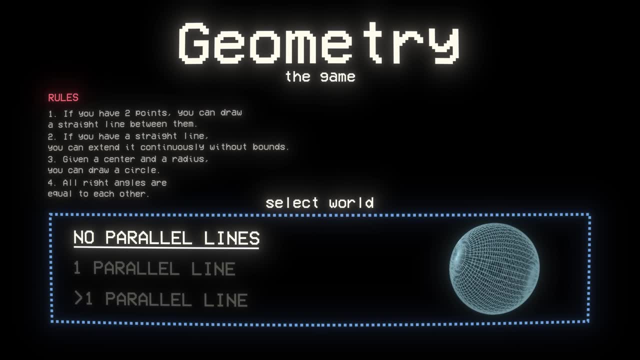 The first four postulates are like the minimum rules required to play that game. and then the fifth postulate selects the world that you'll play in. If you pick that there are no parallel lines, you're playing in spherical geometry If you choose one parallel line. 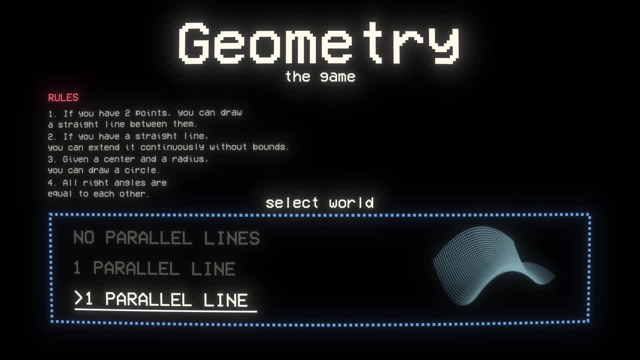 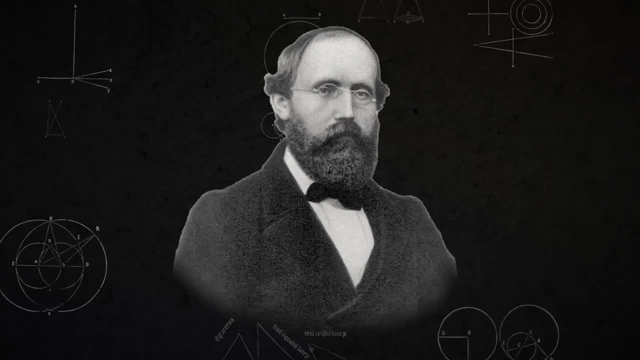 you're playing in flat geometry, And if you go for more than one parallel line, then you're playing in hyperbolic geometry. But Riemann decided to take it one step further. Instead of selecting just one world to play in, why not combine them all into one? 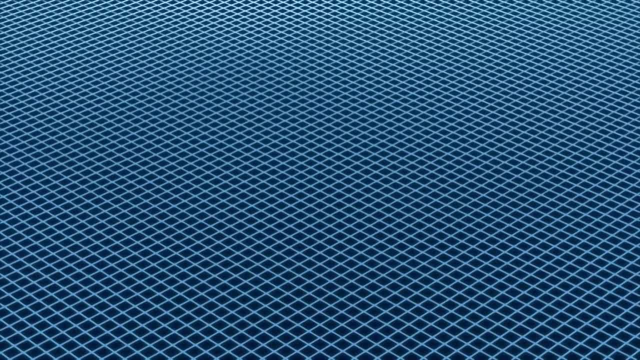 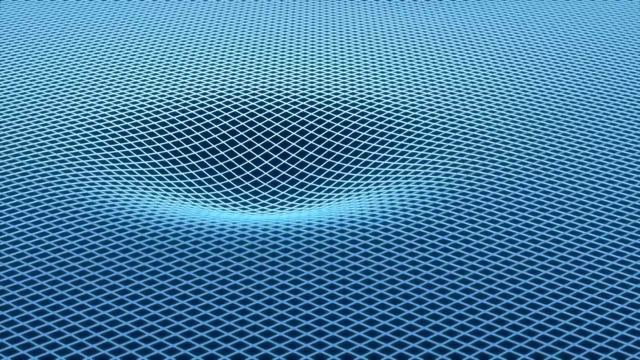 During his inaugural speech in 1854,, he laid out the groundwork for a geometry where the curvature could differ from place to place. One part might be flat, another part might be slightly curved and yet another part might have a very strong curvature. 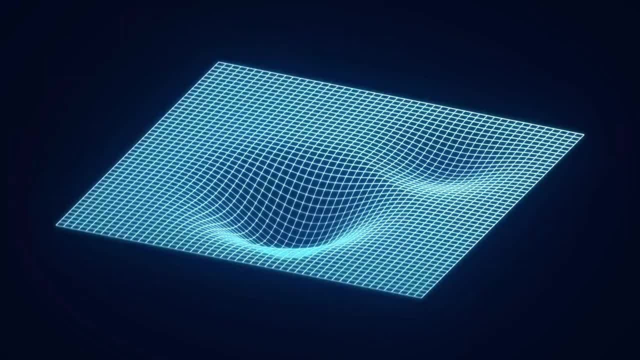 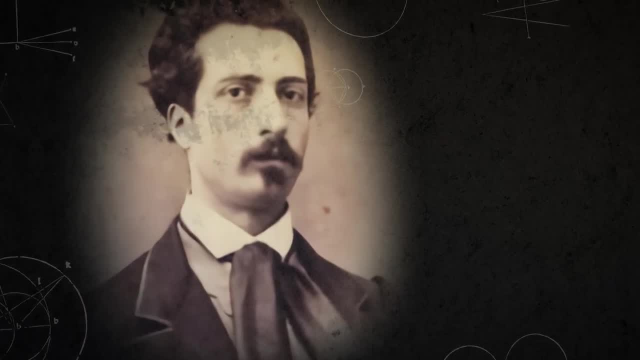 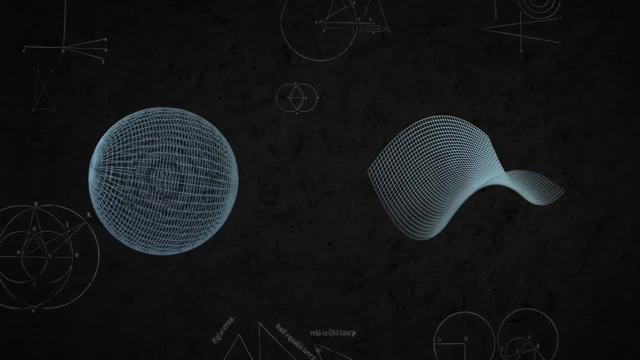 And this geometry wouldn't be limited to two-dimensional planes either. It could be extended to three or more dimensions. Another breakthrough came in 1868, when Eugenio Beltrami unequivocally proved that hyperbolic and spherical geometry were just as consistent as Euclid's flat geometry. 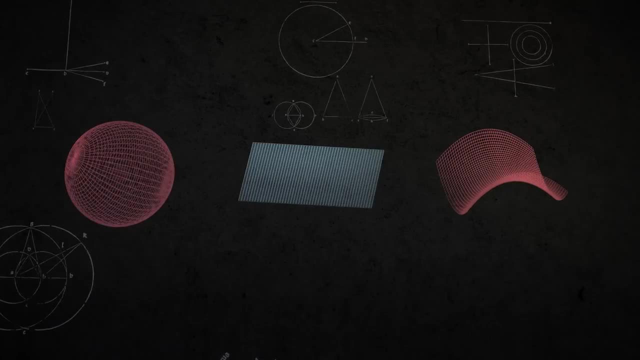 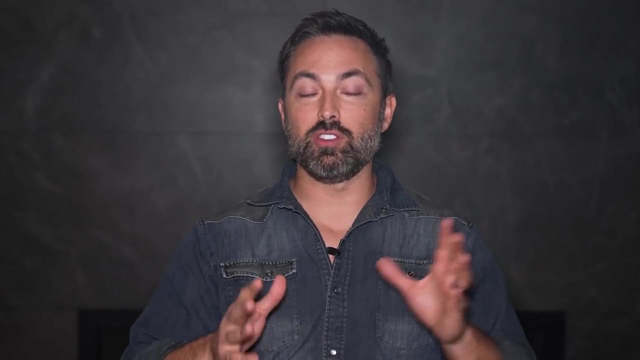 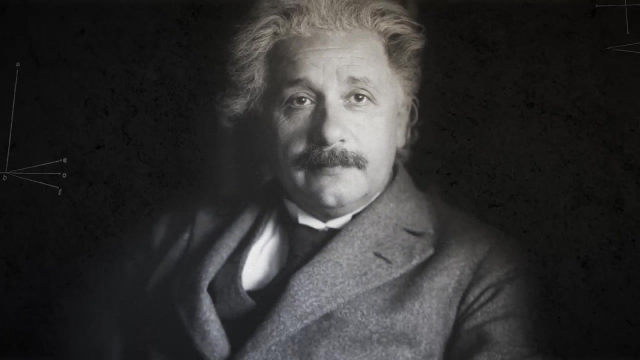 That is, if there were any inconsistencies in hyperbolic or spherical geometry, then they must also be present in Euclid's flat geometry. The prospects for these new geometries were looking great, and it turns out this was just the beginning In 1905,. 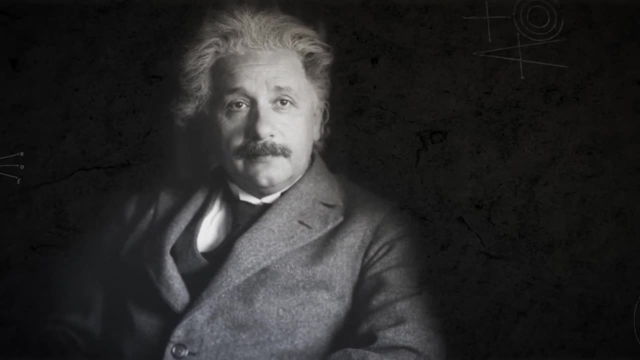 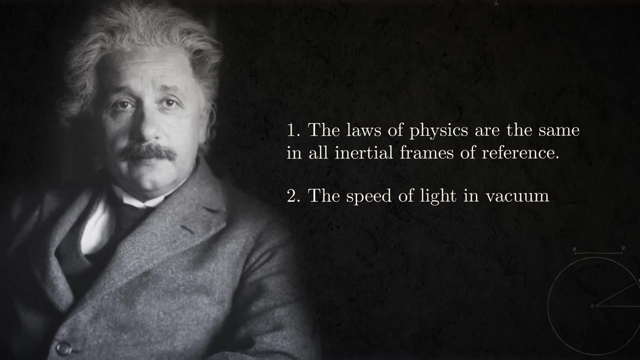 Einstein proposed the special theory of relativity, which is based on just two postulates: the laws of physics are the same in all inertial frames of reference. and two: the speed of light in a vacuum is the same for all inertial observers. 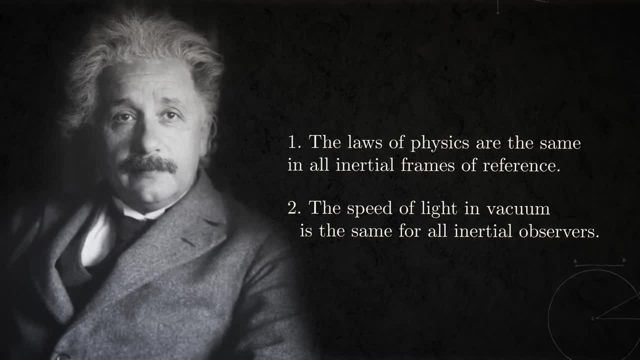 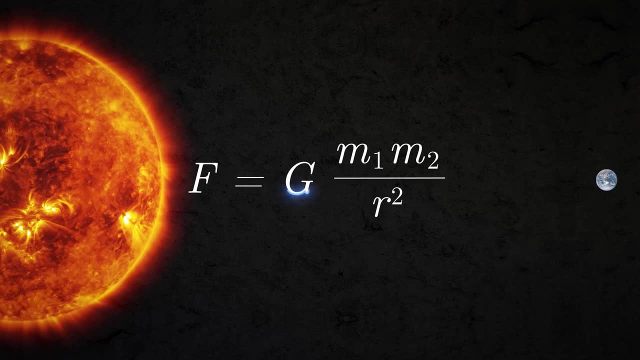 So as a result, space and time must be relative. But that created a problem for Newtonian gravity, because according to Newton the force of gravity is inversely proportional to the distance between the two objects squared. But in Einstein's special relativity 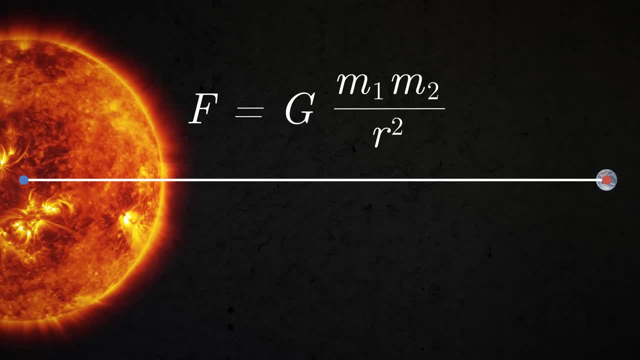 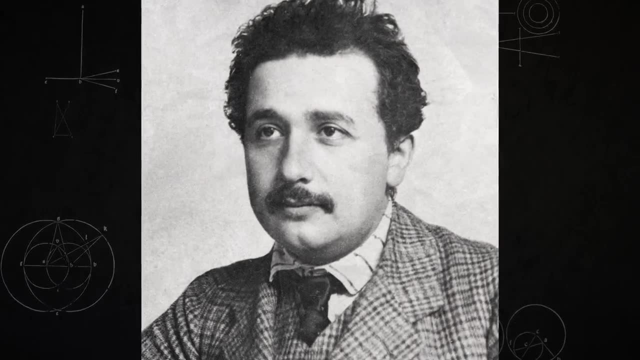 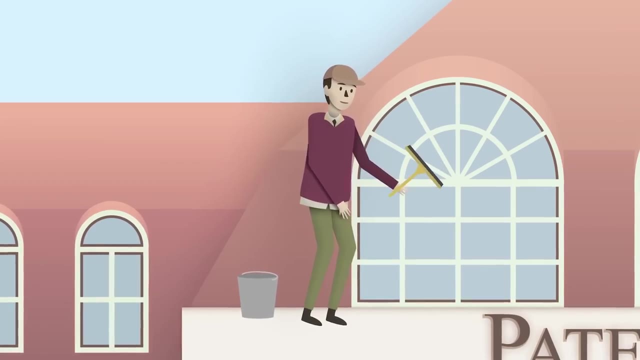 that distance is no longer well defined. In whose reference frame are we measuring? And so Einstein had to find a way to reconcile relativity and gravity. Two years later, in 1907, Einstein had the happiest thought of his life. He imagined a man falling off the roof of a house. 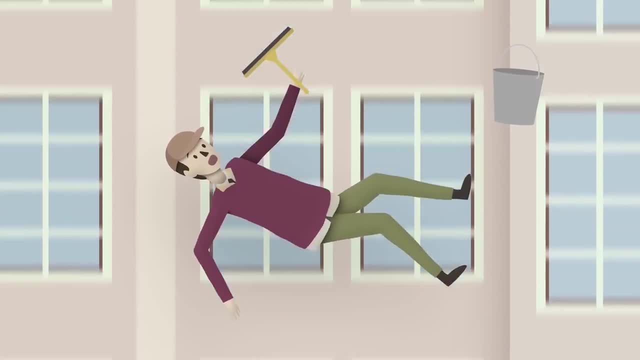 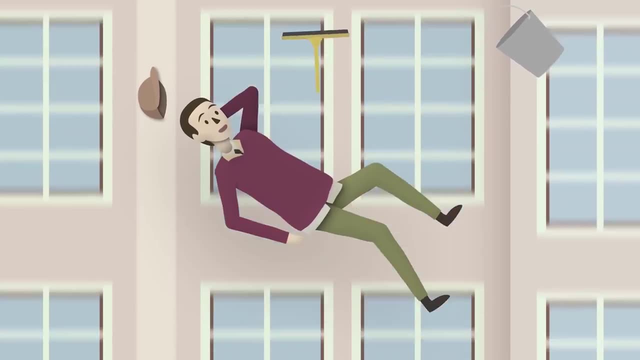 And what made Einstein so joyful is that he realized that while the man is falling, he would feel absolutely weightless, And if he let go of an object, it would just remain in uniform motion relative to him. It would be just like being in space. 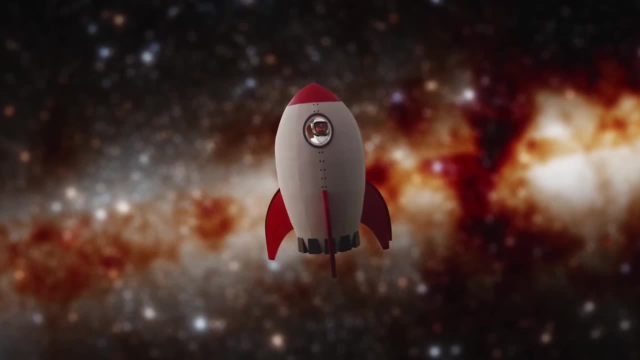 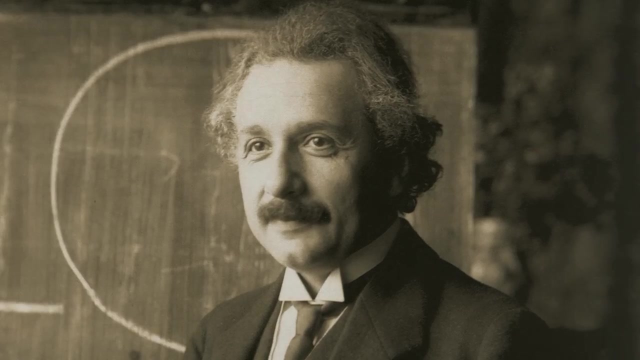 not near any masses floating around in a spaceship at constant velocity, And that is an inertial observer. Now here's the big breakthrough: Einstein realized that they're not just similar, they are identical, Because there is no experiment you could do to determine whether you're in free fall. 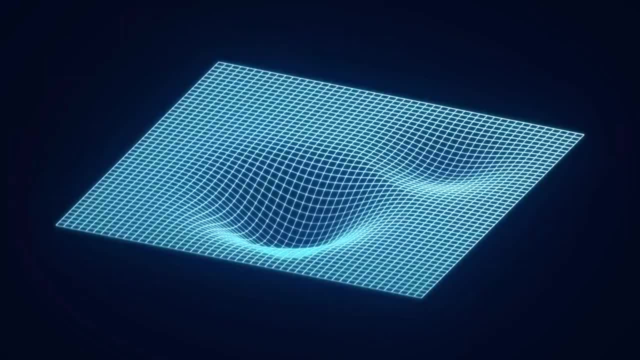 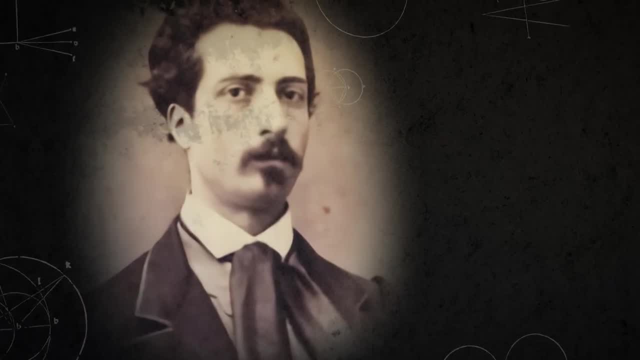 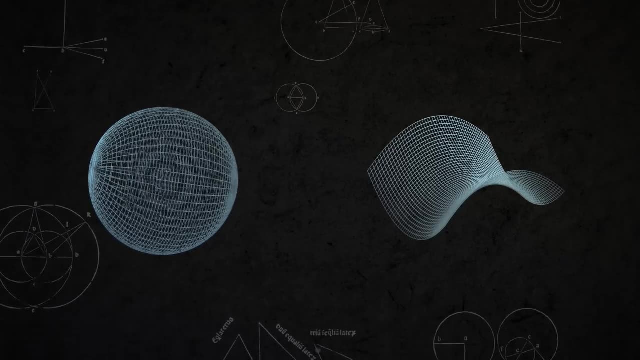 And this geometry wouldn't be limited to two-dimensional planes either. It could be extended to three or more dimensions. Another breakthrough came in 1868, when Eugenio Beltrami unequivocally proved that hyperbolic and spherical geometry were just as consistent as Euclid's flat geometry. 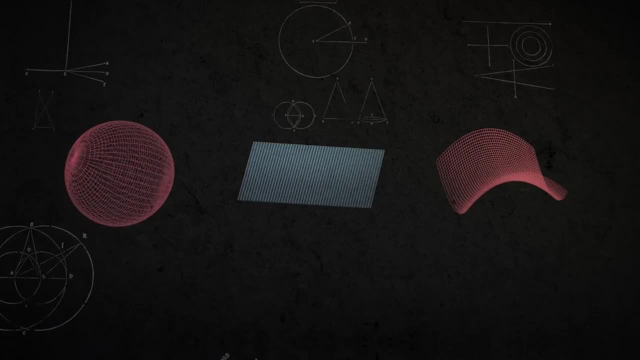 That is, if you look at Euclid's flat geometry, it's just as consistent as Euclid's flat geometry. That is, if you look at Euclid's flat geometry, it's just as consistent as Euclid's flat geometry. If there were any inconsistencies in hyperbolic or spherical geometry, 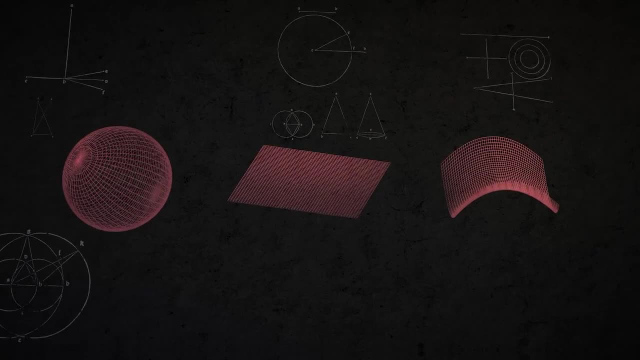 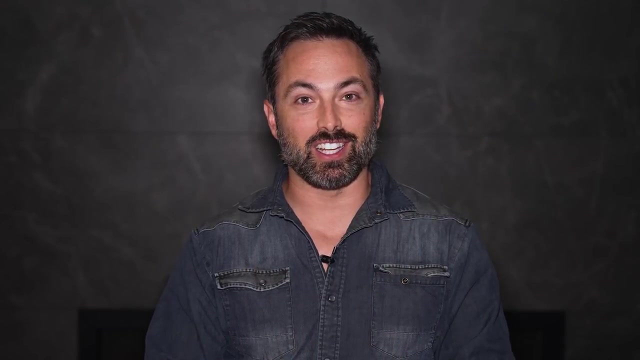 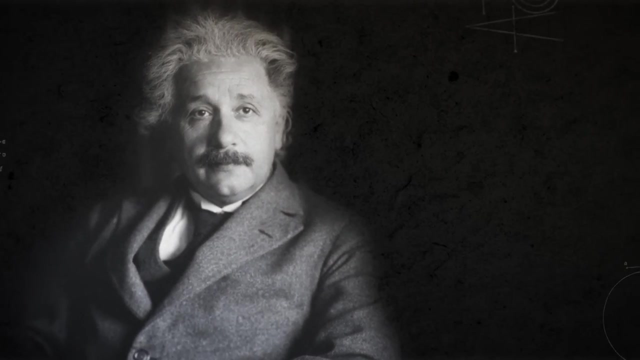 then they must also be present in Euclid's flat geometry. The prospects for these new geometries were looking great, and it turns out this was just the beginning. In 1905, Einstein proposed the special theory of relativity, which is based on just two postulates. 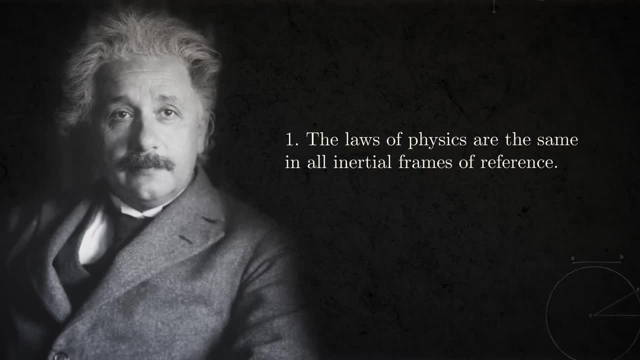 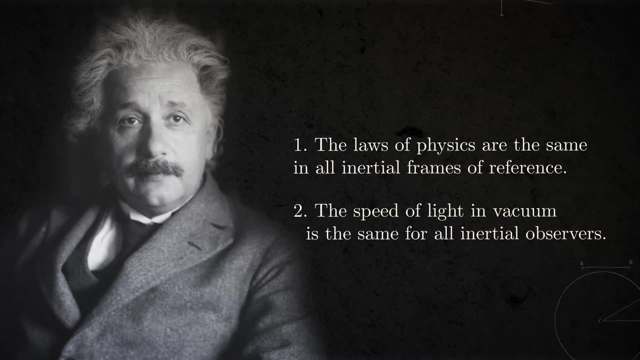 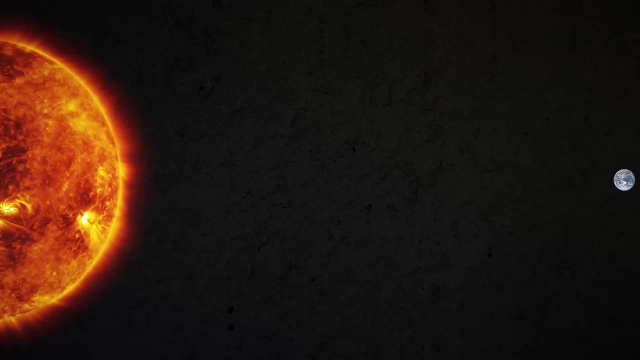 One, the laws of physics are the same in all inertial frames of reference and, two, the speed of light in a vacuum is the same for all of them. So, as a result, space and time must be relative. But that created a problem for Newtonian gravity, because, according to Newton, 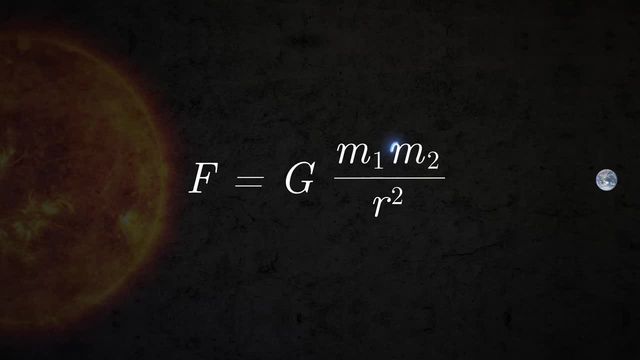 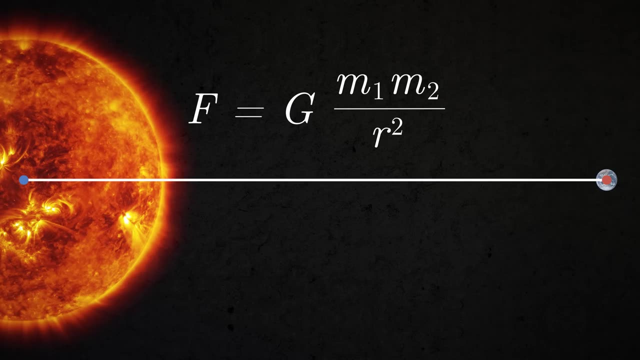 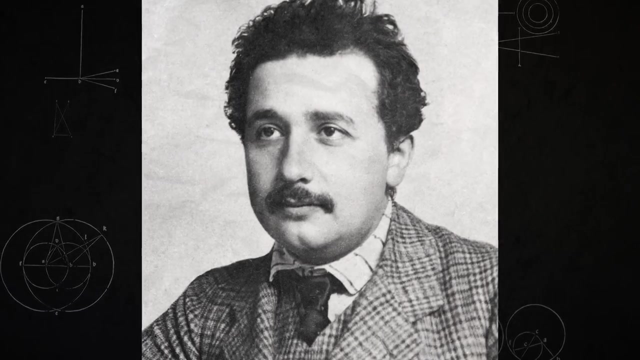 the force of gravity is inversely proportional to the distance between the two objects squared. But in Einstein's special relativity that distance is no longer well defined. In whose reference frame are we measuring? And so Einstein had to find a way to reconcile relativity and gravity. 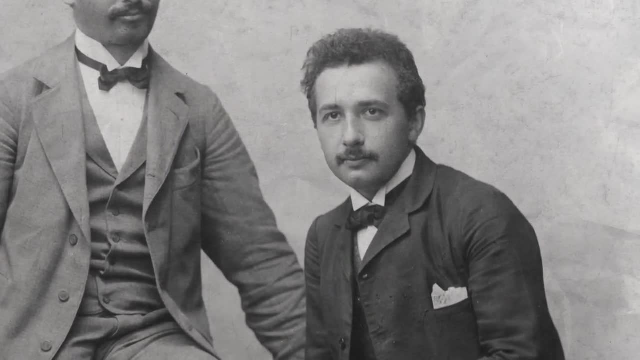 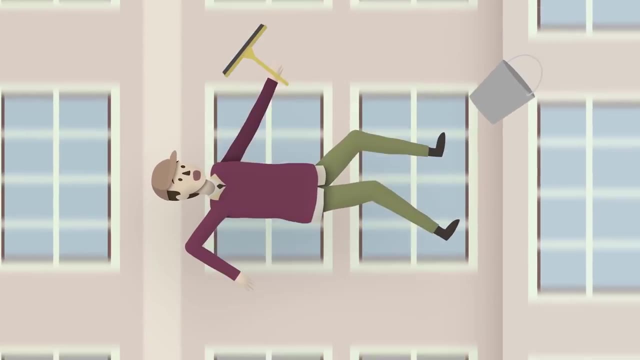 Two years later, in 1907, Einstein had the happiest thought of his life. He imagined a man falling off the roof of a house, And what made Einstein so joyful is that he realized that while the man is falling, he would feel absolutely weightless. 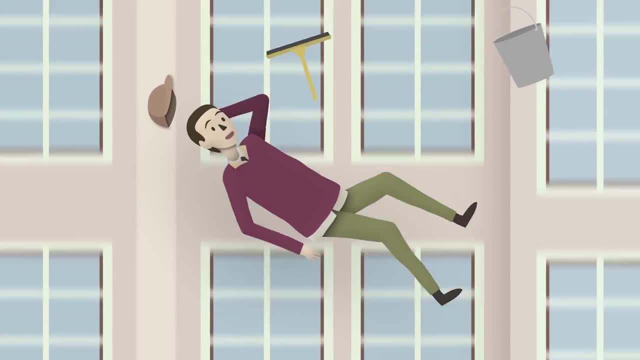 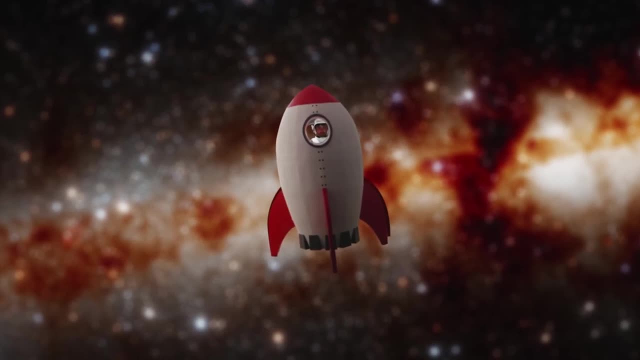 And if he let go of an object, it would just remain in uniform motion relative to him. It would be just like being in space, not near any masses floating around in a spaceship at constant velocity, And that is an inertial observer. 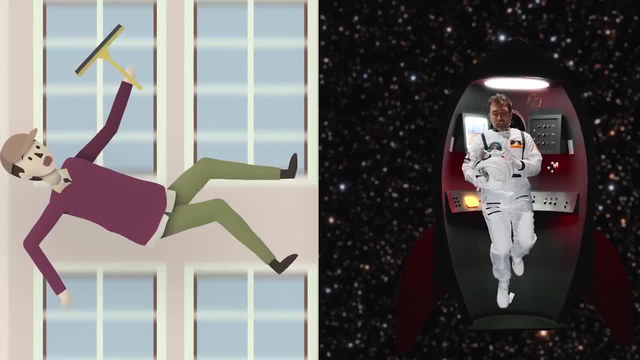 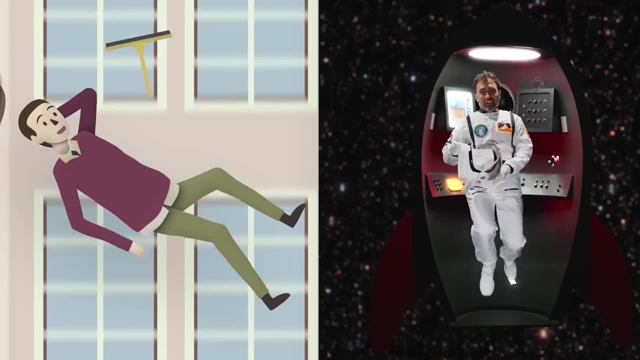 Now here's the big breakthrough: Einstein realized that they're not just similar, they are identical, Because there is no experiment you could do to determine whether you're in free fall in a uniform gravitational field or whether you're in deep space, not near any massive objects. 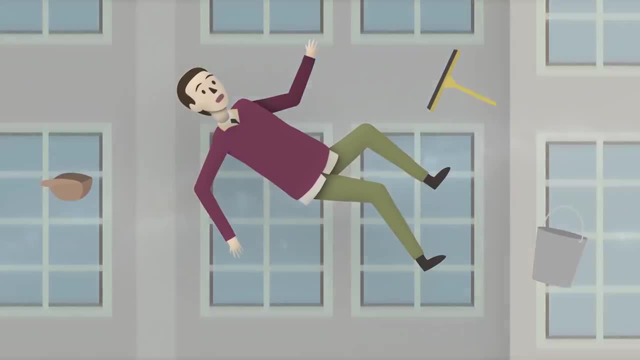 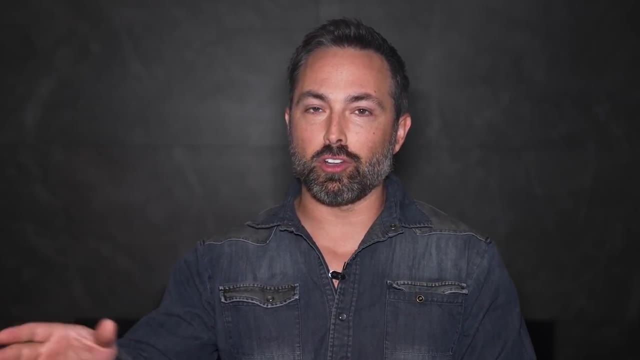 in a uniform gravitational field, or whether you're in deep space, not near any massive objects, And so the free falling man too must be an inertial observer, meaning he is not accelerating and he's not experiencing any force of gravity. 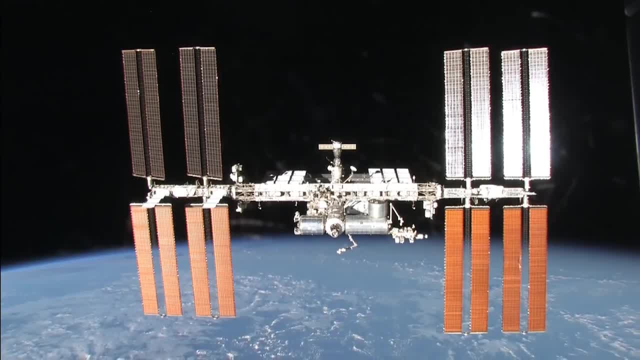 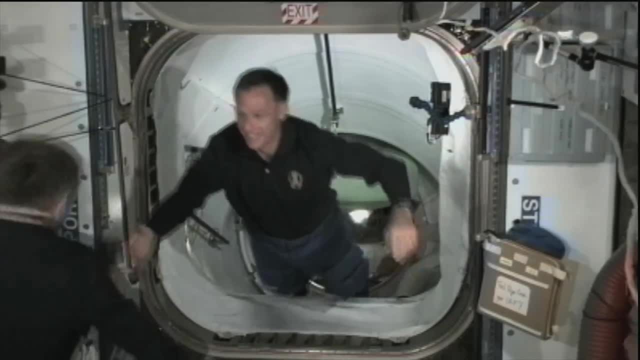 But if gravity is not a force, then how do you explain things like the space station orbiting Earth? Shouldn't it just fly off in a straight line? Well, astronauts in the space station also feel weightless, And that's the key. 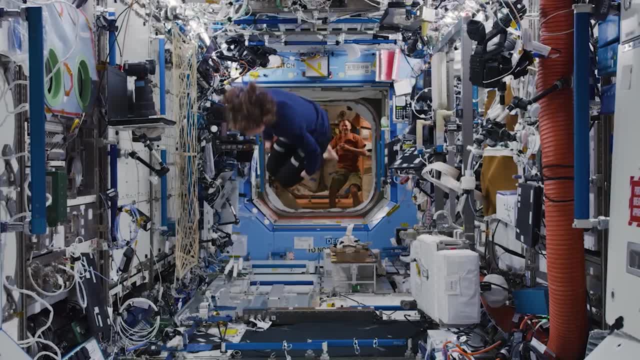 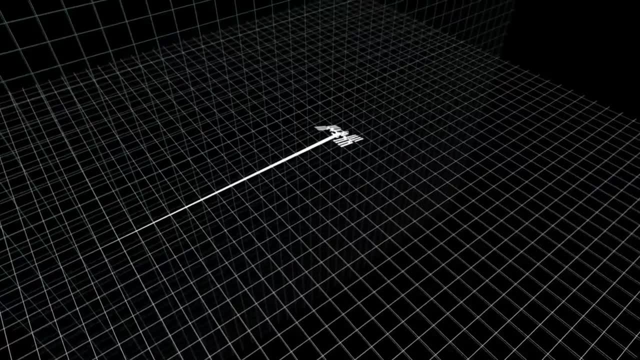 It feels just as if they're traveling at constant velocity in a straight line. It feels like that because that's precisely what they're doing: They're traveling in a straight line. How then, could that straight line appear curved to a distant observer? The answer is because the space station 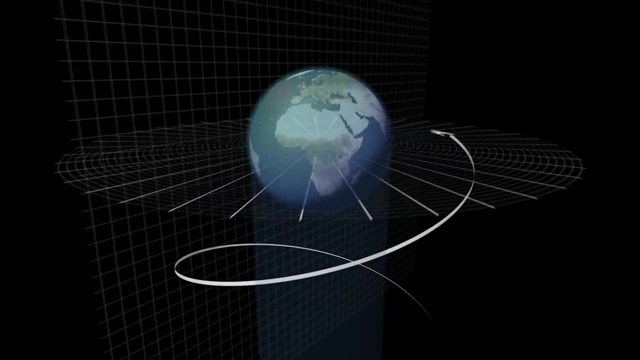 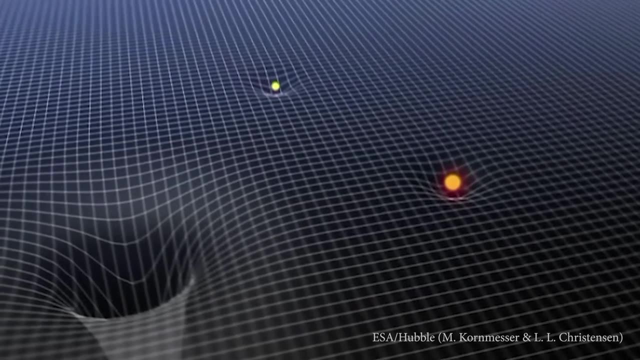 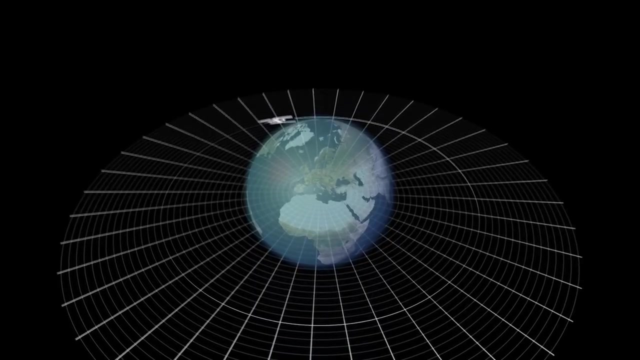 is curved. the space time that straight line is on is curved- See massive objects, curve space time And objects moving through curved space time will follow the shortest path through that curved geometry, the geodesic. So, while astronauts in the space station 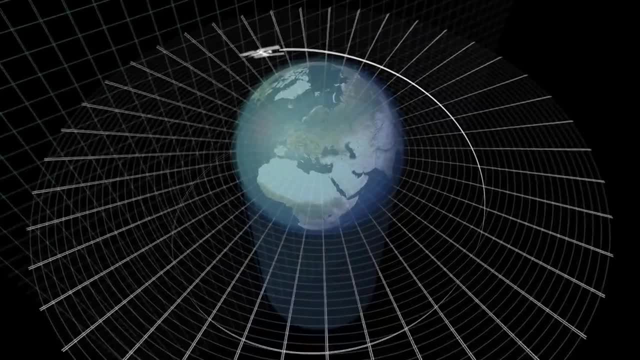 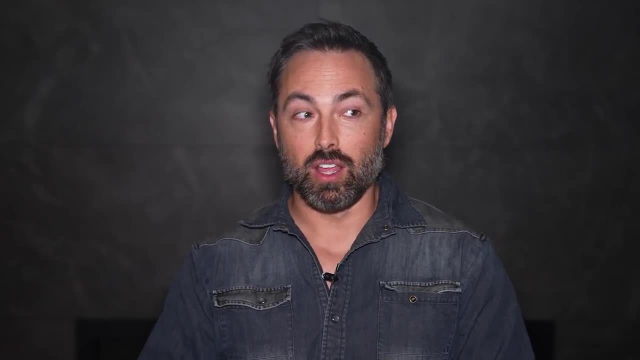 are following a straight line. it appears curved to a distant observer because the Earth curves the space time around it. So the behavior of straight lines is core to understanding the universe we live in And in the more than 100 years since it was published. 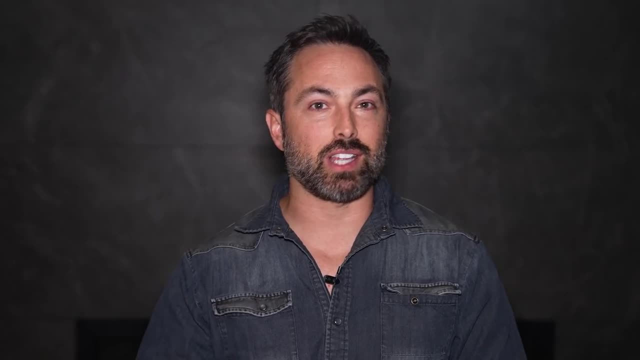 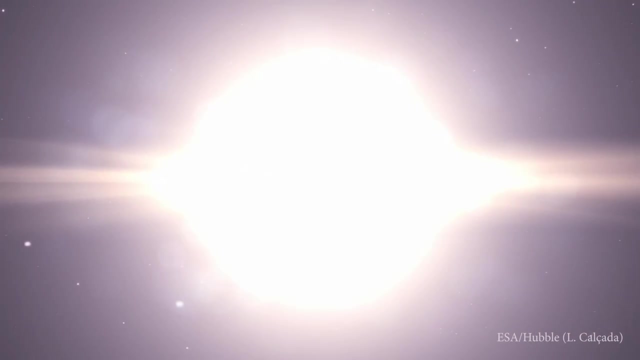 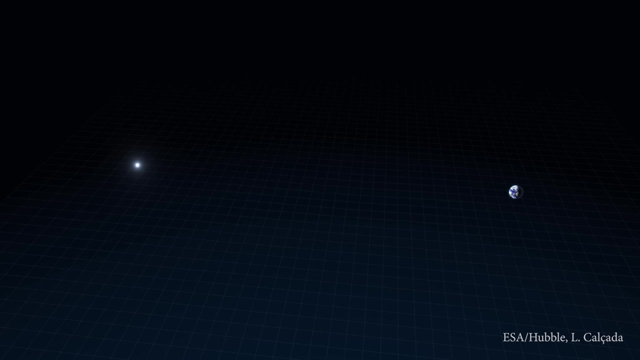 the general theory of relativity has been remarkably successful. In 2014,, astronomers briefly observed a supernova, a violent and extremely bright death of a star. In fact, they saw the exact same supernova in four different places. How Well in between the supernova and Earth. 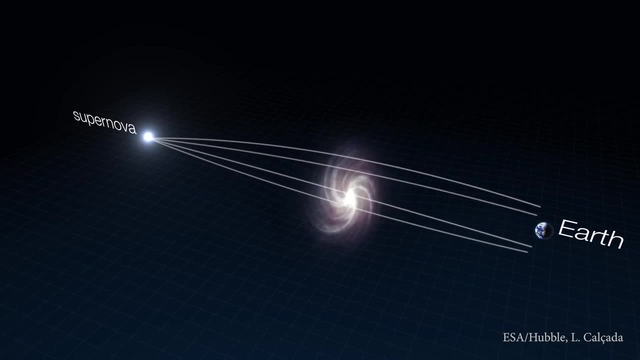 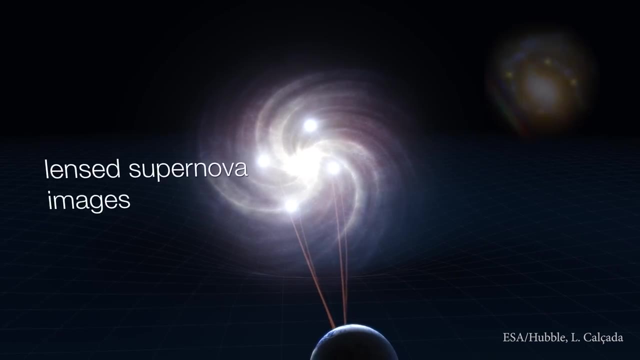 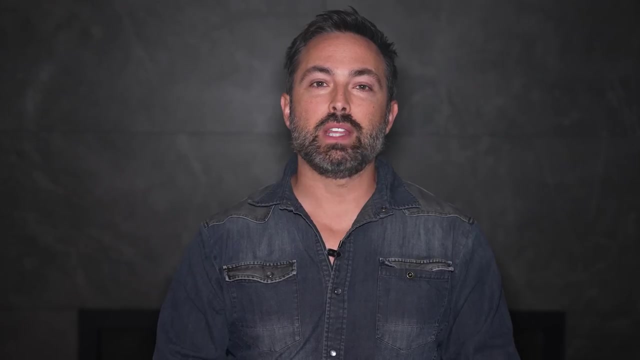 there was a massive galaxy which curved space time, And even the supernova, which was spreading out in all directions, had several different paths to reach the Earth, And four of those reached Earth at approximately the same time. The galaxy had functioned as a massive gravitational lens. The astronomers realized that other galaxies in the cluster might also lens the light from that supernova, but with different path lengths and gravitational potentials, So the light would reach Earth at different times. After careful modeling they predicted the same play of that supernova. 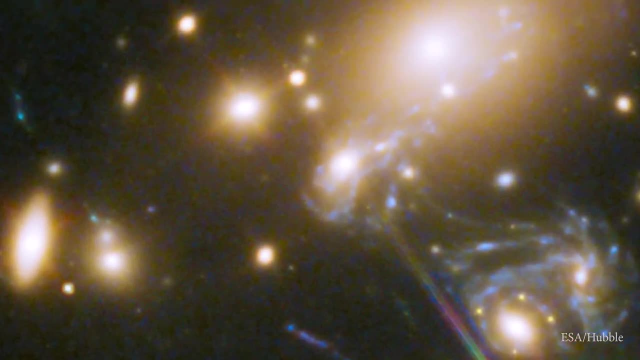 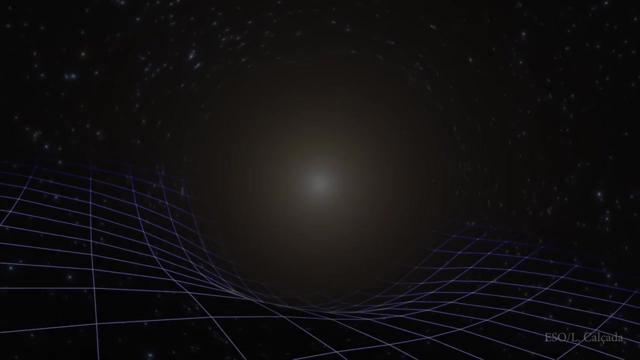 just a year later, And on the 11th of December 2015,. just as predicted, they saw the same supernova once more. In addition to being able to observe the effects of curved space time, we can now even measure the ripples. 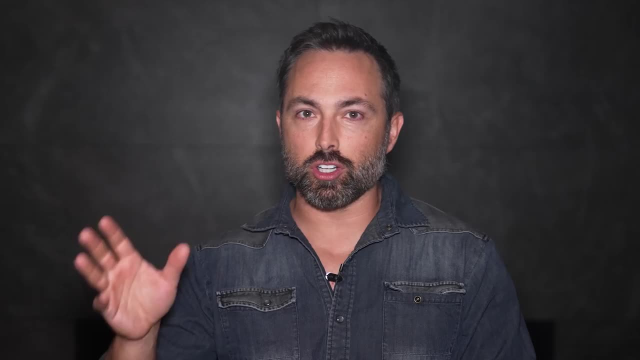 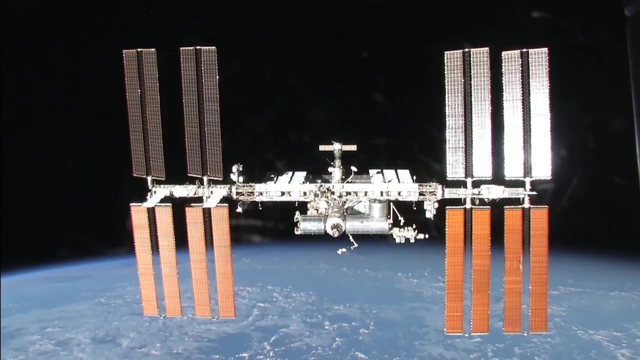 And so the free-falling man too must be an inertial observer, meaning he is not accelerating and he's not experiencing any force of gravity. But if gravity is not a force, then how does it make a man fall? How do you explain things like the space station orbiting Earth? 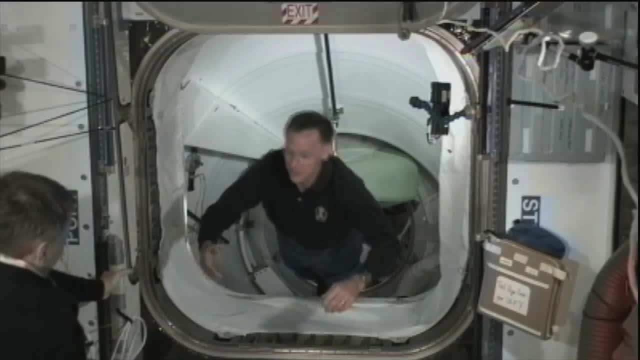 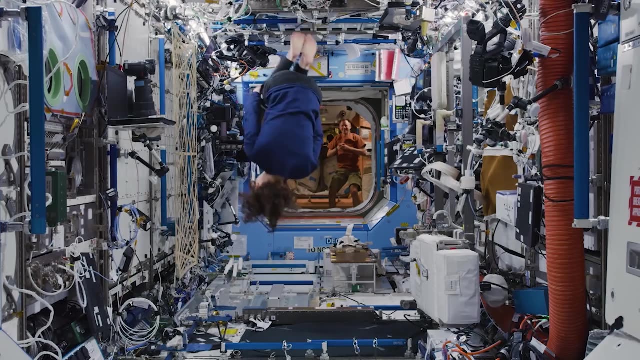 Shouldn't it just fly off in a straight line? Well, astronauts in the space station also feel weightless, And that's the key. It feels just as if they're traveling at constant velocity in a straight line. It feels like that because that's precisely what they're doing. 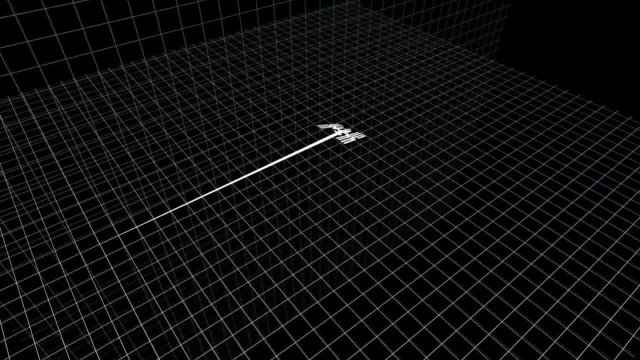 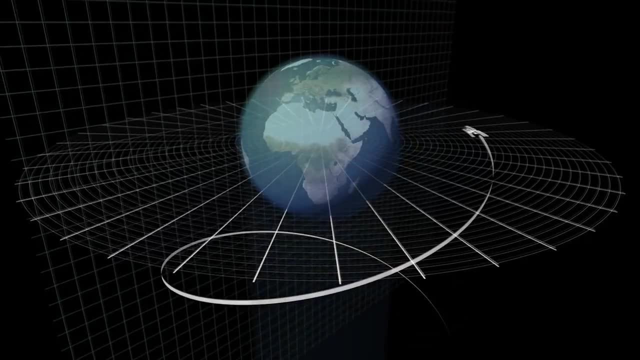 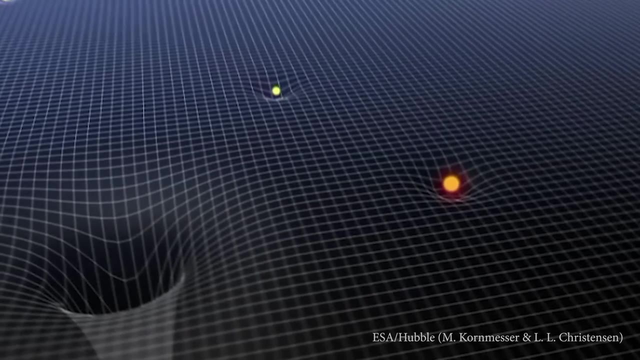 They're traveling in a straight line. How then could that straight line appear curved to a distant observer? The answer is because the space-time that straight line is on is curved. See massive objects, curve space-time And objects moving through curved space-time will follow the shortest path. 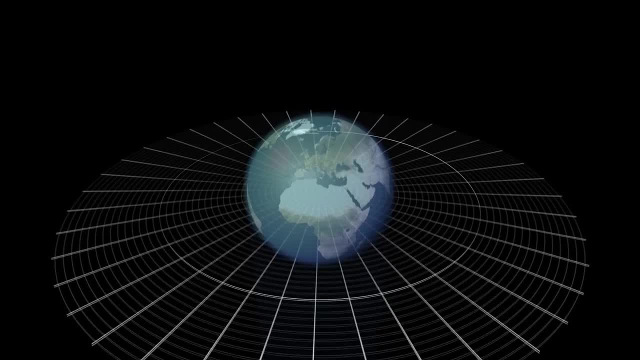 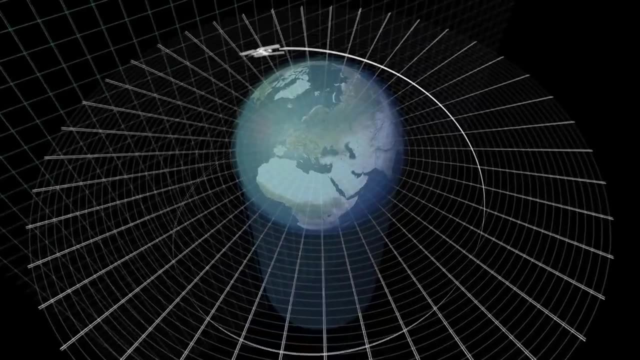 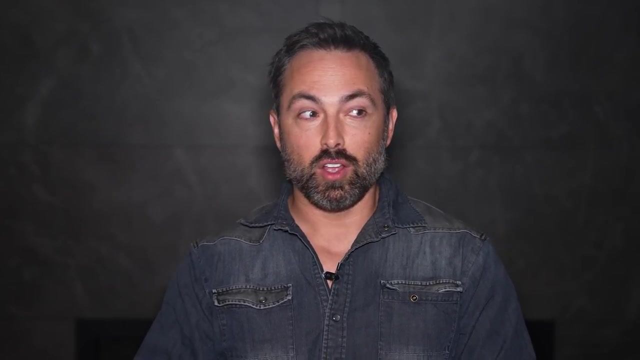 through that curved geometry, the geodesic. So while astronauts in the space station are following a straight line, it appears curved to a distant observer because the Earth curves the space-time around it. So the behavior of straight lines in curved geometries is core to understanding the universe. 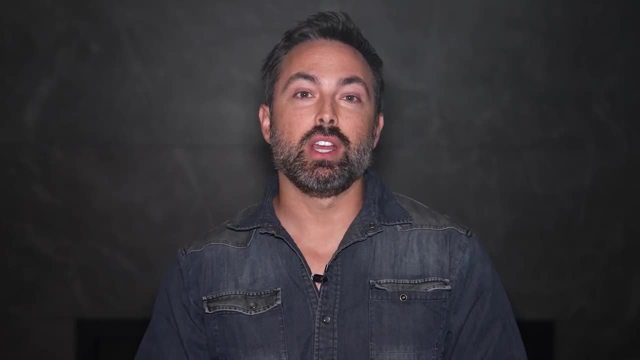 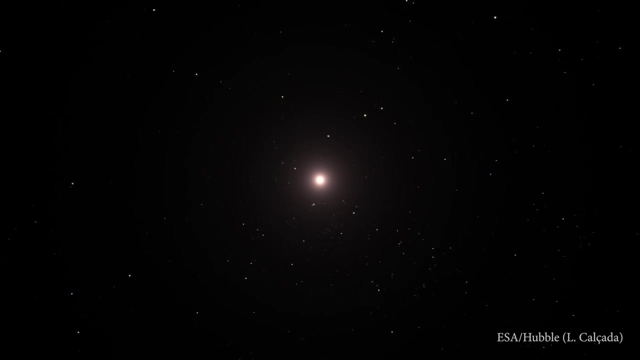 we live in, And in the more than 100 years since it was published, the general theory of relativity has been remarkably successful. In 2014,, astronomers briefly observed a supernova, a violent and extremely bright death of a star. 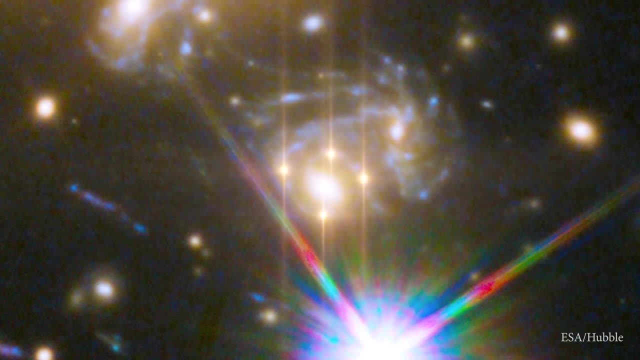 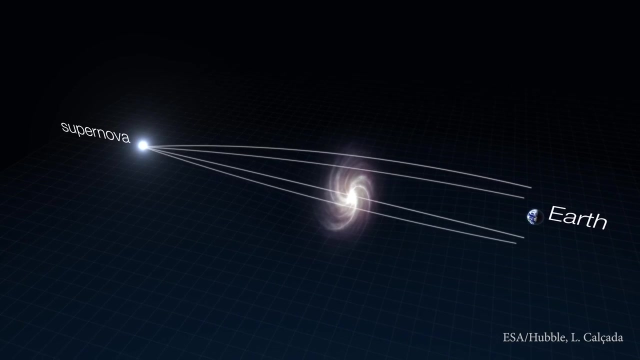 In fact they saw the exact same supernova in four different places. How Well in between the supernova and Earth there was a massive galaxy which curved space-time, So light from the supernova which was spreading out in all directions. 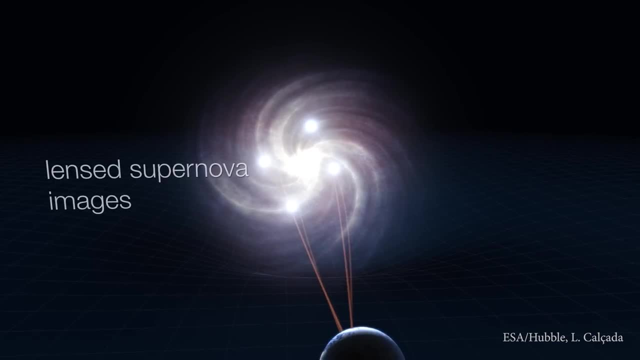 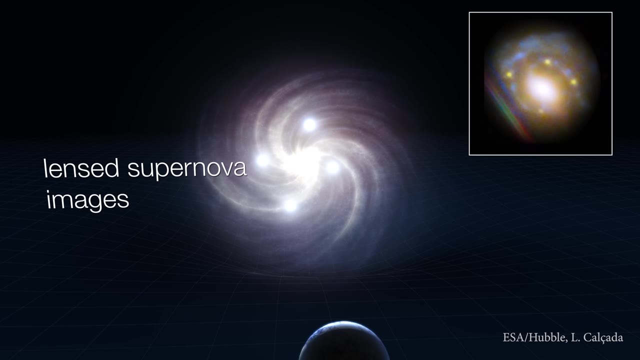 had several different paths to the Earth And four of those reached Earth at approximately the same time. The galaxy had functioned as a massive gravitational lens. The astronomers realized that other galaxies in the cluster might also lens the light from that supernova, but with different path lengths and gravitational potentials. 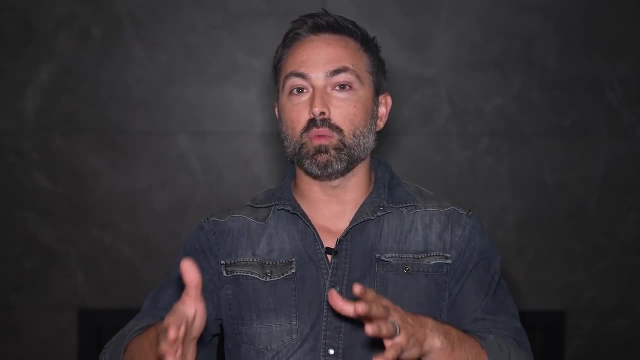 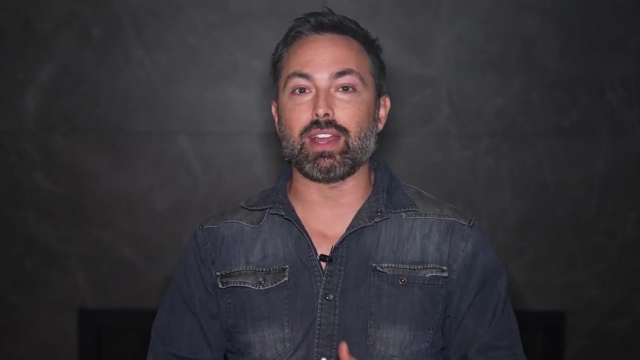 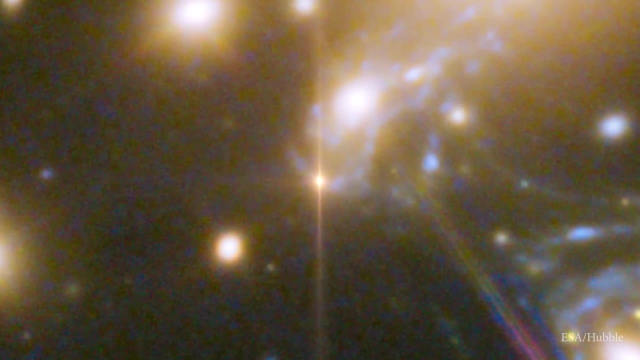 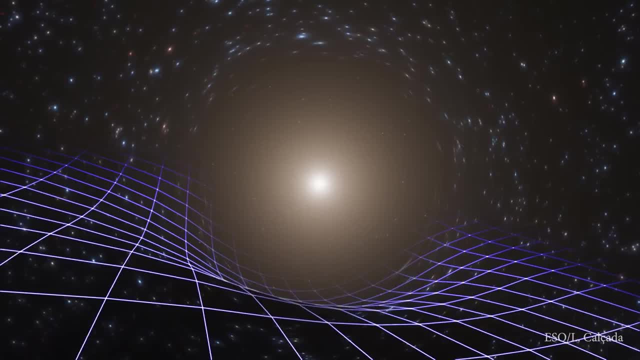 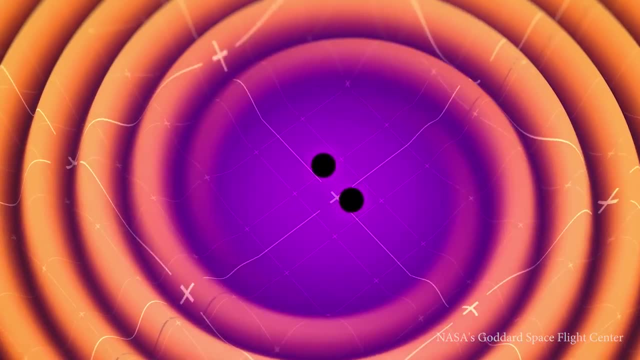 In addition to being able to observe the effects of curved space-time, we can now even measure the ripples of space-time itself: gravitational waves formed by cosmic events far, far away, Like the merger of black holes, And, according to a recent survey by NaNoGrav. 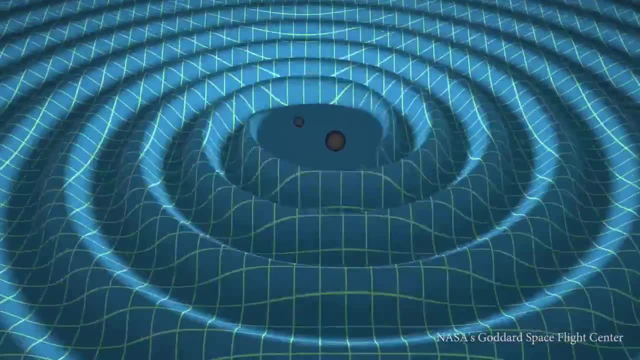 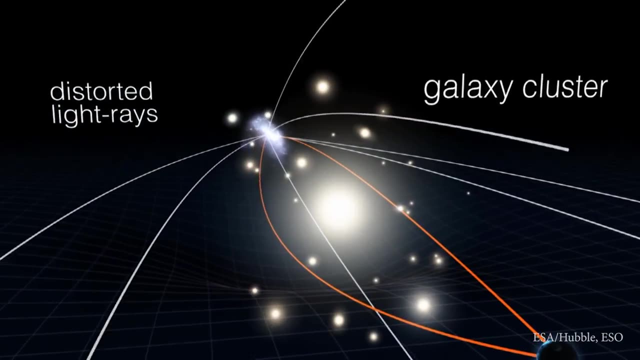 the fabric of space-time seems to be buzzing with the remnants of grand cosmic events. In the hundred years since General Relativity was published, countless findings have supported its predictions, and at its very core are the curved geometries of Boliae and Riemann. 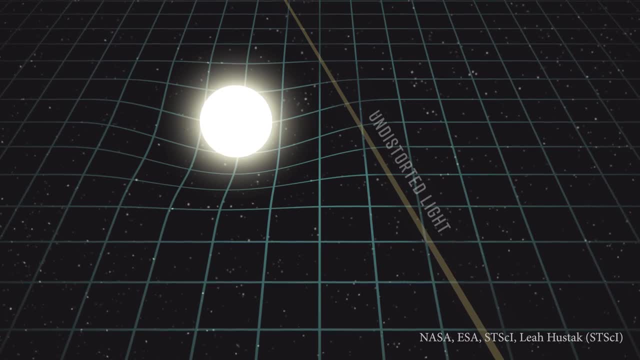 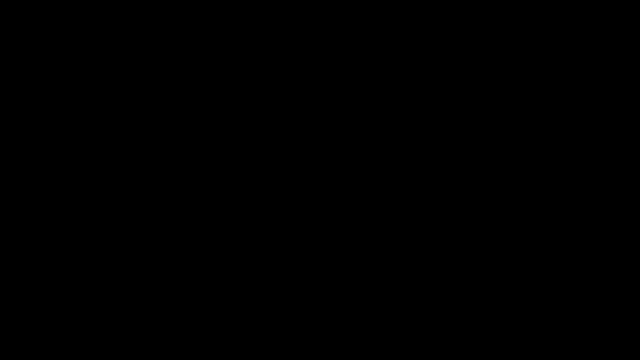 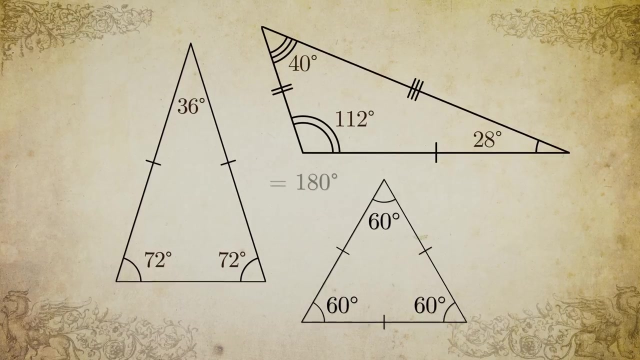 But so far all the effects we've looked at are local distortions of spacetime. What is the shape of the entire universe? Using the differences between the geometries, we can find that out too. In flat geometry. we expect all the angles of a triangle to add up to 180 degrees without 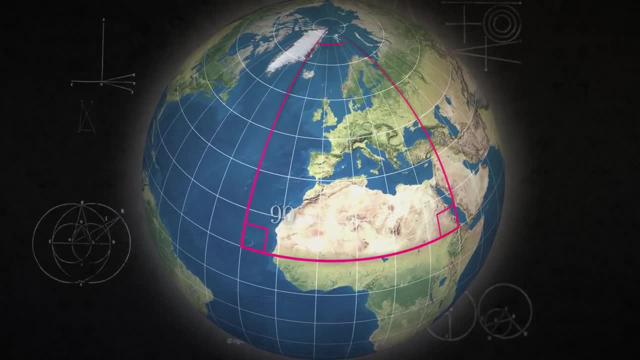 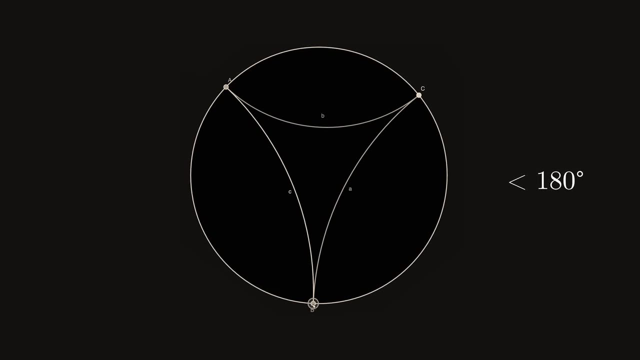 fail. But in spherical geometry the angles don't add up to 180 degrees but to more. Similarly, in hyperbolic geometry the angles add up to less than 180 degrees. So to determine the shape of the universe you just need to measure the angles of a triangle. 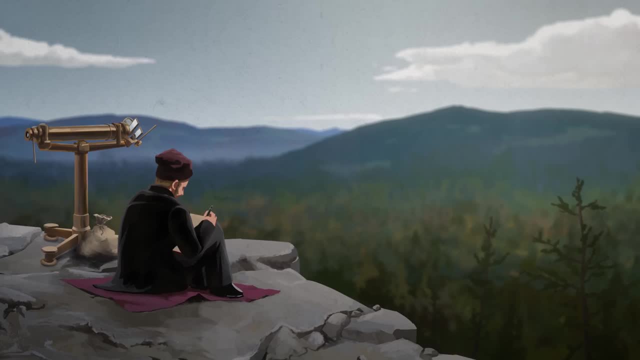 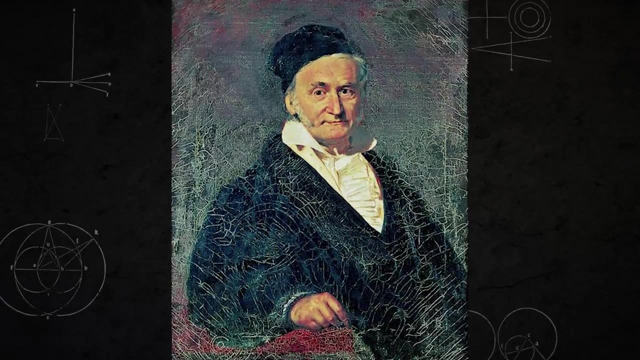 And measuring a triangle is precisely what Gauss was doing 200 years ago. In fact, this led some to speculate that he was actually trying to measure the angles of the universe. He was trying to measure the curvature of space itself, The angle he found. 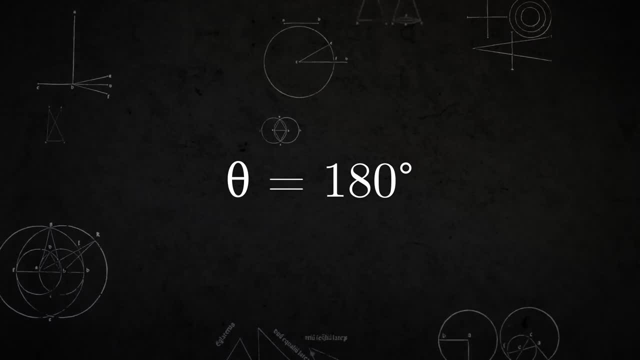 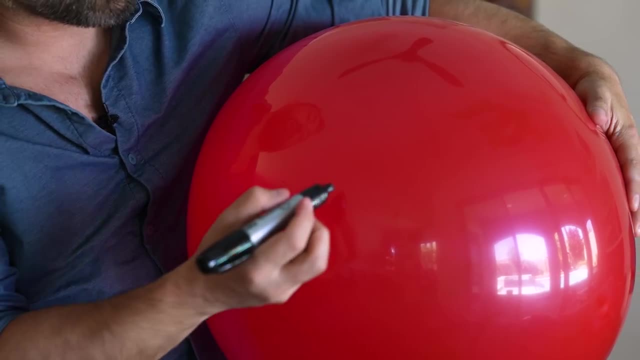 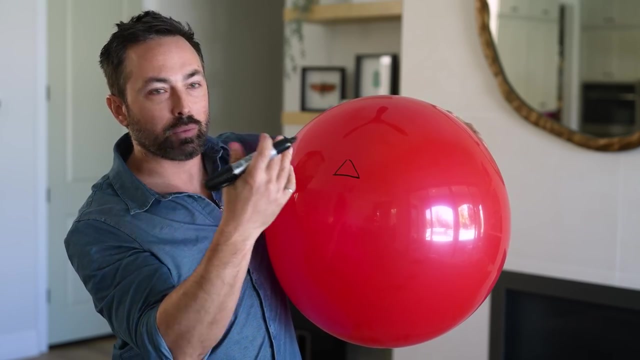 180 degrees within observational error, But that shouldn't be very surprising. Take this balloon, for example, which approximates a sphere If I draw a small triangle on it. well, the surface I'm drawing on is basically flat, so the angles inside the triangle will add up to essentially 180 degrees. 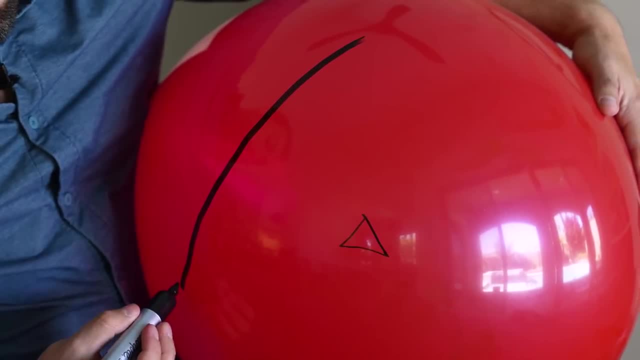 Only if I make the triangle large enough will the effects of curvature come out. And that's what we're going to do. We're going to measure the curvature of space And then we'll add up the angles of the universe and the angles of the universe. 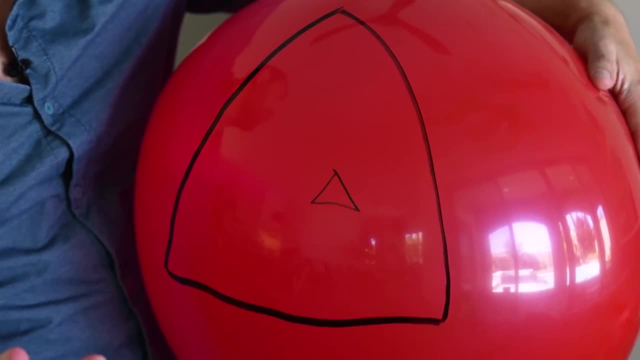 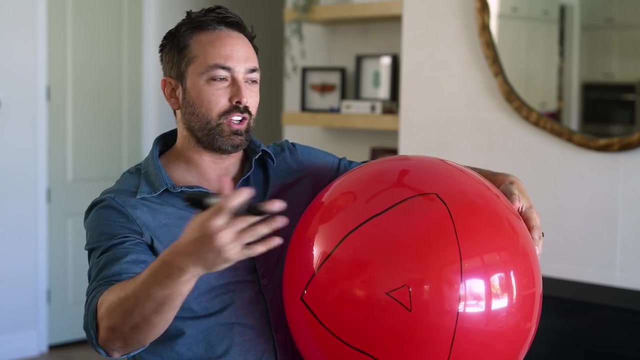 And then the angles in the triangle will add up to more than 180 degrees. And this was the problem with Gauss' experiment. Even if he was trying to measure the curvature of space itself, for which there is no solid evidence, the triangle he measured would have been far too small relative to the size of 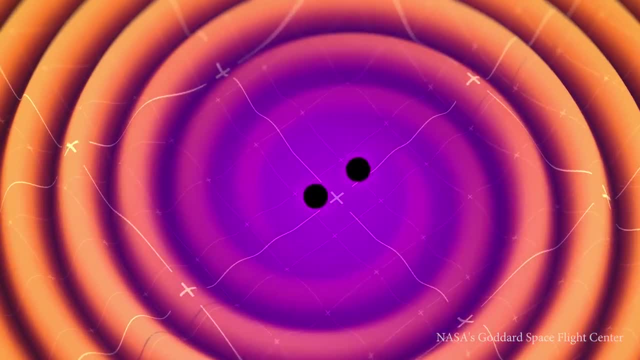 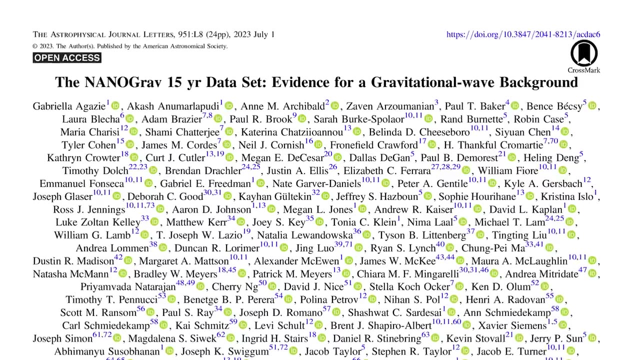 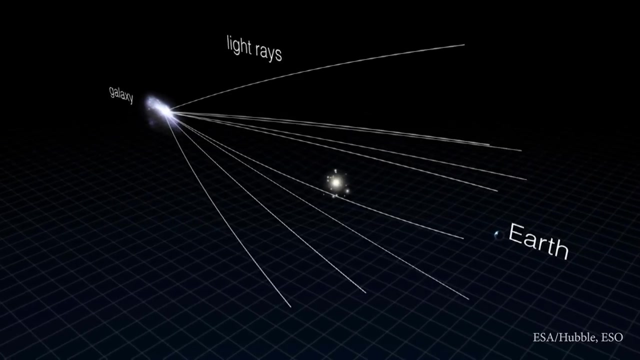 of space time itself: Gravitational waves formed by cosmic events far, far away, Like the merger of black holes, And according to a recent survey by Nanograv, space time seems to be buzzing with the remnants of grand cosmic events In the hundred years. 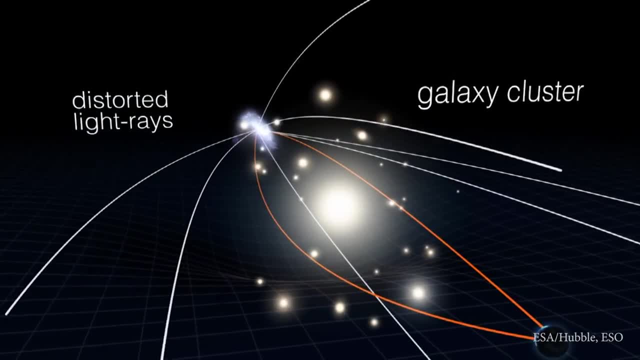 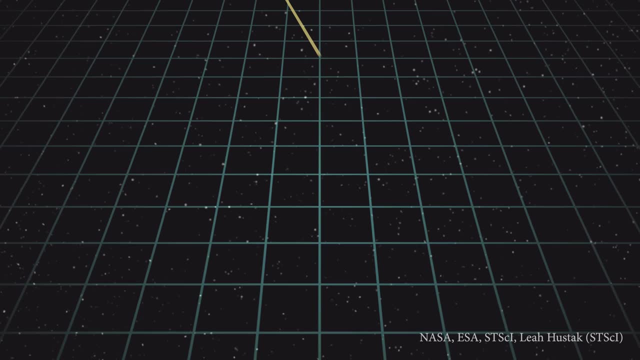 since General Relativity was published, countless findings have supported its predictions, And at its very core are the curved geometries of Bolyai and Remon. But so far all the effects we've looked at are local distortions of space time. 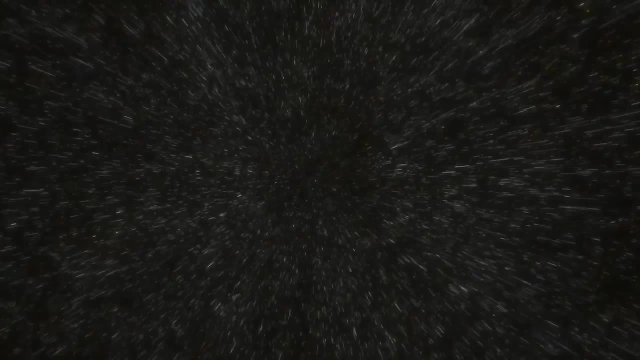 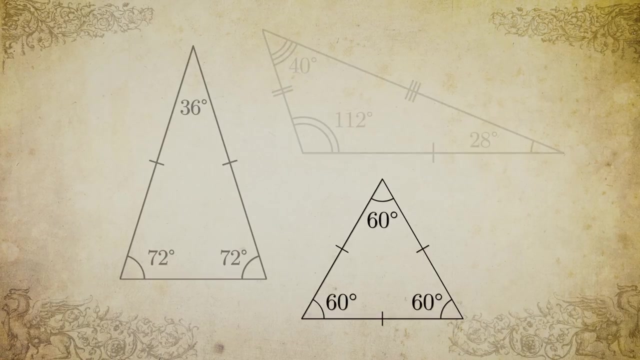 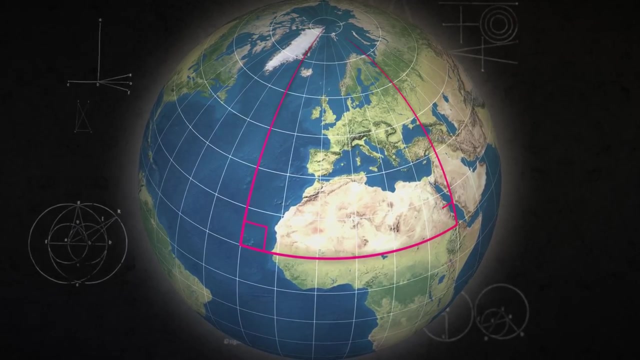 What is the shape of the entire universe? Using the differences between the geometries, we can find that out too. In flat geometry, we expect all the angles of a triangle to add up to 180 degrees without fail. But in spherical geometry, the angles 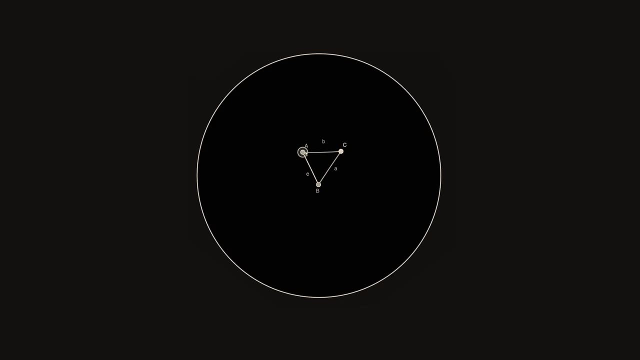 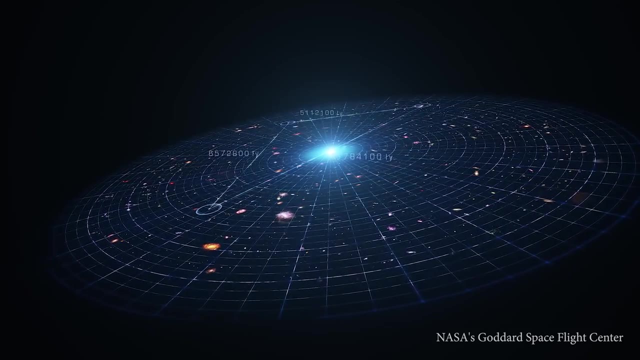 don't add up to 180 degrees, but to more. Similarly, in hyperbolic geometry the angles add up to less than 180 degrees. So to determine the shape of the universe you just need to measure the angles of a triangle. 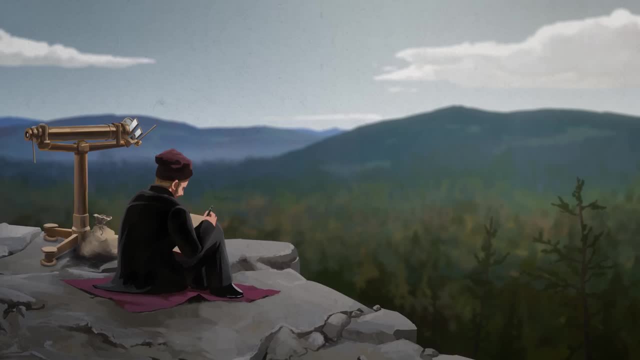 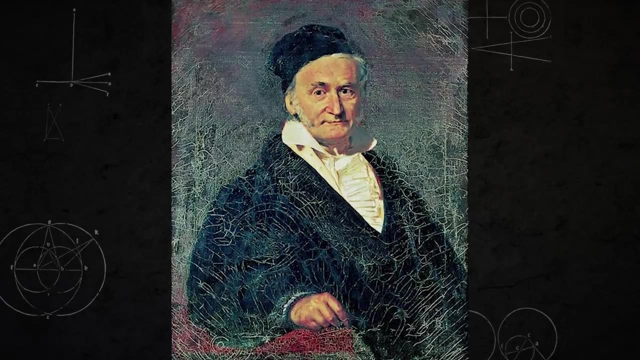 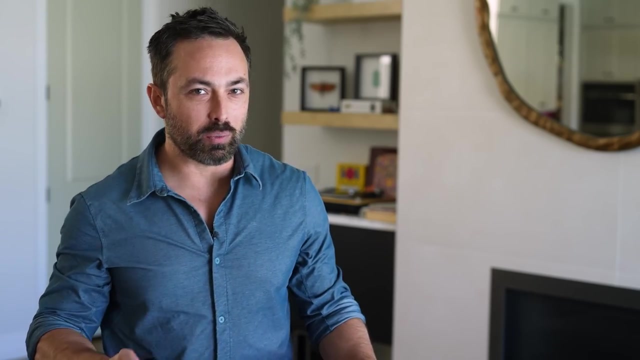 And measuring a triangle is precisely what Gauss was doing 200 years ago. In fact, this led some to speculate that he was actually trying to measure the curvature of space itself. The angle he found 180 degrees within observational error, But that shouldn't be very surprising. 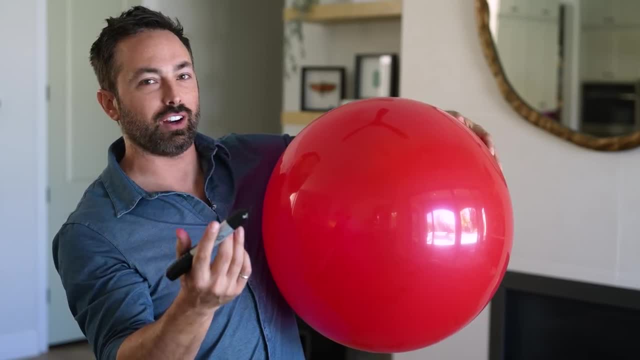 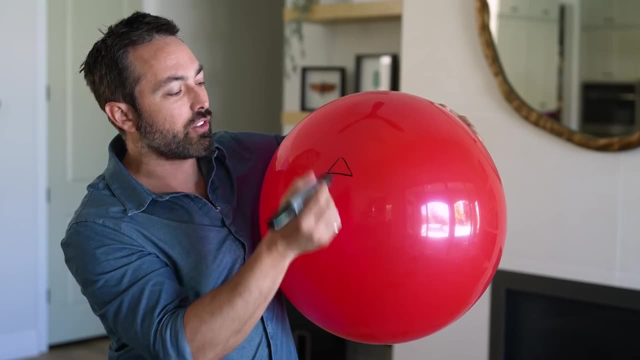 Take this balloon, for example, which approximates a sphere. If I draw a small triangle on it, well, the surface I'm drawing on is basically flat, So the angles inside the triangle will add up to essentially 180 degrees Only if I make the triangle. 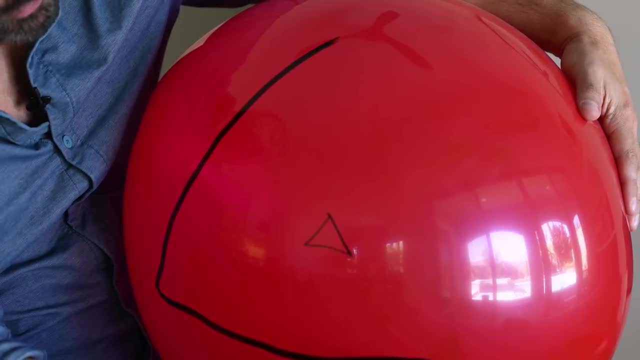 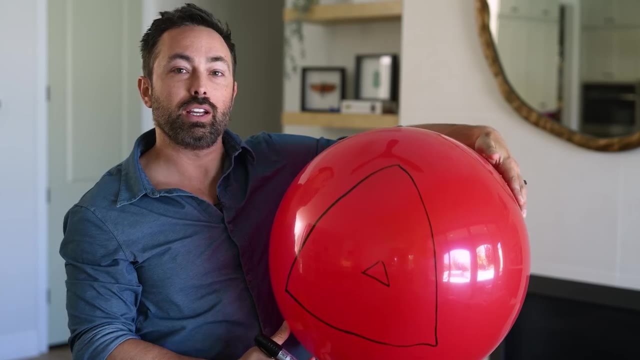 large enough, will the effects of curvature come into play, And then the angles in the triangle will add up to more than 180 degrees. And this was the problem with Gauss' experiment, Even if he was trying to measure the curvature of space itself. 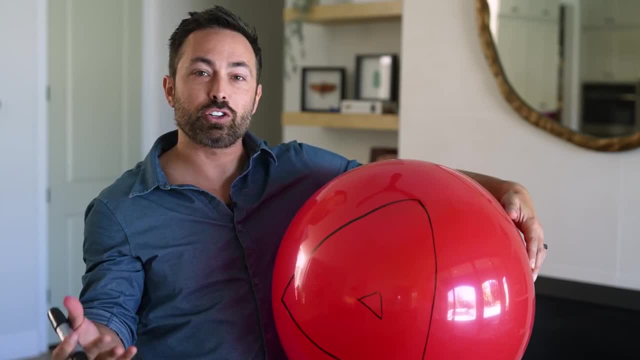 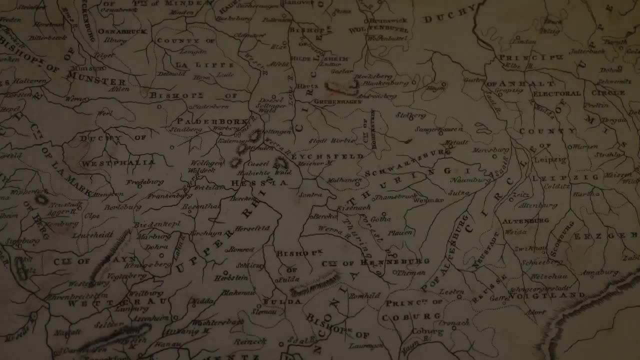 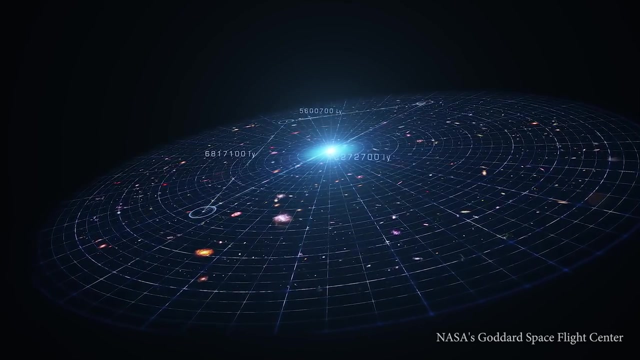 for which there is no solid evidence. the triangle he measured would have been far too small relative to the size of the universe. So in order to overcome the scale issue that Gauss encountered, we need to scale the triangles formed between mountains up to the largest triangles. 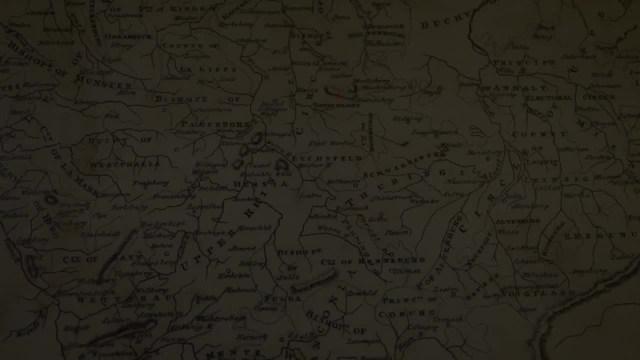 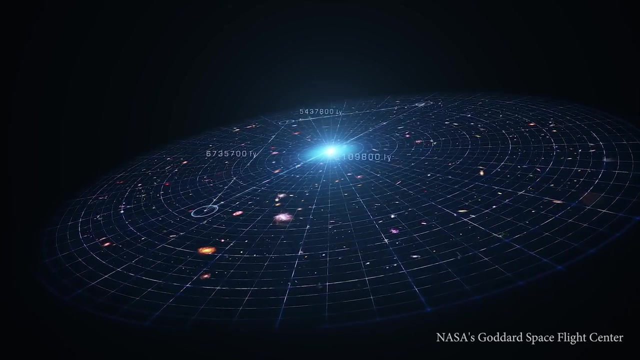 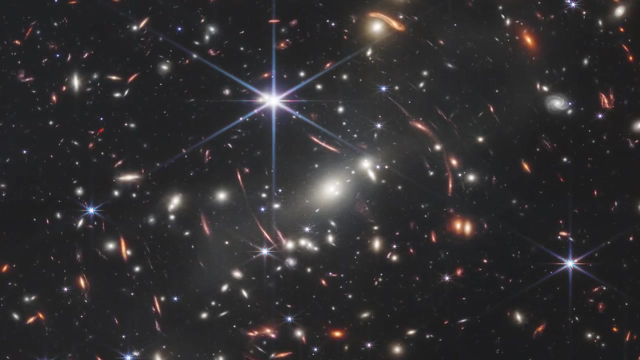 the universe. So, in order to overcome the scale issue that Gauss encountered, we need to scale the triangles formed between mountains up to the largest triangles we can. And since looking further and further away is the same as looking further back in time, we need to look back as far as possible to the very first light we can see, the Cosmic. 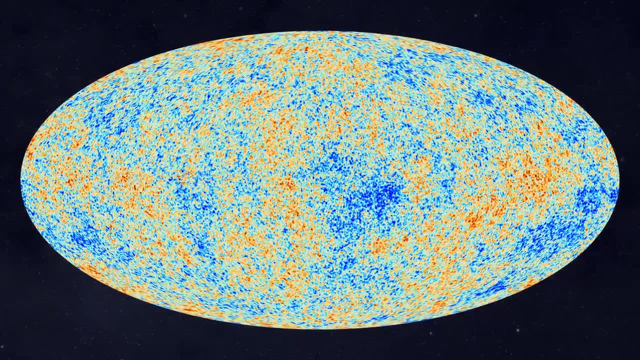 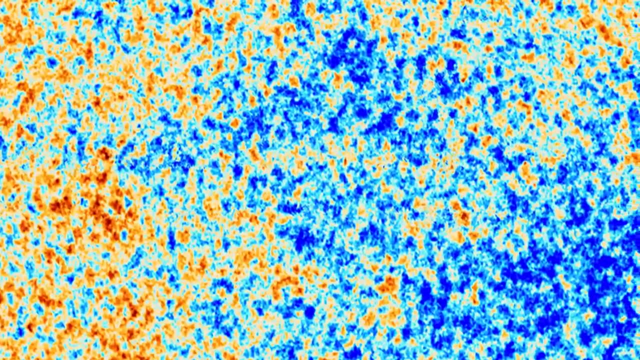 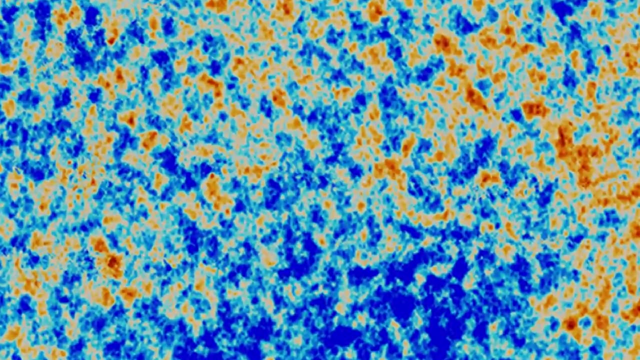 Microwave Background, or CMB, a picture from when the universe was just 380,000 years old. While the CMB is almost completely uniform, there are some spots that are slightly hotter or colder. Now we know how far away the CMB is, so if we can figure out how large such a spot is, 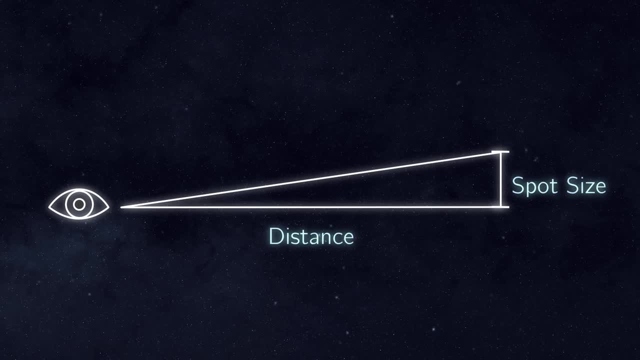 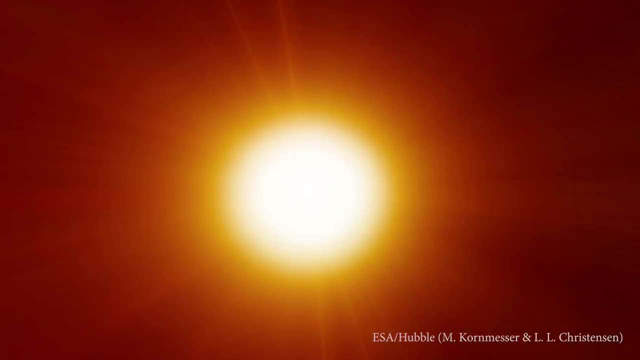 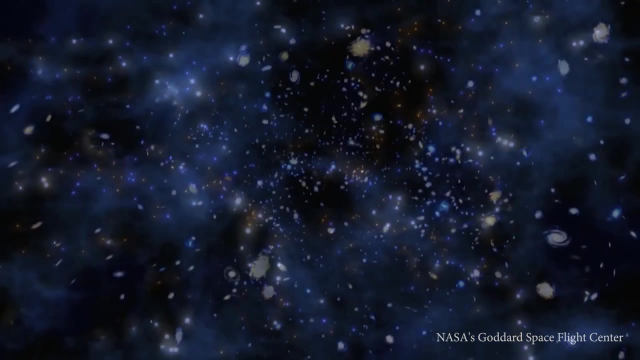 then we can draw a cosmic triangle. It's thought that the first density and temperature variations originated from quantum fluctuations in the very early universe, which were then blown up as the universe expanded. But due to this rapid expansion not all regions were in causal contact with each other. 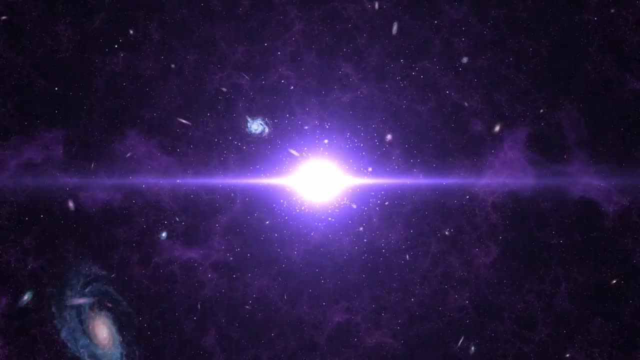 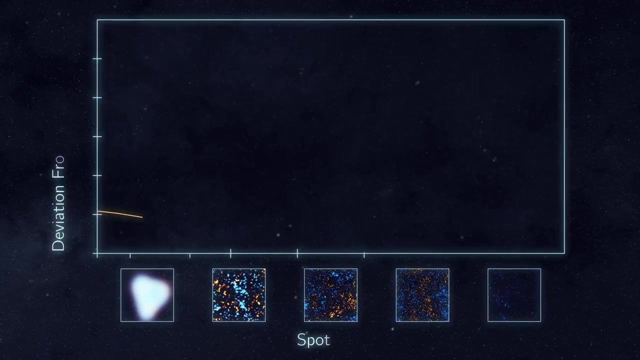 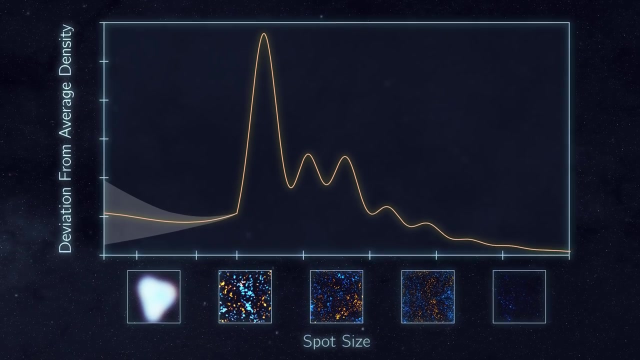 So, using the information we have of how the early universe evolved, astronomers can predict how often spots of different sizes should appear in the CMB. This is what this power spectrum shows, essentially a histogram of how often each spot size should occur if the universe is flat. 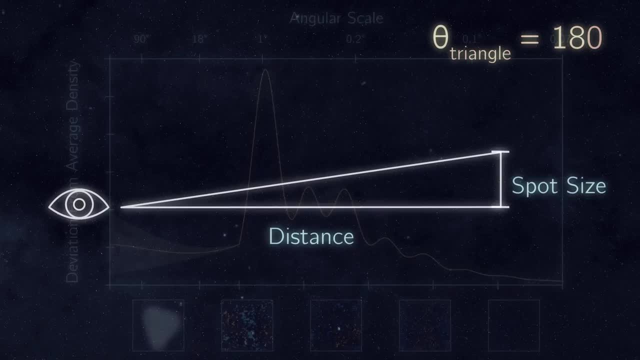 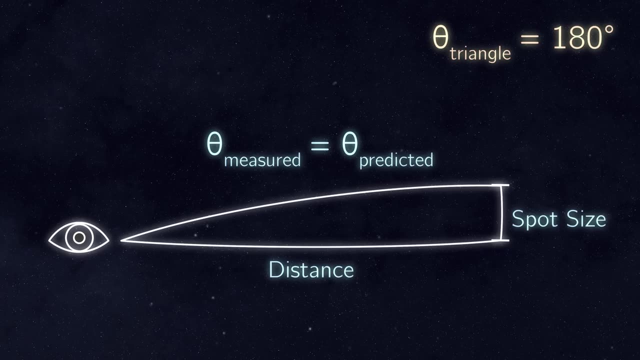 So now we have something to compare our measurement to. If the universe is flat, the angle we measure on the sky should be the same as we'd expect, But if the universe is curved like a sphere, the angles of the triangle should add up to. 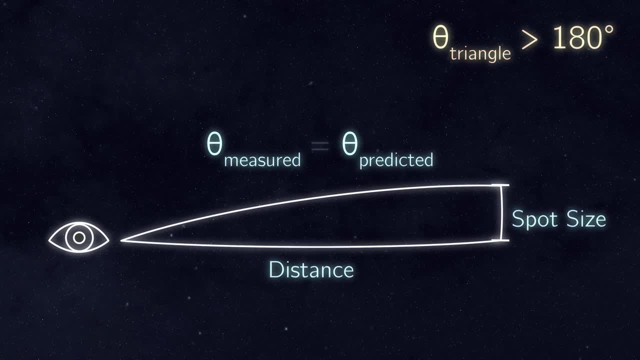 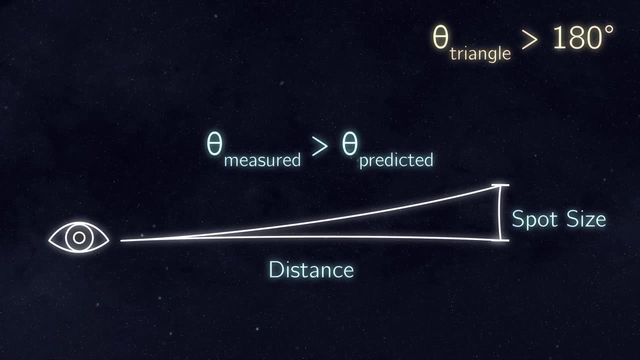 more than 180 degrees. That's a lot. So the angle we'd measure would be larger than predicted and this peak would shift to the left. Similarly, if the universe has hyperbolic geometry, then spots should appear smaller than predicted and this peak would shift to the right. 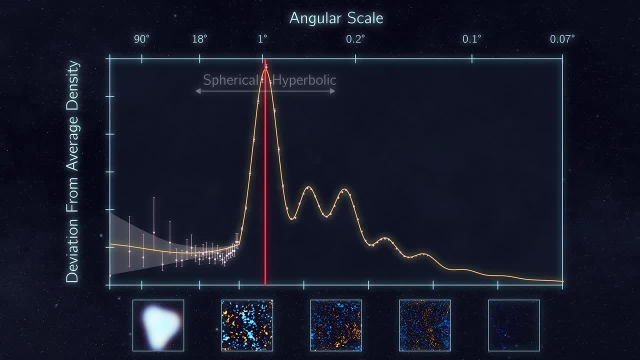 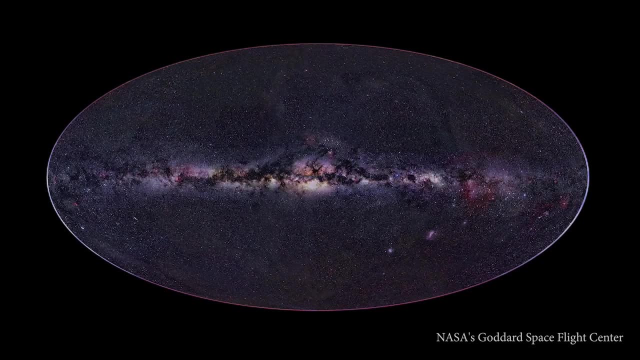 So what did we measure? This is the data from the Planck mission, which is almost exactly what you'd expect if the universe were flat. This mission also gives us the current best estimate for the curvature of the universe, which is 0.0007 ± 1.. 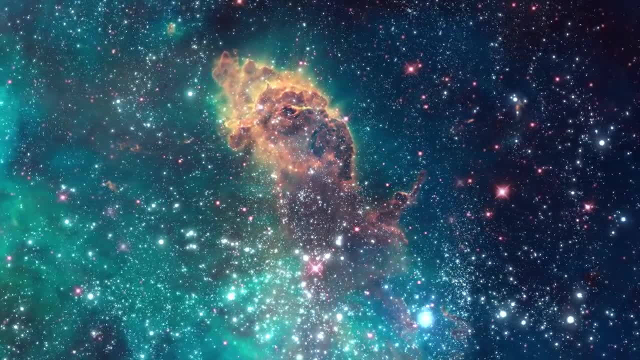 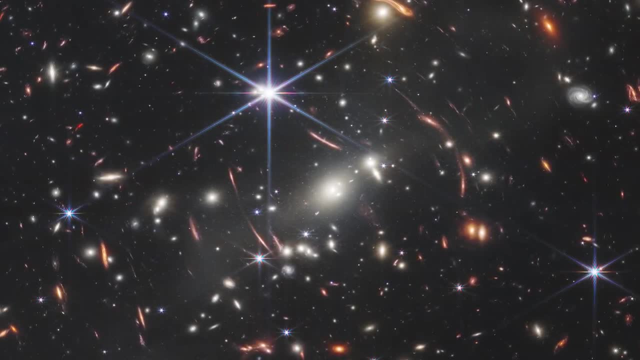 we can, And since looking further and further away is the same as looking further back in time, we need to look back as far as possible to the very first light. we can see the Cosmic Microwave Background, or CMB, a picture from when the universe 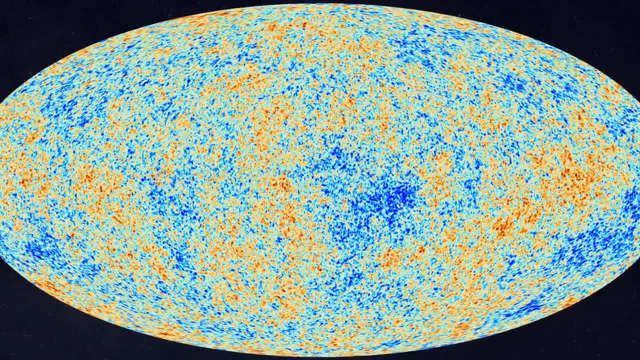 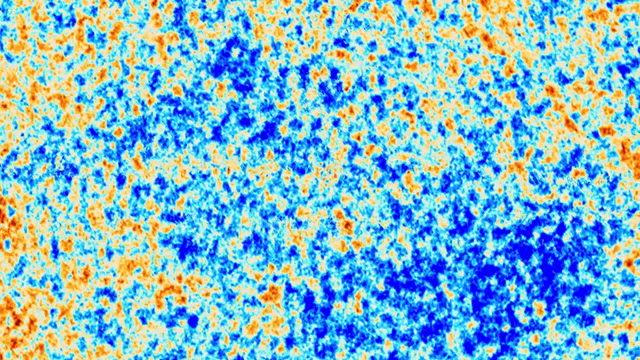 was just 380,000 years old. While the CMB is almost completely uniform, there are some spots that are slightly hotter or colder. Now we know how far away the CMB is, so if we can figure out how large such a spot, 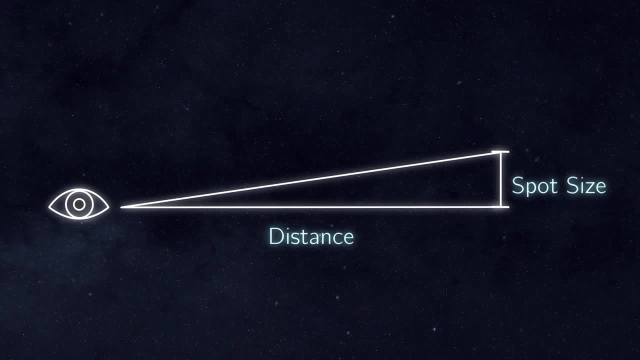 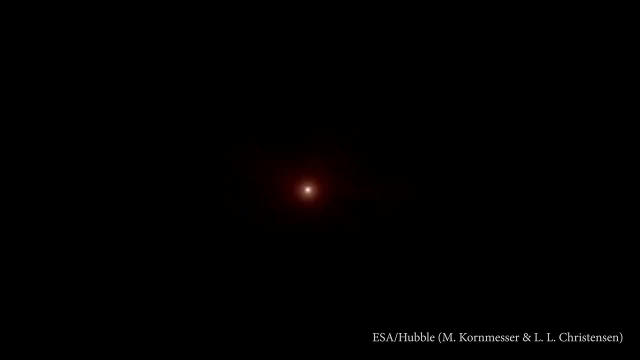 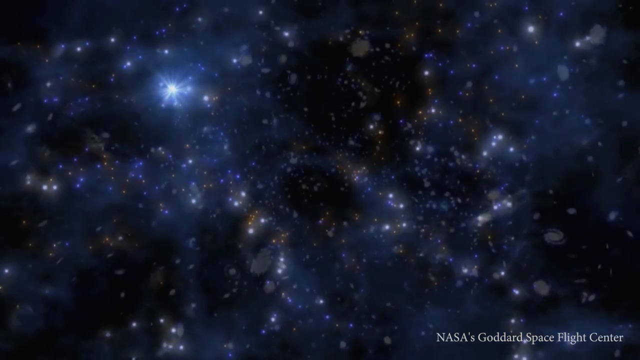 is, then we can draw a cosmic triangle. It's thought that the first density and temperature variations originated from quantum fluctuations in the very early universe, which were then blown up as the universe expanded. But due to this rapid expansion, not all regions were in causal 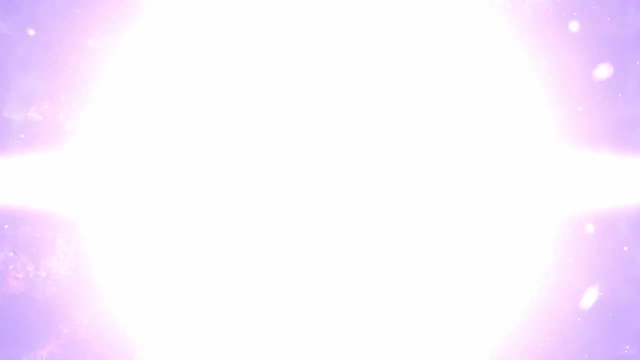 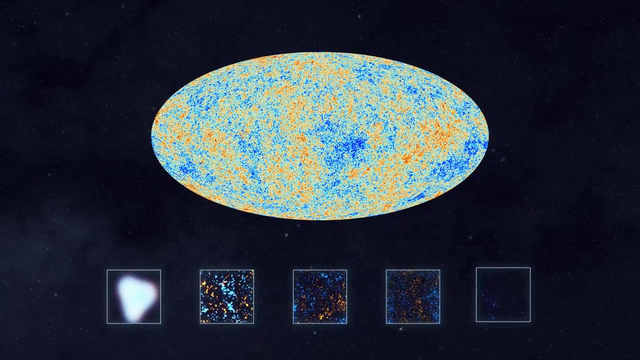 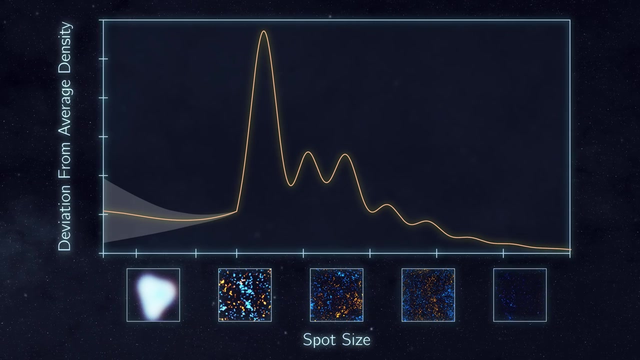 contact with each other. So, using the information we have of how the early universe evolved, astronomers can predict how often spots of different sizes should appear in the CMB. This is what this power spectrum shows, essentially a histogram of how often each spot. 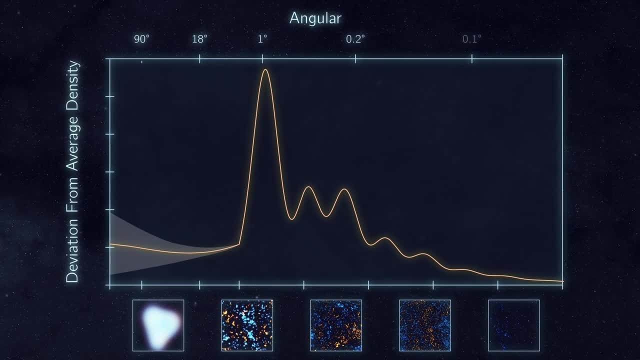 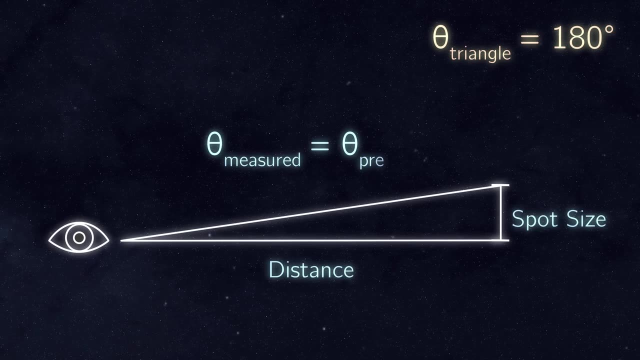 size should occur if the universe is flat. So now we have something to compare our measurement to. If the universe is flat, the angle we measure on the sky should be the same as we'd expect. But if the universe is curved like a sphere, 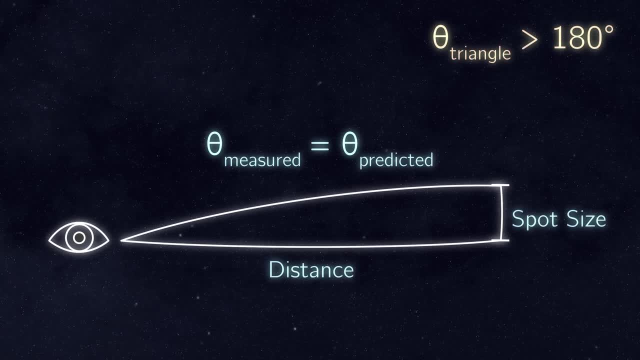 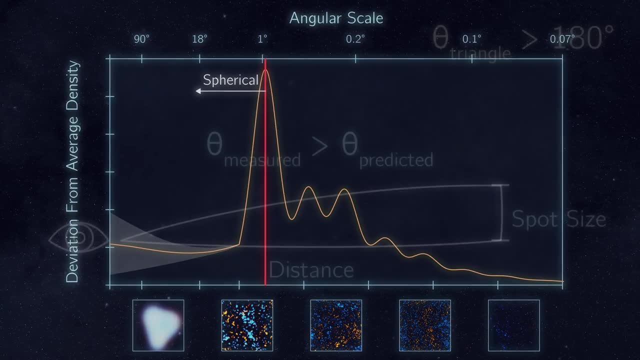 the angles of the triangle should add up to more than 180 degrees, so the angle we'd measure would be larger than predicted, And this peak would shift to the left. Similarly, if the universe has hyperbolic geometry, then spots should appear smaller than predicted. 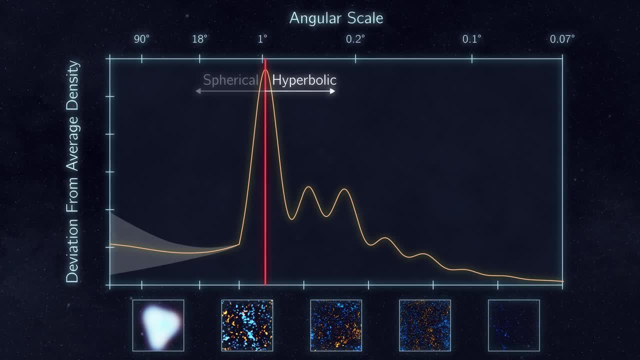 and this peak would shift to the right. So what did we measure? This is the data from the Planck mission, which is almost exactly what you'd expect if the universe were flat. This mission also gives us the current best estimate for the curvature. 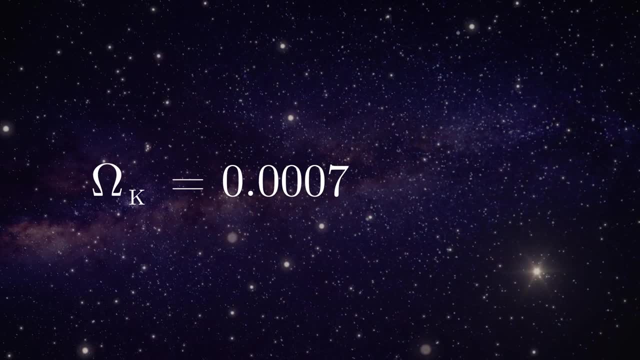 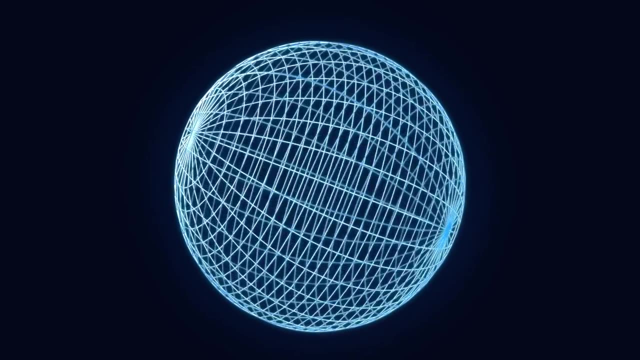 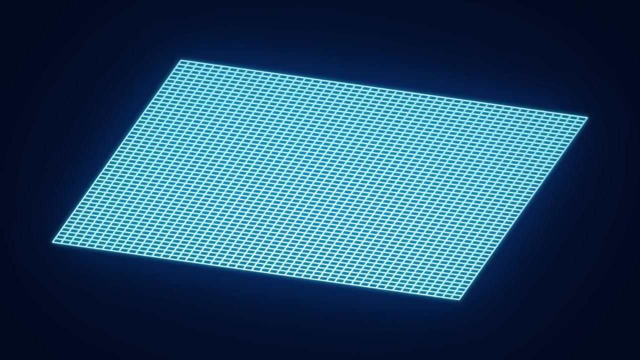 of the universe, which is .0007 plus minus .0019.. So that's basically zero within the margin of error. So we're fairly certain that the universe we live in is flat. But living in a flat universe seems to be remarkably serendipitous. 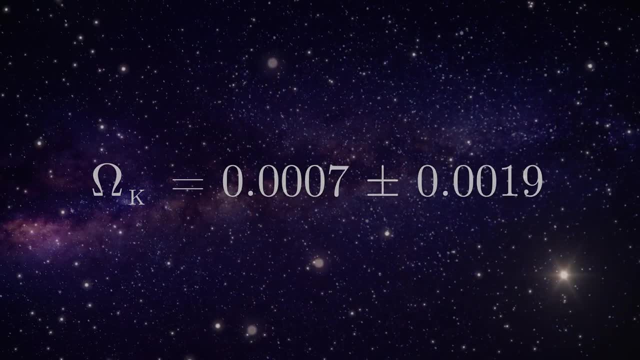 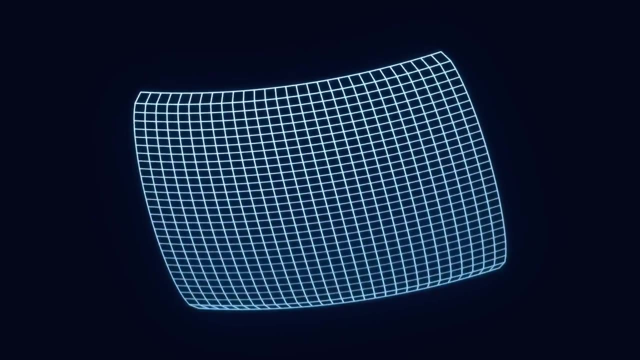 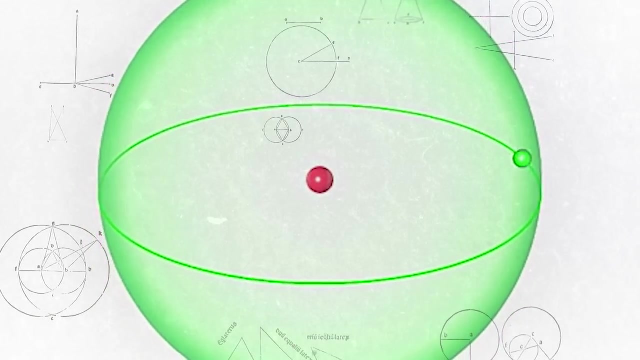 So that's basically zero within the margin of error. So we're fairly certain that the universe we live in is flat. But living in a flat universe seems to be remarkably serendipitous. Right now, the average mass-energy density comes down to the equivalent of about 6 hydrogen. 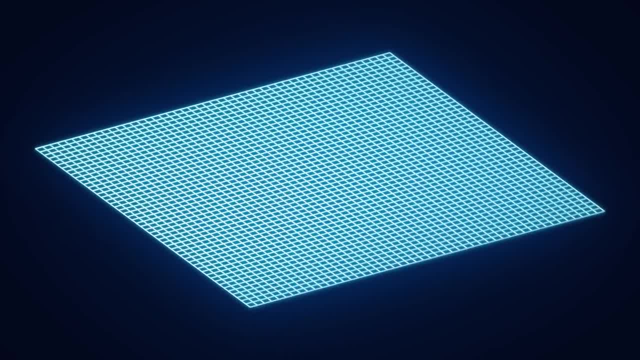 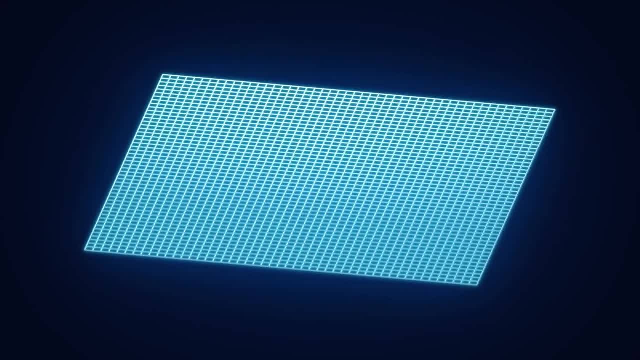 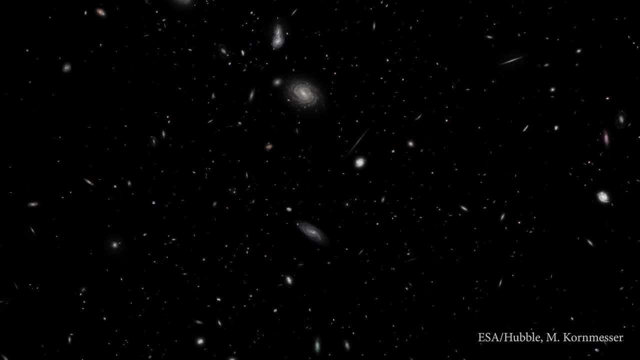 atoms per cubic meter. If on average that was just one more hydrogen atom, the universe would have been more spherically curved. If it were just one less, the curvature would be hyperbolic geometry. And so far we're not entirely sure why the universe has the mass-energy density it has. 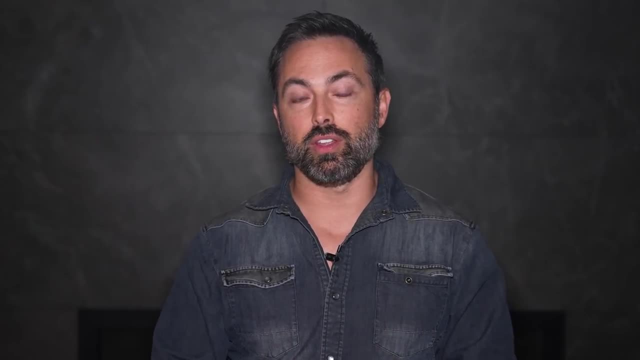 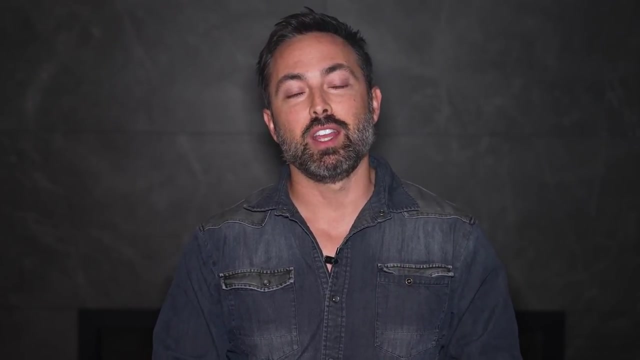 What we do know is that general relativity is one of our best physical theories of reality, And at the very heart of it are those paradoxical and seemingly absurd geometries, ones we found because mathematicians spent over 2,000 years thinking about a single sentence from the 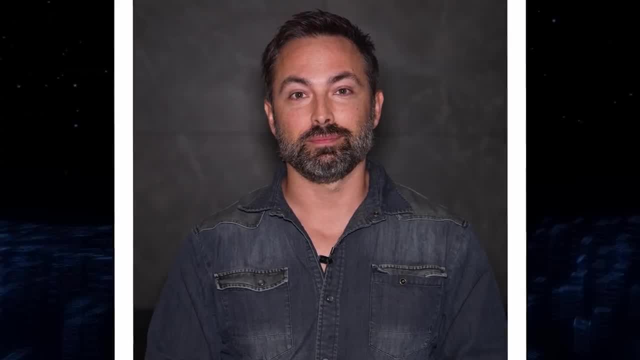 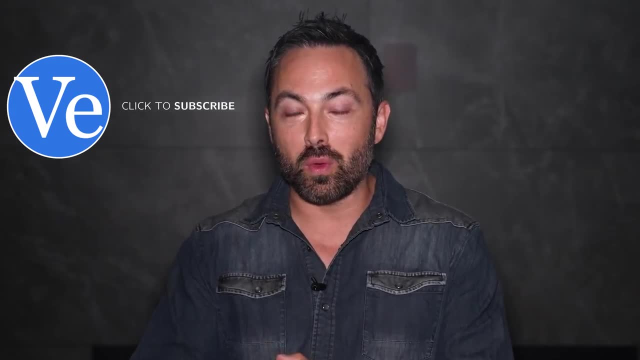 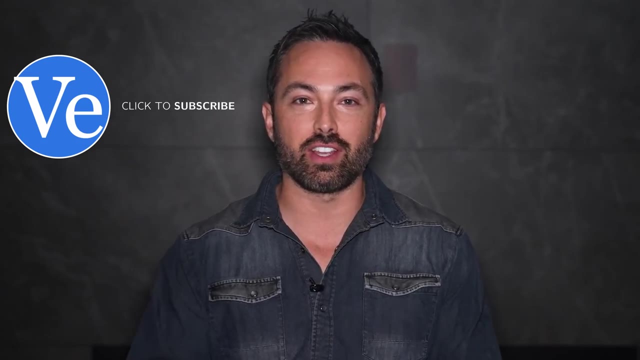 world's most famous math text, So let's take a look at some of them. When it comes to human brilliance, it's not just what you know, it's also how you think, And a great way to improve how you think is by building your knowledge and problem-solving. 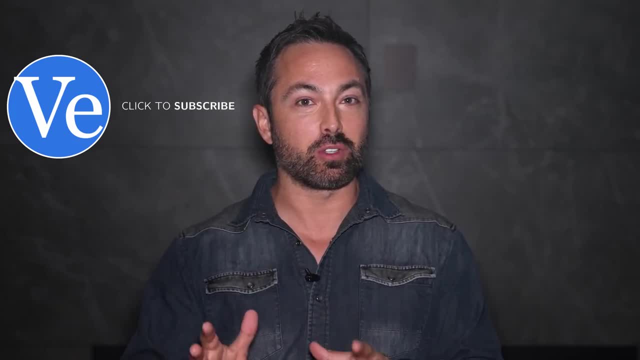 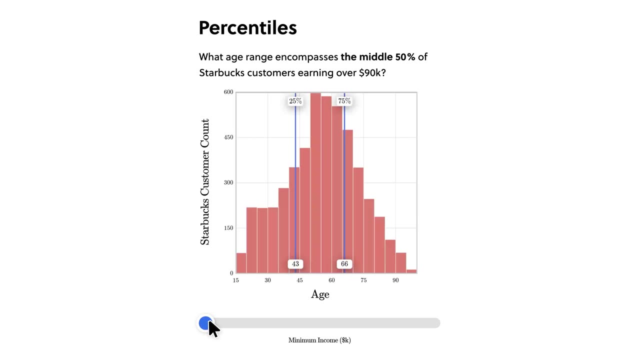 skills. So if you're looking for a free and easy way to do just that, then check out this video's sponsor, Brilliantorg. With Brilliant, you can master key concepts in everything from math and data science to programming and technology. All you have to do is click on the link in the description. 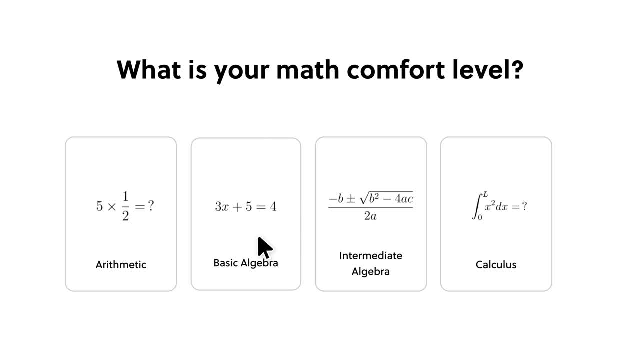 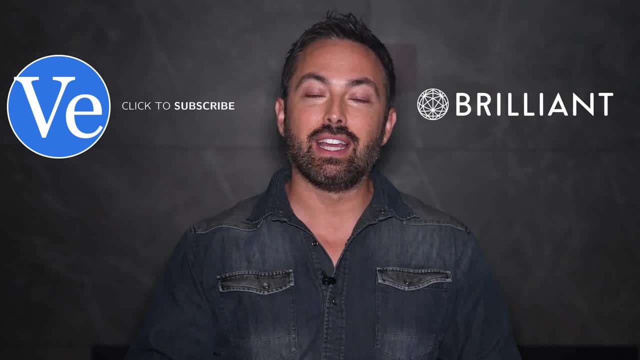 What you have to do is set your goal and Brilliant will design the perfect learning path for you, giving you all the tools you need to reach it. Want to follow in the footsteps of Euclid and Bolyai? Then Brilliant's latest course, Measurement, is the perfect addition to your problem-solving. 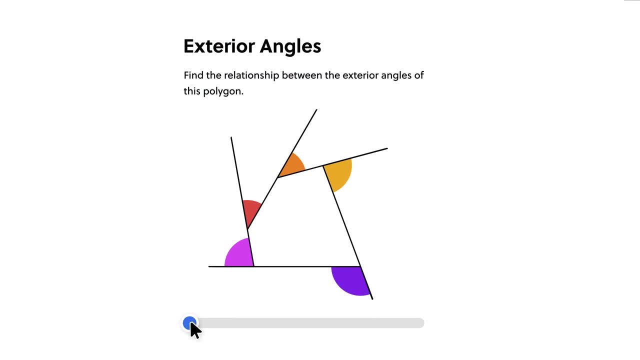 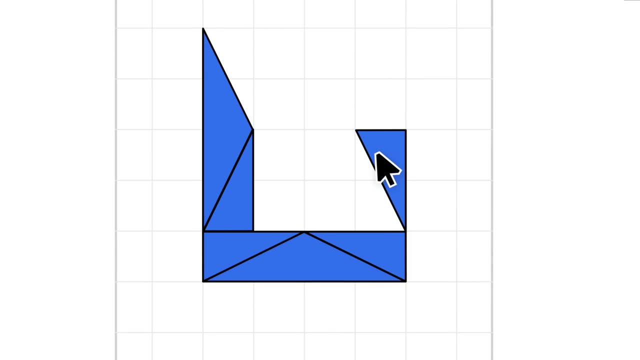 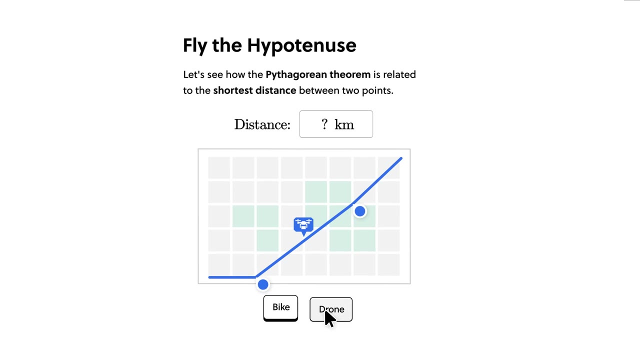 toolkit. The course takes you on a tour through the essentials of geometry, getting you hands-on with concepts to help sharpen your spatial reasoning skills. A solid foundation in geometry can be a launchpad to hundreds of other problems. There are hundreds of applications, everything from computer graphics and data clustering. 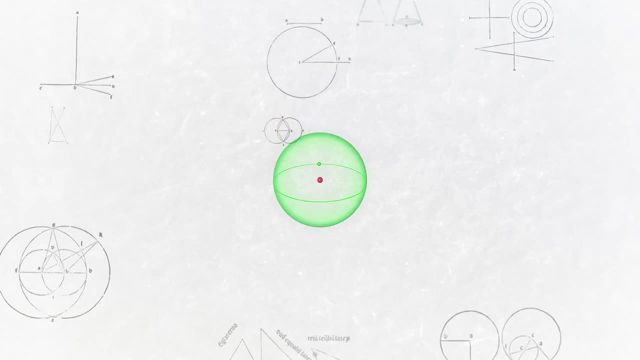 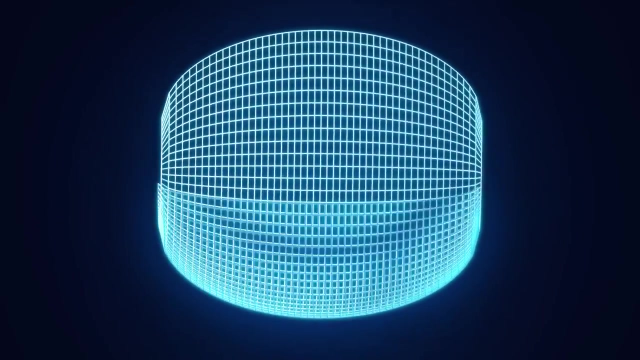 Right now, the average mass energy density comes down to the equivalent of about six hydrogen atoms per cubic meter. If, on average, that was just one more hydrogen atom, the universe would have been more spherically curved. If there were just one less. 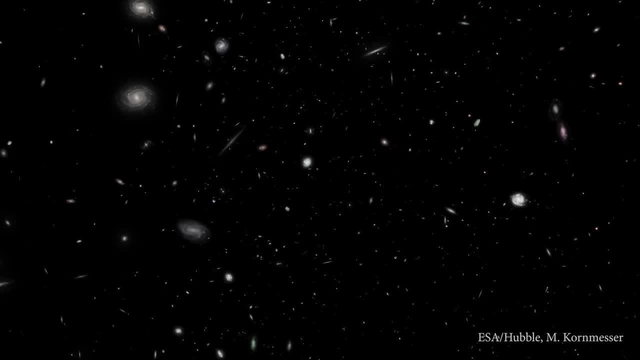 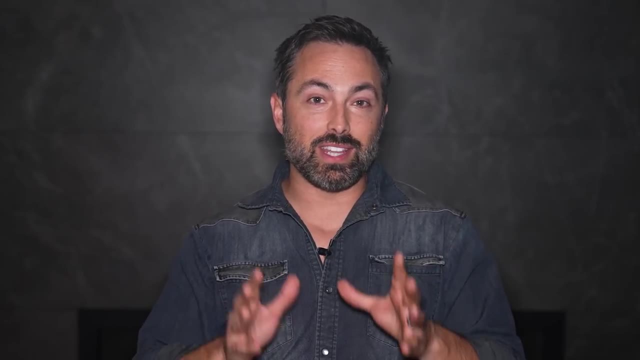 the curvature would be hyperbolic geometry, And so far we're not entirely sure why the universe has the mass energy density it has. What we do know is that general relativity is one of our best physical theories of reality, And at the very heart of it. 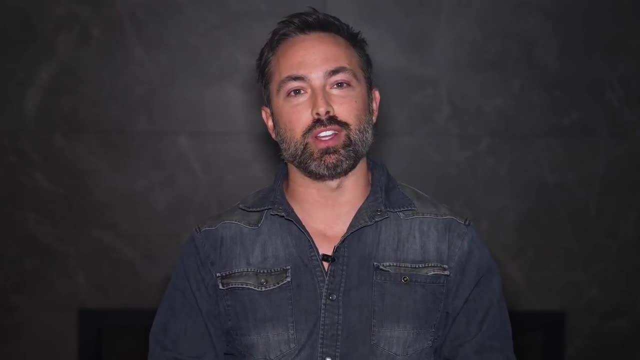 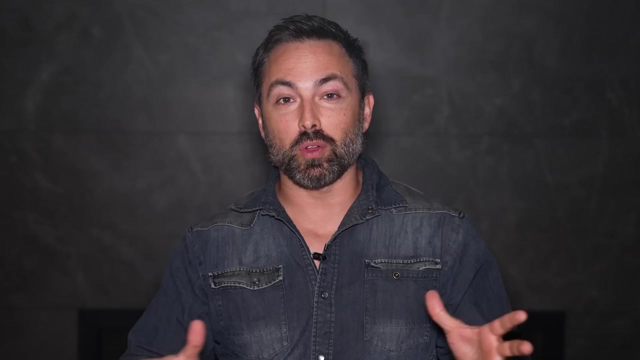 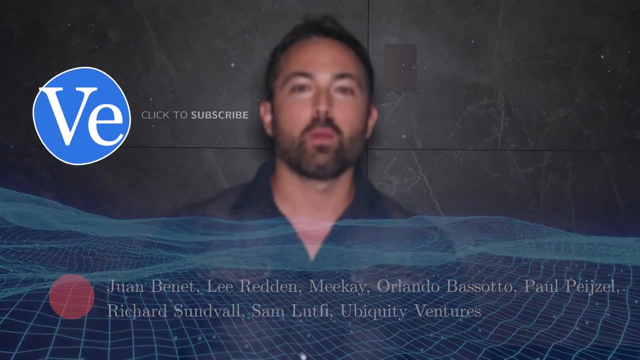 are those paradoxical and seemingly absurd geometries, Ones we found because mathematicians spent over 2,000 years thinking about a single sentence from the world's most famous math text. When it comes to human brilliance, it's not just what you know, it's also how. 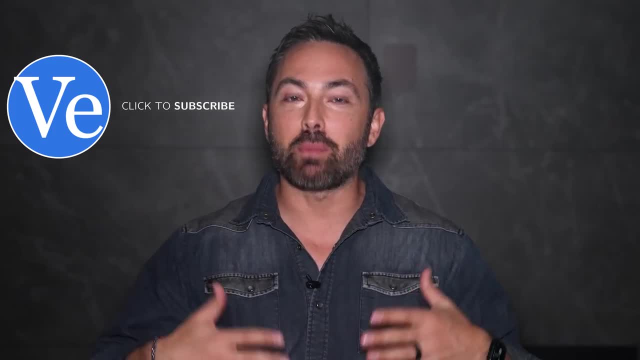 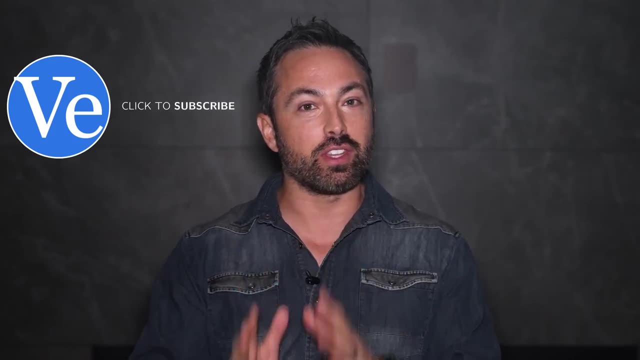 you think, And a great way to improve how you think is by building your knowledge and problem-solving skills. So if you're looking for a free and easy way to do just that, then check out this video's sponsor, Brilliantorg. With Brilliant, you can master key concepts. 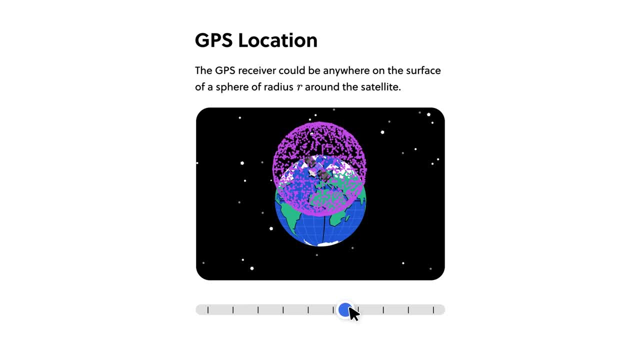 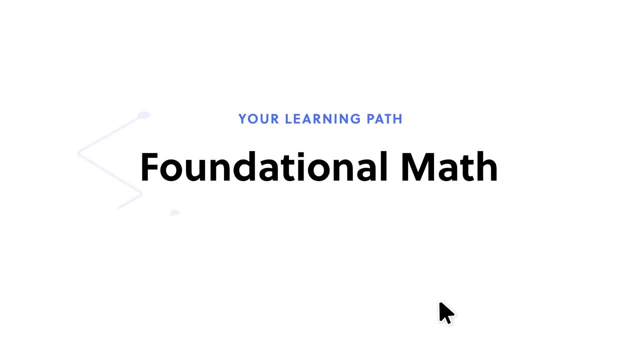 in everything from math and data science to programming and technology. All you have to do is set your goal and Brilliant will design the perfect learning path for you, giving you all the tools you need to reach it. Want to follow in the footsteps of Euclid? 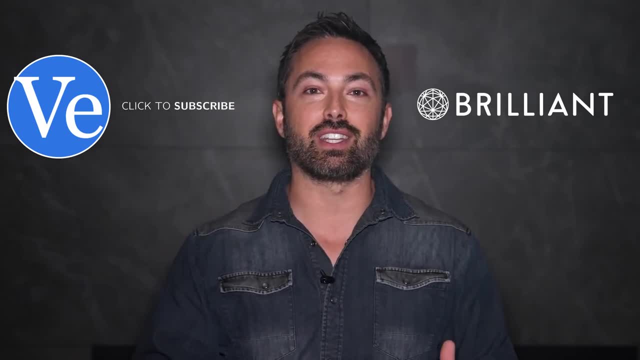 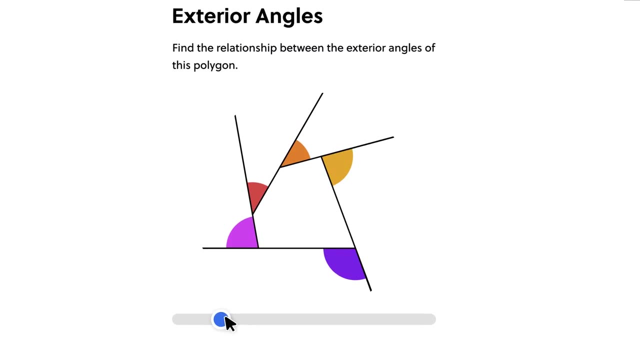 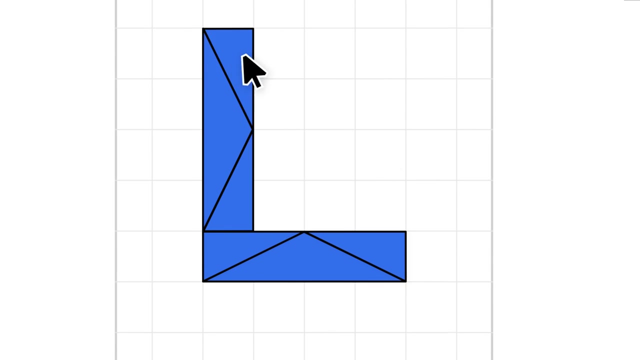 and Boleyi. Then Brilliant's latest course, Measurement, is the perfect addition to your problem-solving toolkit. The course takes you on a tour through the essentials of geometry, getting you hands-on with concepts to help sharpen your spatial reasoning skills. A solid foundation in geometry. 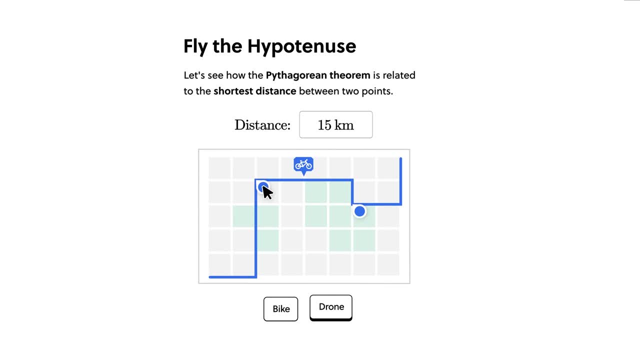 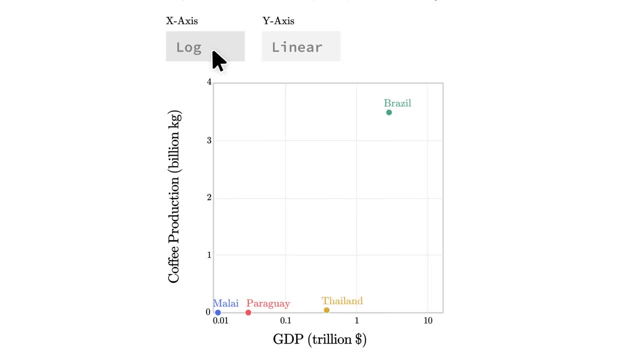 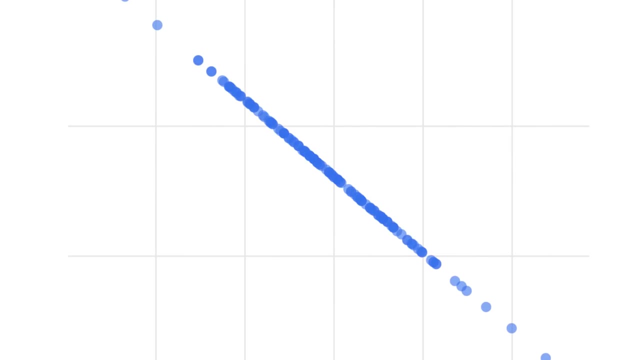 can be a launchpad to hundreds of applications, everything from computer graphics and data clustering in AI algorithms to understanding Einstein's theory of general relativity. Beyond Measurement, Brilliant has a huge library of things to learn, But what I love most about Brilliant is that they connect what you learn. 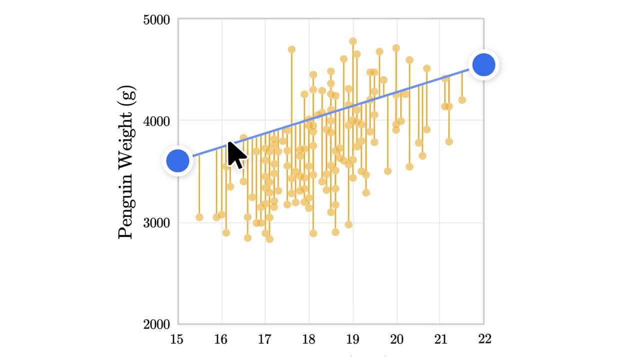 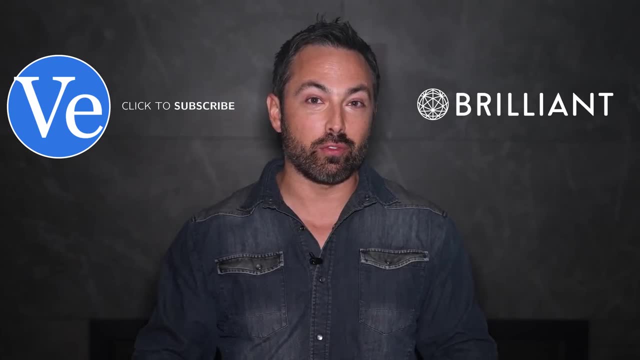 to real-world examples And because each lesson is hands-on, you'll build intuition so you can put what you've learned to good use, To try everything Brilliant has to offer for free for a full 30 days. visit Brilliantorg Or click that link down in the description.